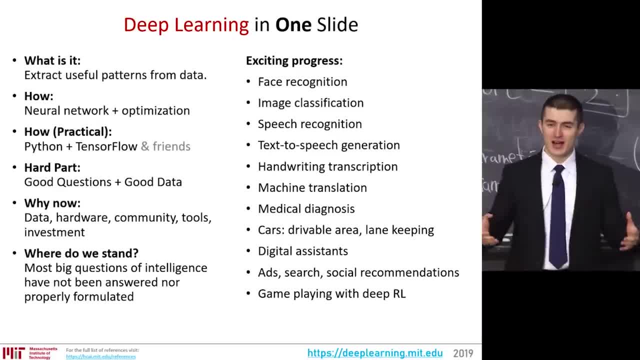 How. the fundamental aspect that we'll talk about a lot is the optimization of neural networks. The practical nature that we'll provide through the code and so on is that there's Libraries that make it accessible and easy to do some of the most powerful things in deep learning using Python, TensorFlow and Friends. 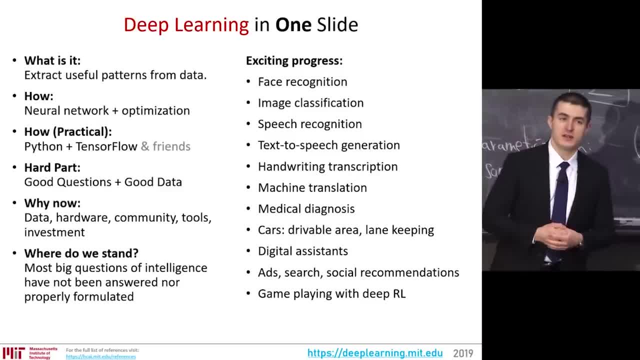 The hard part always with machine learning and artificial intelligence in general, is asking good questions and getting good data. A lot of times, the exciting aspects of what the news covers and a lot of the exciting aspects of what is published in the prestigious conferences in an archive. 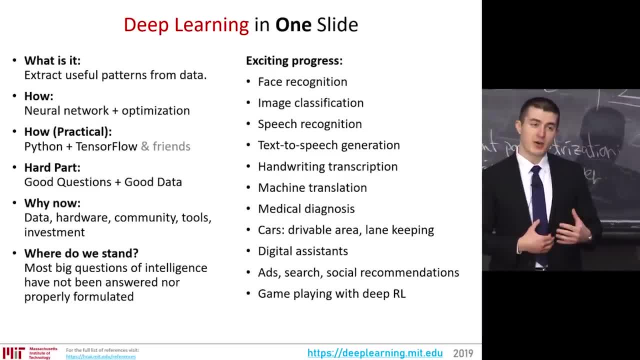 in a blog post is the methodology. The hard part is applying that methodology to solve real-world problems, to solve fascinating, interesting problems, and that requires data. That requires asking the right questions of that data, organizing that data and labeling, selecting aspects of that. 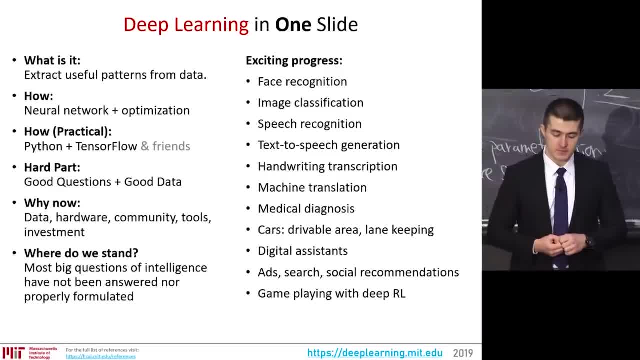 data that can reveal the answers to the questions you ask. So why has this breakthrough over the past decade of the application of neural networks? the ideas of neural networks, what has happened? what has changed? have been around since the 1940s and ideas have been percolating even before. 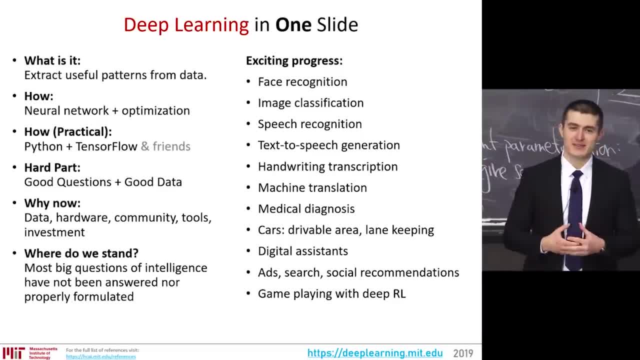 The digitization of information, data, the ability to access data easily in a distributed fashion across the world- all kinds of problems have now a digital form that can be accessed by learning algorithms, Hardware compute- both the Moore's Law of CPU and GPU- and ASICs- Google's TPU. 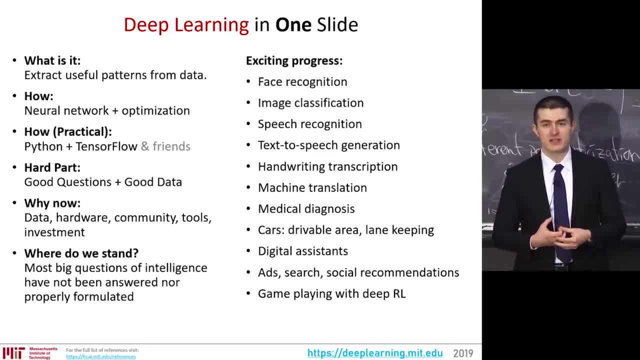 systems, hardware that enables the efficient, effective, large-scale execution of these algorithms, Community people here, people all over the world, Being able to work together, to talk to each other, to feed the fire of excitement behind machine learning, GitHub and beyond The tooling, as we'll talk about TensorFlow, PyTorch and everything. 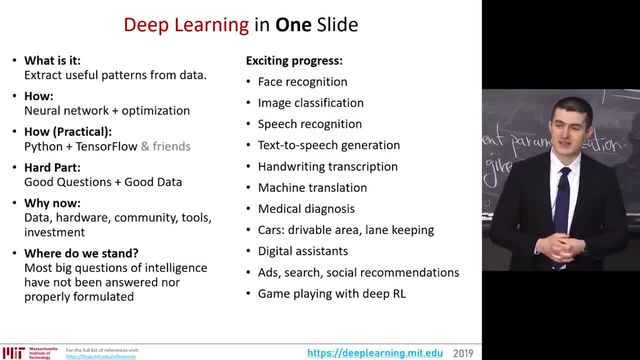 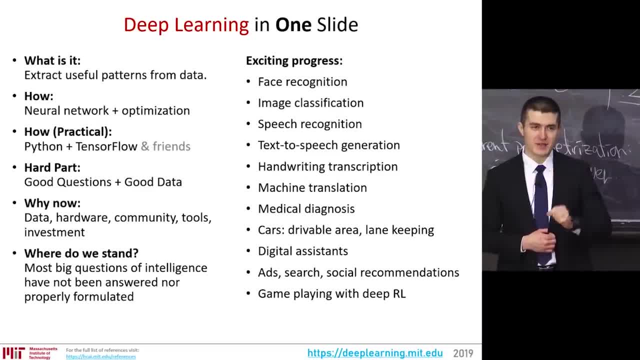 with less and less knowledge, where the idea and the data become the central point, not the effort that takes you from the idea to the solution. And there's been a lot of exciting progress, some of which we'll talk about, from face recognition to the general problem of scene understanding. 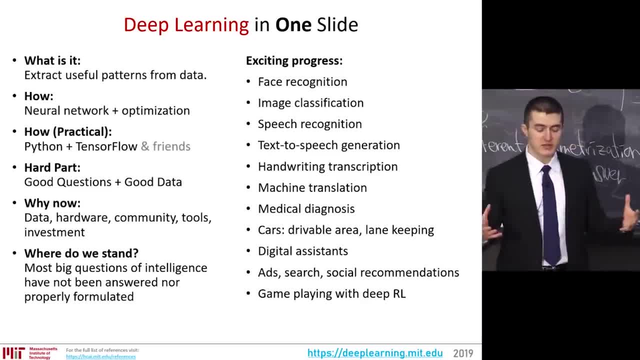 image classification to speech text, natural language processing, transcription, translation in medical applications and medical diagnosis. And cars being able to solve many aspects of perception in autonomous vehicles with drivable area, lane detection, object detection, digital assistance- the ones on your phone and beyond, the ones in your home. Ads recommender systems. 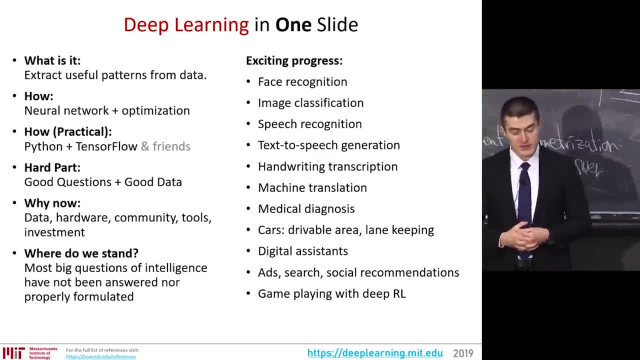 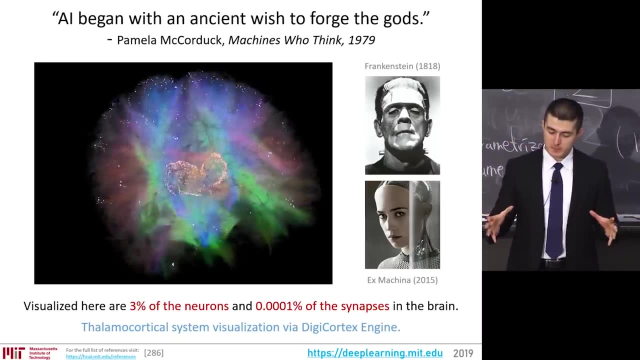 from Netflix to search, to social Facebook And, of course, the deep reinforcement learning successes in the playing of games, from board games to StarCraft and Dota. Let's take a step back. Deep learning is more than a set of tools to solve practical problems. 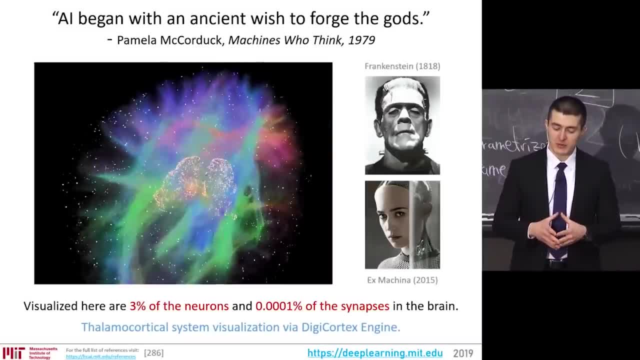 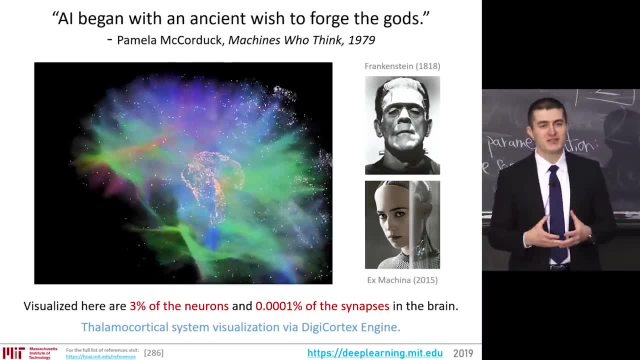 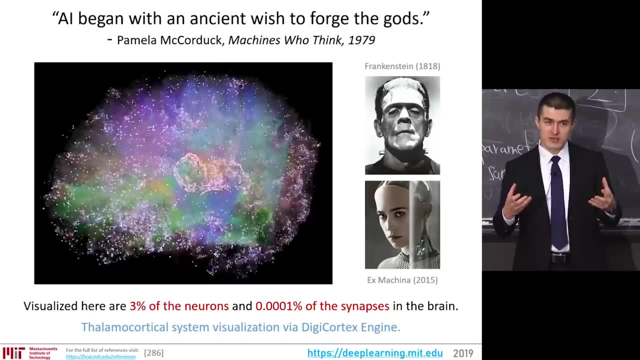 Pamela McCordick said in 79,: AI began with the ancient wish to forge the gods. Throughout our history, throughout our civilization, human civilization, we've dreamed about creating echoes of whatever is in this mind of ours, in the machine, and creating living organisms. 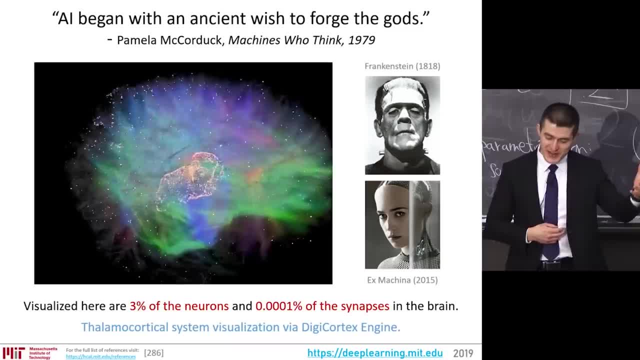 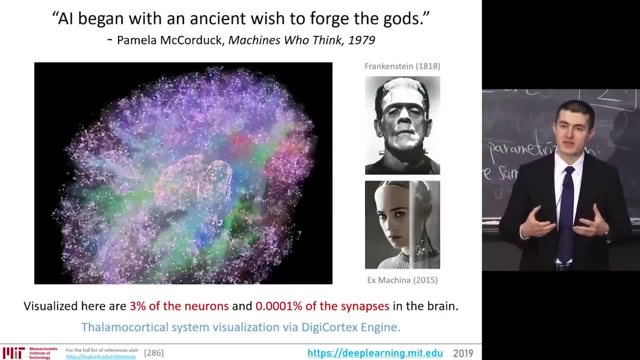 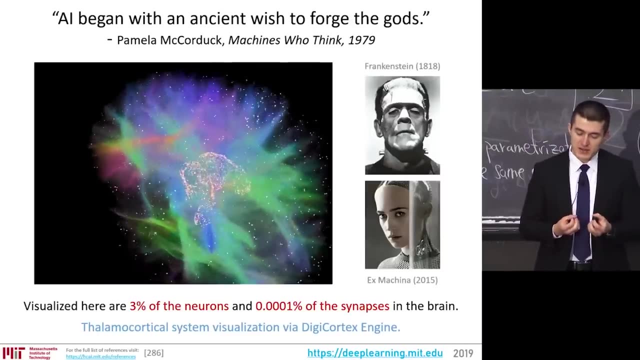 From the popular culture in the 1800s, with Frankenstein to Ex Machina. this vision, this dream of understanding intelligence and creating intelligence has captivated all of us, And deep learning is at the core of that, because there's aspects of it, the learning aspects, that elasticity 응. 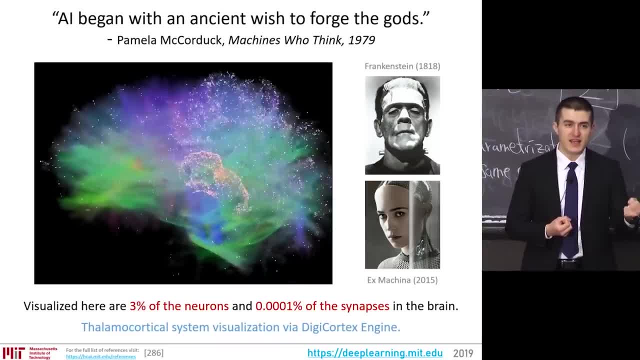 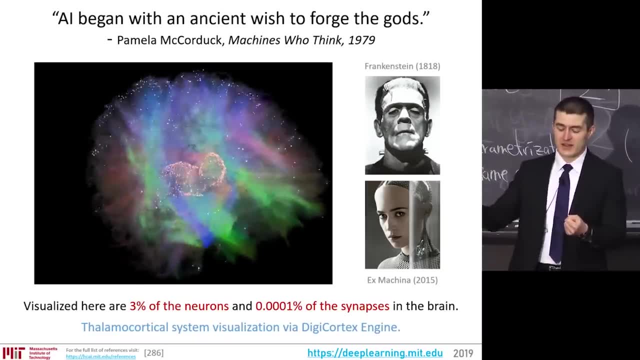 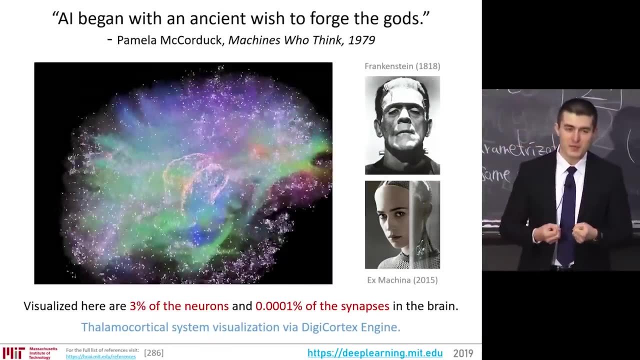 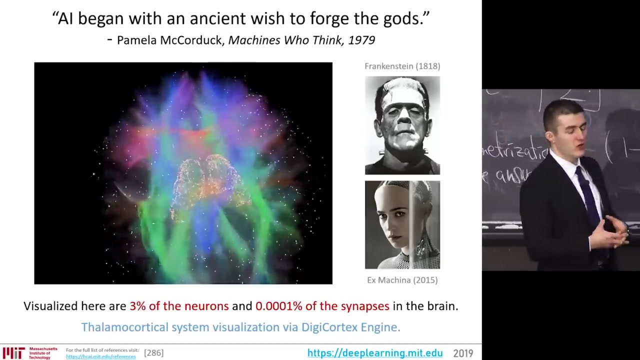 captivate our imagination about what is possible given data and methodology, what learning, learning to learn and beyond, how far they can take us. and here visualize is just 3% of the neurons and 1 millionth of the synapses in our own brain, this incredible structure that's in our mind and there's only echoes of. 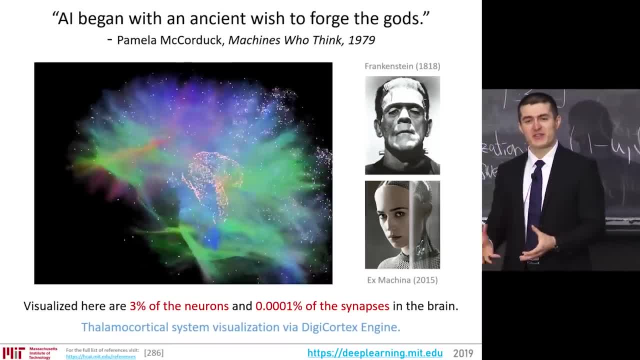 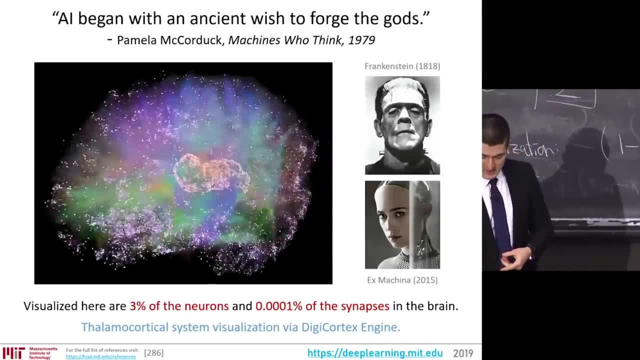 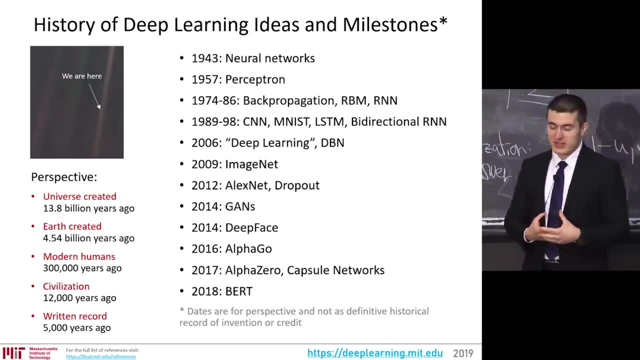 it small shadows of it in our artificial neural networks were able to create, but nevertheless those echoes are inspiring to us. the history of neural networks on this pale blue dot of ours started quite a while ago with summers and winters, with excitements and periods of pessimism, starting in the forties with 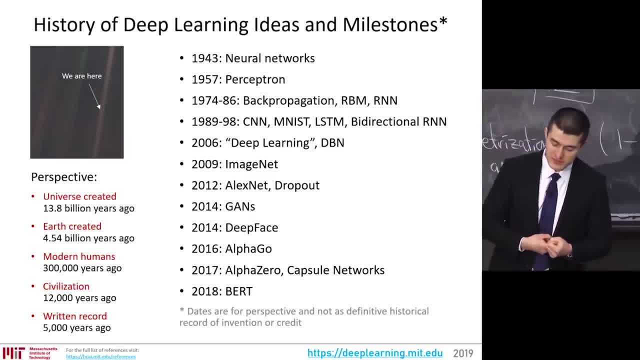 neural networks and the implementation of those neural networks as a perceptron in the 50s, with ideas of back propagation, restricted balls machines or current neural networks in the 70s and 80s, with convolutional neural networks and the MNIST data set, with data sets beginning to percolate in LSTMs- bidirectional RNN- in the 90s and the 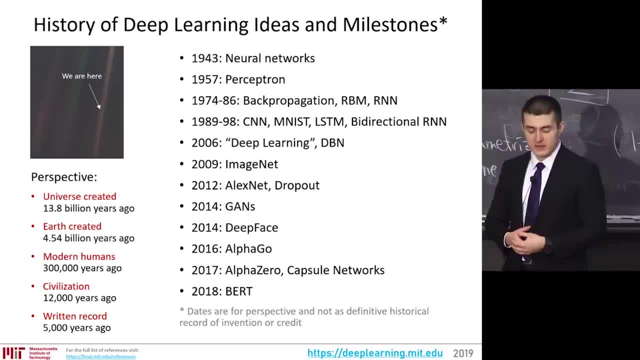 rebranding and the rebirth of neural networks under the flag of deep learning and deep belief. nets in 2006. birth of ImageNet, the data set that on which the possibilities of what deep learning can bring to the world has been first illustrated in the recent years, in 2009,. and AlexNet. 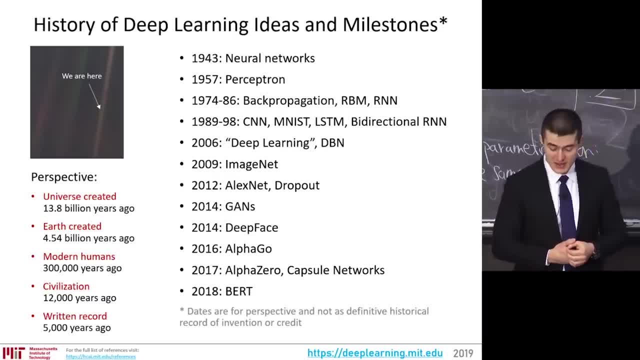 the network that on ImageNet, performed exactly that, with a few ideas like dropout, that improve neural networks over time, every year by year, improving the performance of neural networks In 2014,. the idea of GANs that Yann LeCun called the most exciting idea of the last. 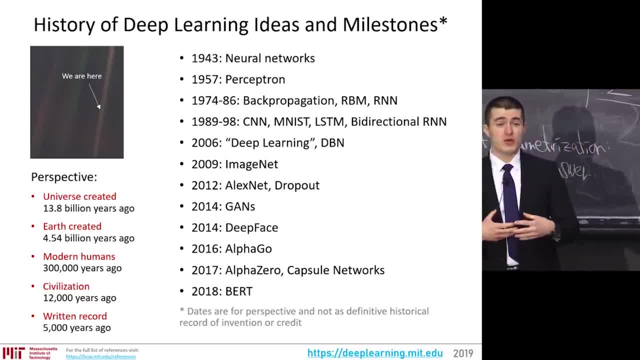 20 years. the generative adversarial networks. the ability to, with very little supervision, generate data, to generate ideas after forming representation of those, From the understanding, from the high level abstractions of what is extracted in the data, be able to generate new samples, create. 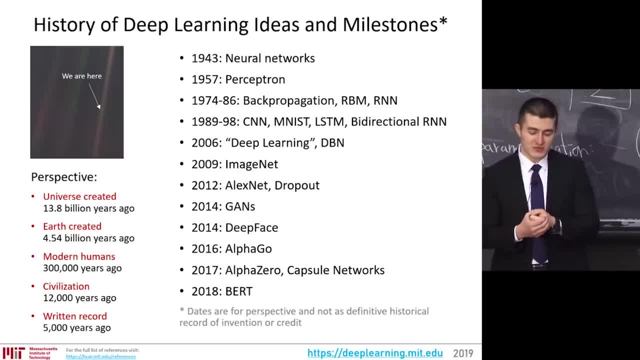 The idea of being able to create- Create as opposed to memorize is really exciting And on the applied side, in 2014, with DeepFace- the ability to do face recognition, There's been a lot of breakthroughs on the computer vision front, that being one of them. 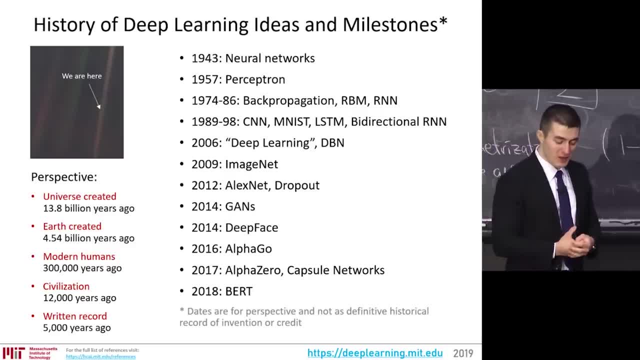 The world was inspired, captivated, in 2016 with AlphaGo and 17 with AlphaZero, beating with less and less and less effort, the best players in the world, The problem that, for most of the history of artificial intelligence, thought to be unsolvable. 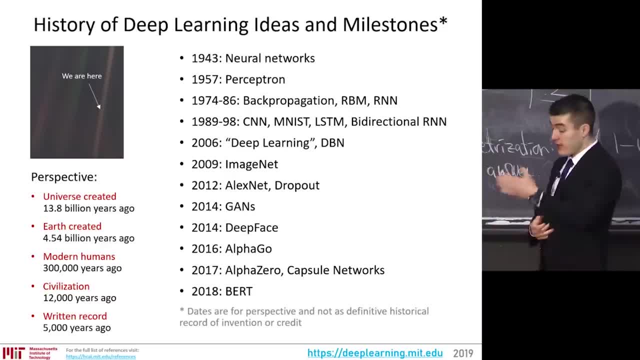 And new ideas with capsule networks, and this year is the year 2018, was the year of natural language processing. A lot of interesting breakthroughs: Google's, BERT and others that we'll talk about. breakthroughs on ability to understand language, understand speech and everything, including language. 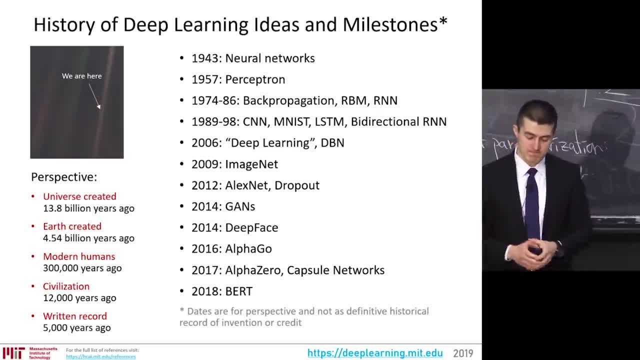 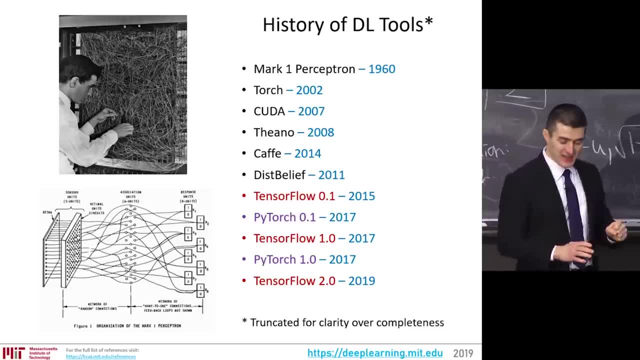 Thank you, And Visual Studio's Cloud and it's part of that and we're going to talk about it. But of course, there's a lot of innovation, including generation, that's built all around that And there's a parallel history of tooling, starting in the 60s with the perceptron and 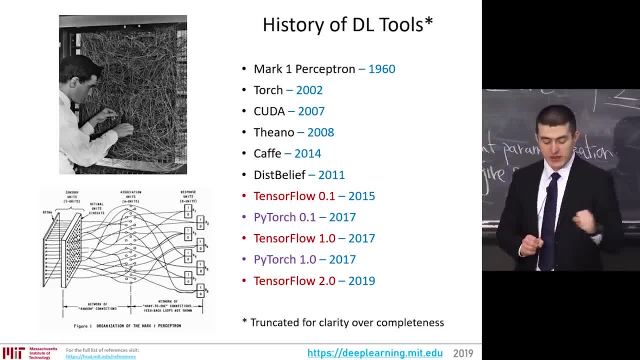 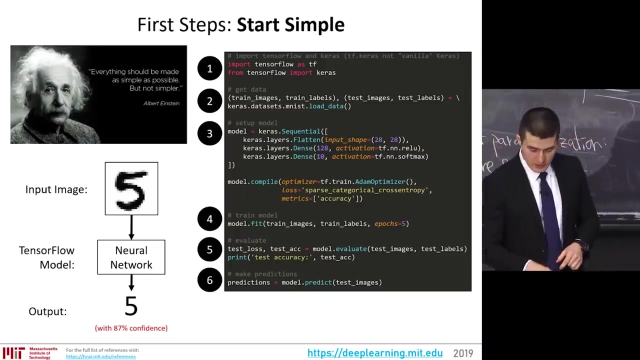 the wiring diagrams there, ending with this year with PyTorch 1.0 and TensorFlow 2.0. These really solidified exciting, powerful ecosystems of tools that enable you to do a lot with very little effort. The sky is the limit, thanks to the tooling. 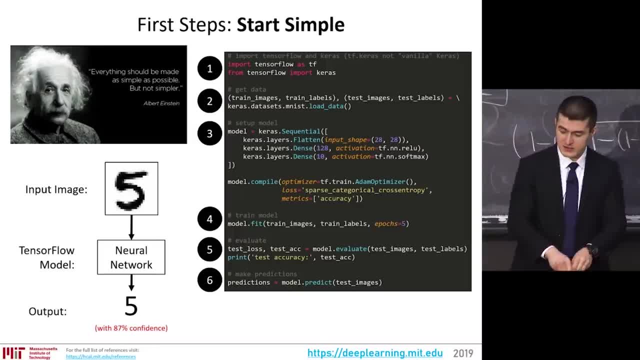 So let's then, from the big picture, take into the smallest. Everything should be made as simple as possible, So let's start simple with a little piece of code before we jump into the details, and a big run-through of everything that is possible in deep learning. 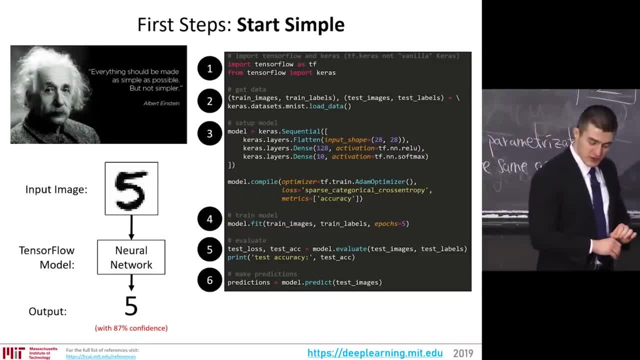 At the very basic level, with just a few lines of code- really six here. six little pieces of code, you can train a neural network to understand what's going on in an image. The classic that I will always love: MNIST data set, the handwriting digits where the 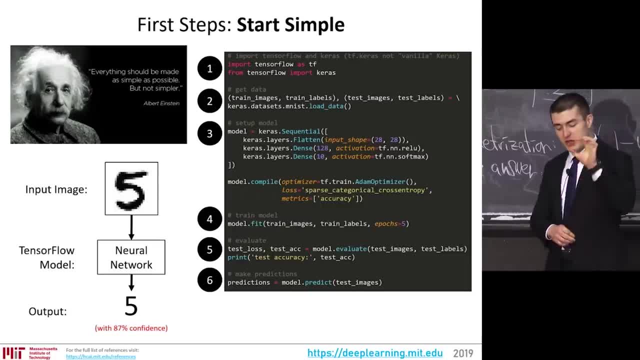 input to a neural network or machine learning system is a picture of a handwriting digit and the output is the number that's in that digit. It's as simple as in. the first step: import the library TensorFlow. Second step: import the data set MNIST. 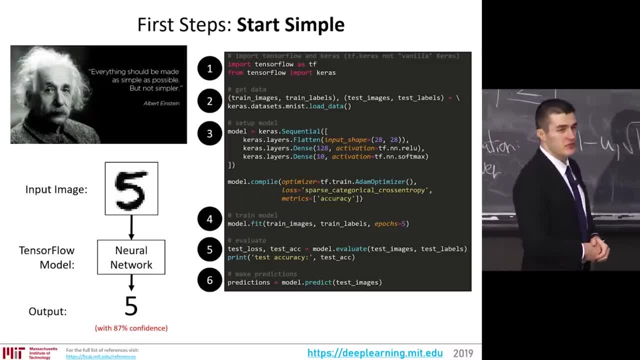 Third step: like Lego bricks, stack on top of each other the neural network, layer by layer, with a hidden layer, an input layer, an output layer. Step four: train the model as simple as a single line model fit. Evaluate the model in step five on the testing data set and that's it. 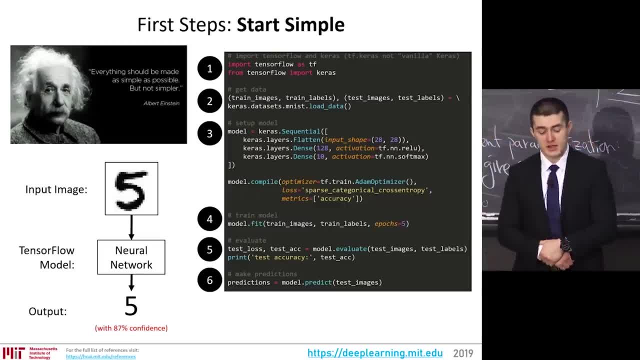 In step six. you're ready to deploy, You're ready to predict what's in the image. It's as simple as that. Much of this code- obviously much more complicated or much more elaborate and rich and interesting and complex- we'll be making available on GitHub, on our repository that accompanies. 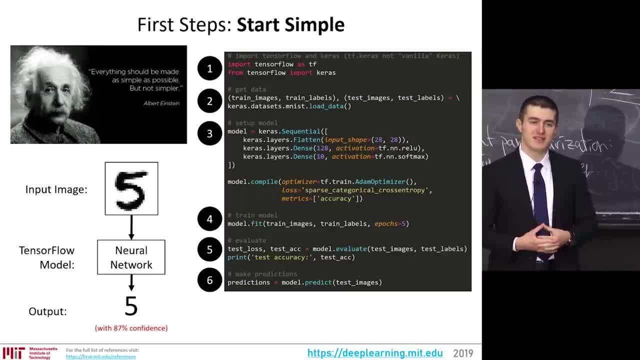 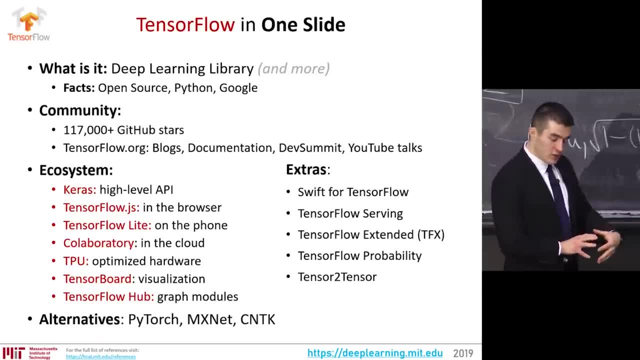 these courses. Today we've released the first tutorial on driver-seat segmentation. I encourage you to check it out. I encourage everybody to go through it. And then on the tooling side, in one slide before we dive into the neural networks and 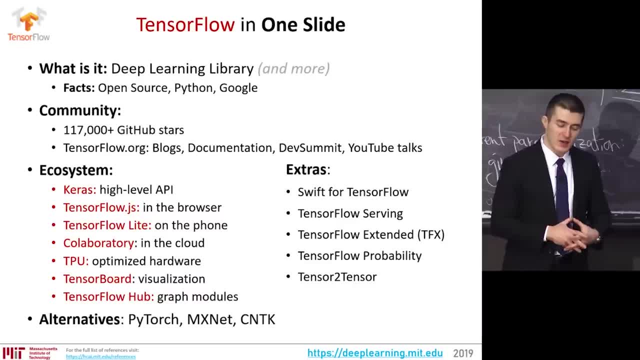 deep learning, the tooling side, amongst many other things. TensorFlow is a deep learning library, an open source library from Google, the most popular one to date, the most active, with a large ecosystem. It's not just something you import in Python and to solve some basic problems. 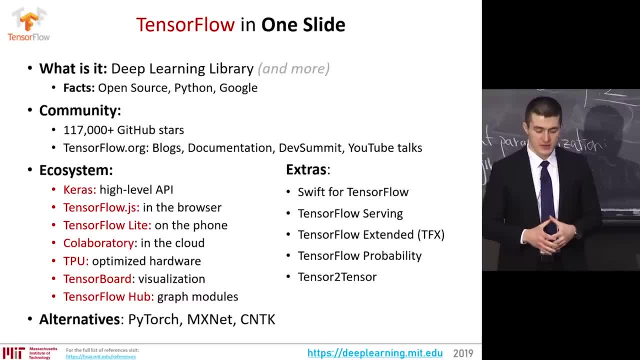 There's an entire ecosystem of tooling. There's different levels of APIs. Much of what we'll do in this course will be the highest level API with Keras, But there's also the ability to run in the browser with TensorFlowjs, on the phone with 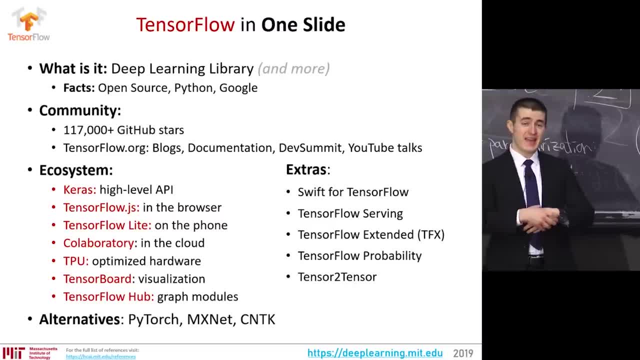 TensorFlow Lite in the cloud without any need to have a computer hardware or anything any of the libraries set up on your own machine. you can run all the code that we're providing in the cloud with Google Collab Collaboratory And the optimized ASICs hardware that Google has optimized for TensorFlow with their TPU. 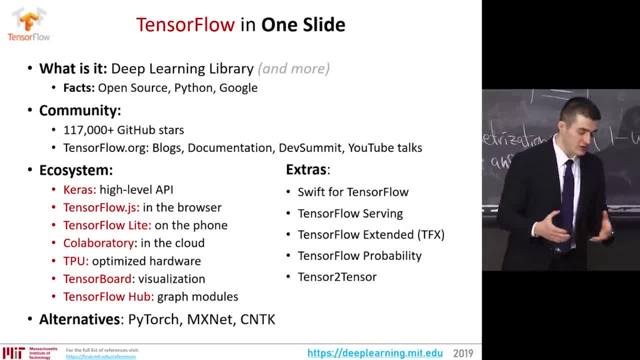 Tensor Processing Unit, ability to visualize TensorBoard models that are provided in TensorFlow Hub, And there's just an entire ecosystem including, most importantly, I think, documentation and blogs that make it extremely accessible to understand the fundamentals of the code. 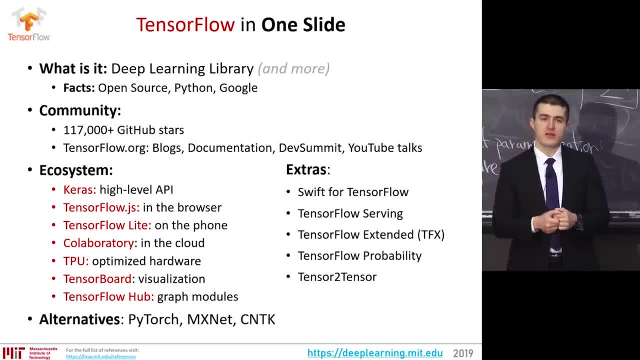 And that's what we're trying to do. So we're trying to provide the fundamentals of the tooling that allow you to solve the problems, from natural language processing to computer vision, to GANs, generative adversarial neural networks, and everything in between deep reinforcement, learning and so on. 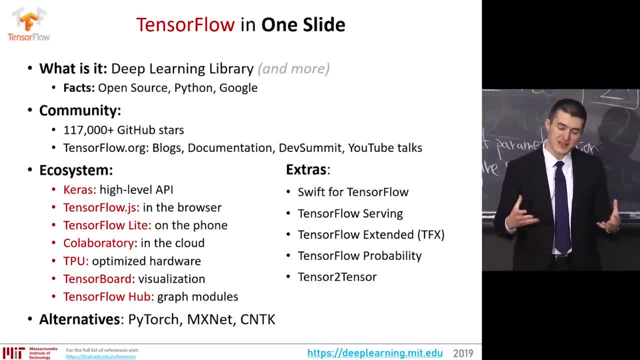 So that's why we're excited to sort of work both in the theory in this course, in this series of lectures, and in the tooling and the applied side of TensorFlow. It really makes it exceptionally, these ideas exceptionally accessible. So thank you. 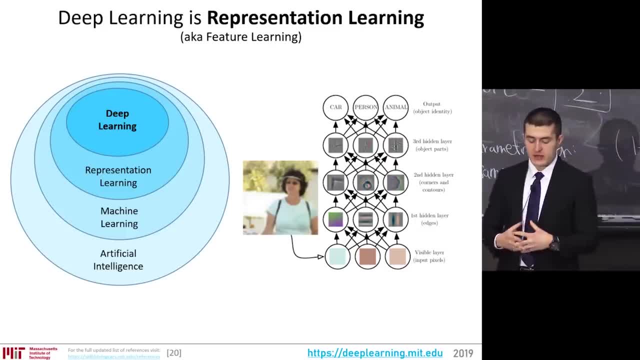 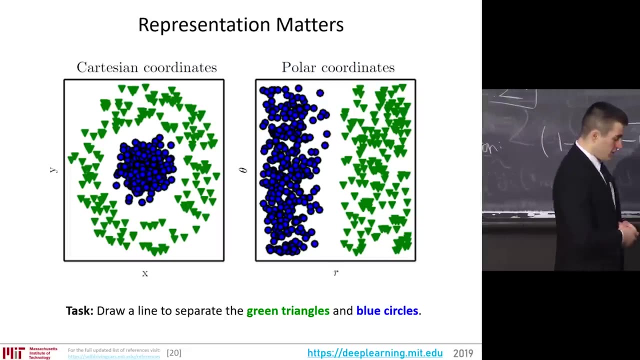 So deep learning. at the core is the ability to form higher and higher level of abstractions of representations in data and raw patterns. higher and higher levels of understanding of patterns And those representations are extremely important and effective for being able to interpret data- Data under certain representations. 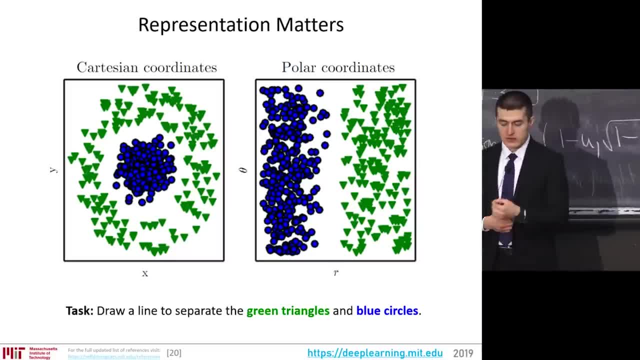 data is trivial to understand: Cat versus dog, blue dot versus green triangle. Under others it's much more difficult In this task. drawing a line under polar coordinates is trivial. Under Cartesian coordinates it's very difficult, well impossible, to do accurately. 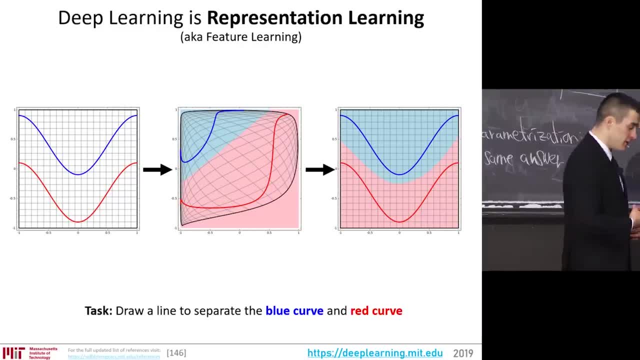 And that's a trivial example of a representation. So our task with deep learning, with machine learning and machine learning in general, is forming representations that map the topology- whatever the topology, the rich space of the problem that you're trying to deal with, of the raw inputs. 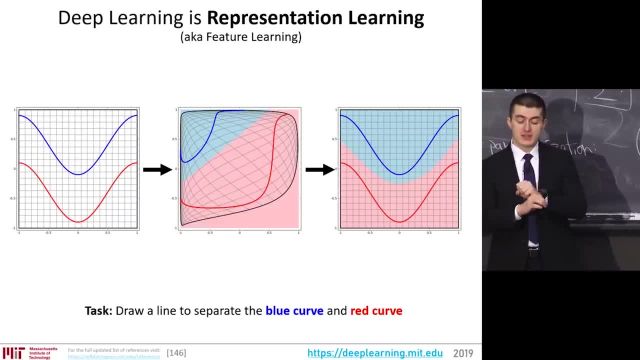 map it in such a way that the final representation is trivial to work with, trivial to classify, trivial to perform regression, trivial to generate new samples of that data. And that representation of higher and higher levels of representation is really the dream of artificial intelligence. 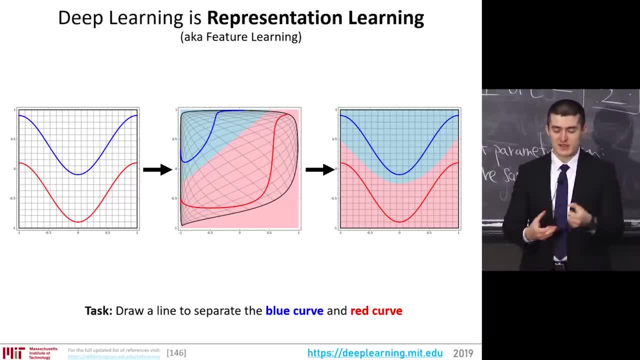 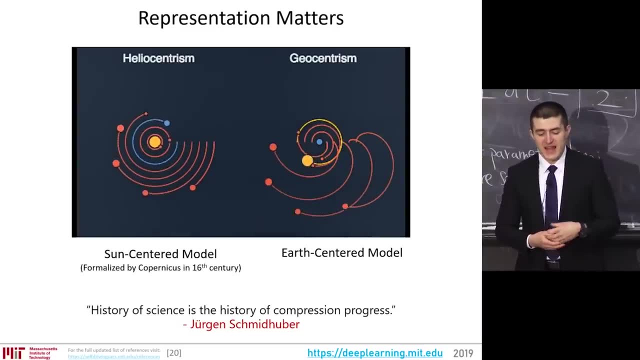 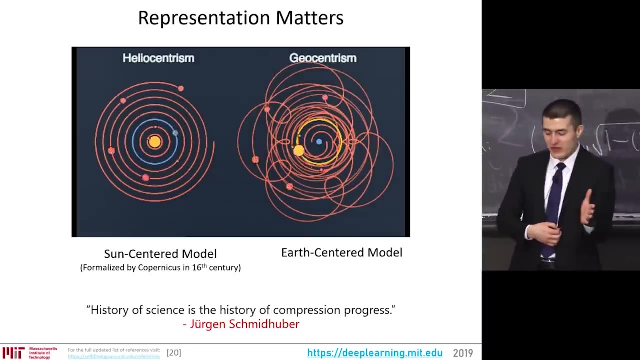 That is what understanding is: making the complex simple. like Einstein, back in a few slides ago, said, And that, with Juergen Schmidhuber and whoever else said it, I don't know- that's been the dream of all of science in general. 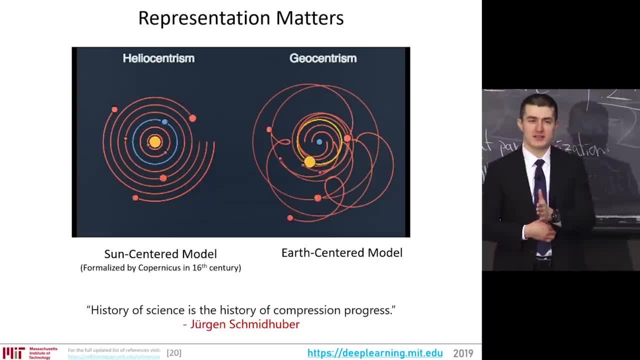 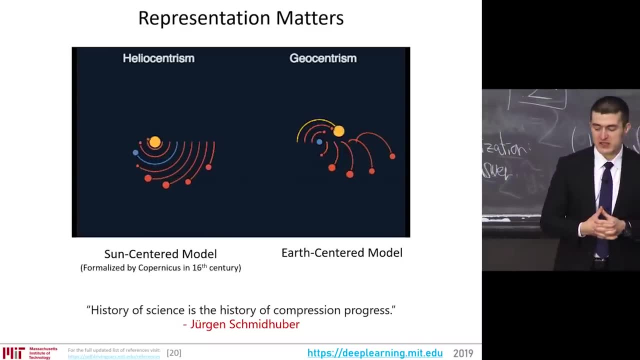 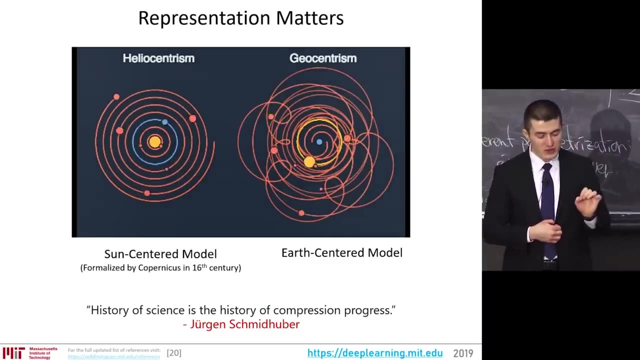 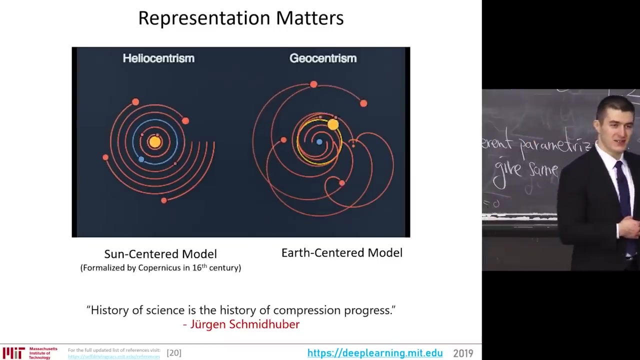 of the history of science is the history of compression, progress, Of forming simpler and simpler representations of ideas. The models of the universe, of our solar system, with the earth at the center of it, is much more complex to perform, to do physics on, than a model where the sun is at the center. 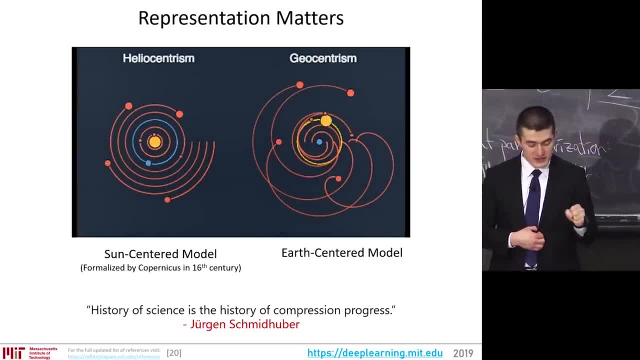 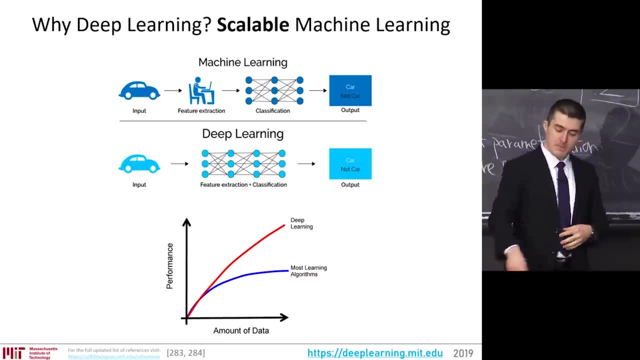 Those higher and higher levels of simple representations enable us to do extremely powerful things. That has been the dream of science and the dream of artificial intelligence. And why deep learning? What is so special about deep learning in the grander world of machine learning? 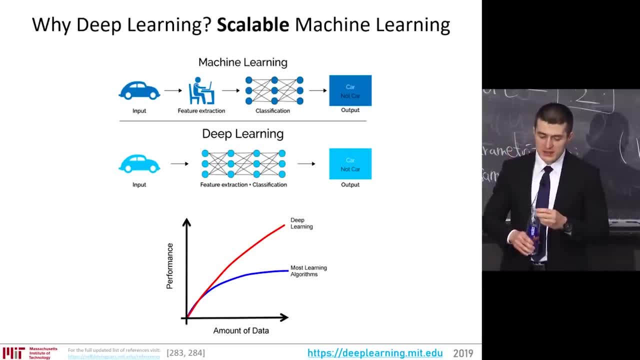 and artificial intelligence. It's the ability to more and more remove the input of human experts, remove the human from the picture, the human, costly, inefficient effort of human beings from the picture. Deep learning automates much of the extraction from the raw, gets us closer and closer to the raw data. 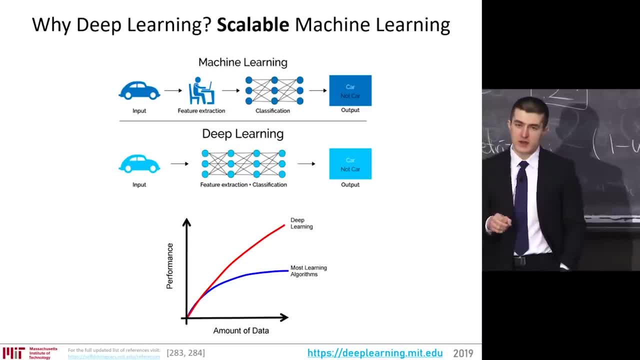 without the need of human involvement. human expert involvement. Ability to form representations from the raw data as opposed to having a human being. need to extract features, as was done in the 80s and 90s and the early aughts to extract features with which then. 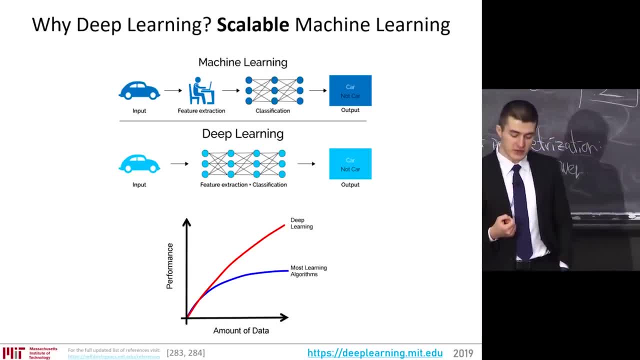 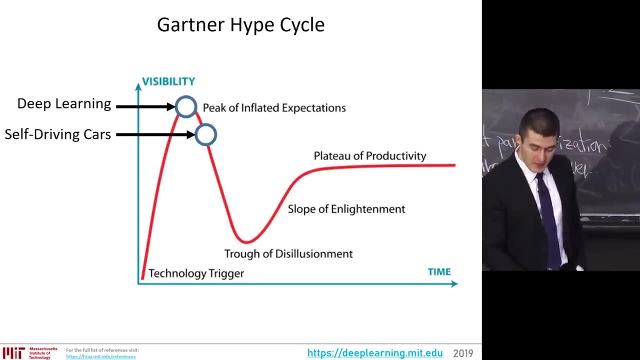 the machine learning algorithms can work with. The automated extraction of features enables us to work with large and large data sets, removing the human completely, except from the supervision labeling step. at the very end It doesn't require the human expert. But at the same time, there is limits to our technologies. 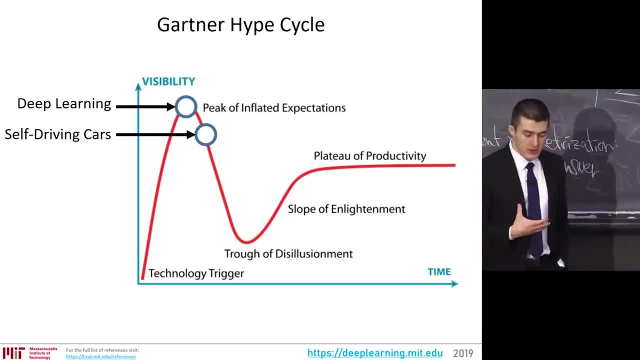 There's always a balance between excitement and disillusionment. The Gartner hype cycle, as much as we don't like to think about it, applies to almost every single technology. Of course, the magnitude of the peaks and the draws is different. 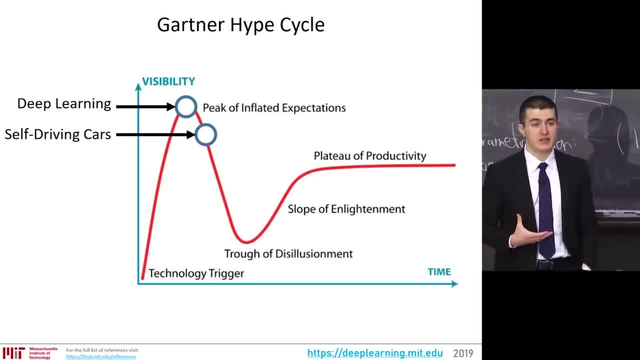 But I would say we're at the peak of an inflated expectation with deep learning, And that's something we have to think about as we talk about some of the ideas and the exciting possibilities of the future, And with self-driving cars that we'll talk about in future lectures in this course- we're at the same. 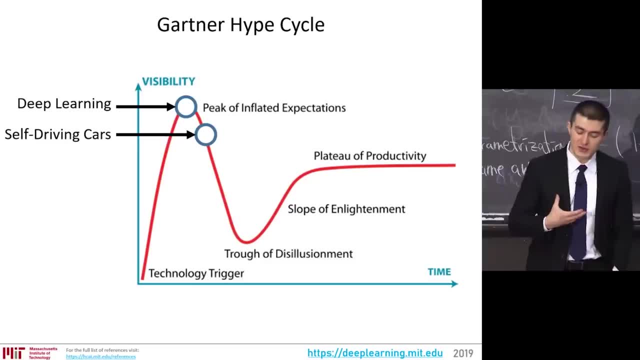 In fact, we're a little bit beyond the peak, And so it's up to us- This is a big deal, Thank you. This is MIT and the engineers and the people working on this in the world to carry us through the draw. 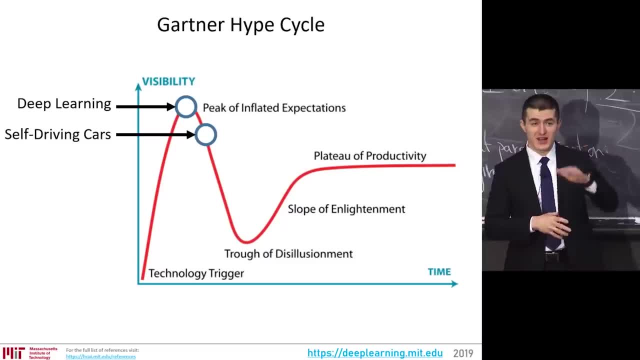 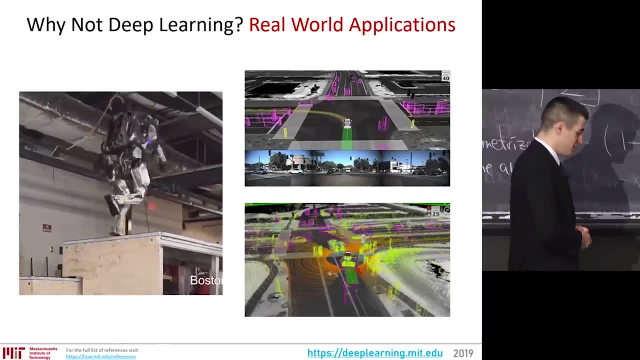 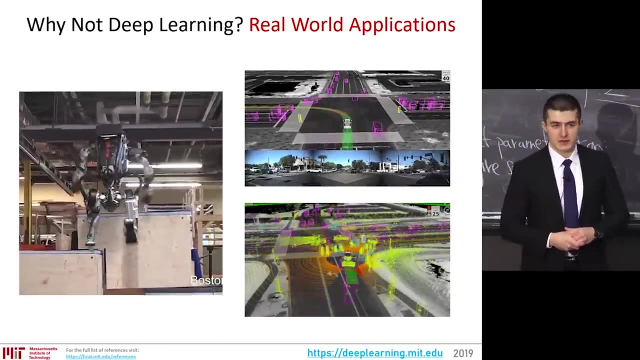 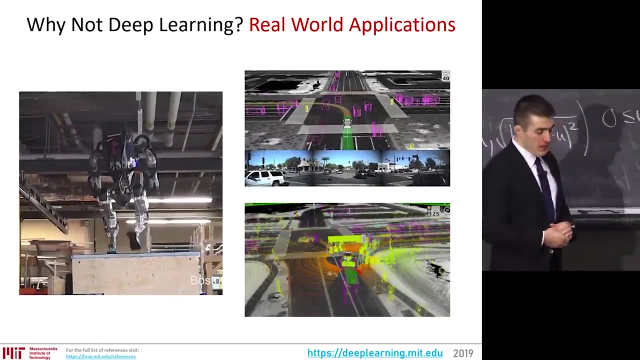 to carry us through the future as the ups and downs of the excitement progresses forward into the plateau of productivity. Why else not deep learning, If we look at real world applications, especially with humanoid robotics, robotic manipulation and even, yes, autonomous vehicles. 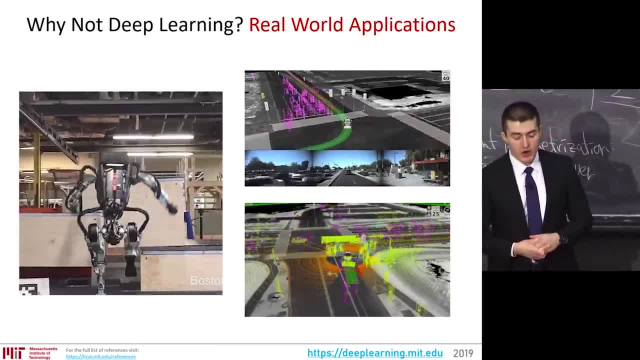 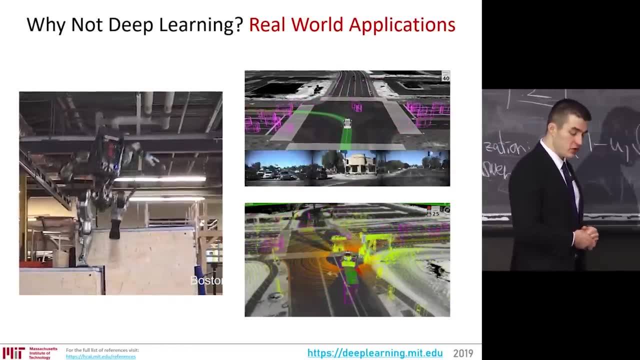 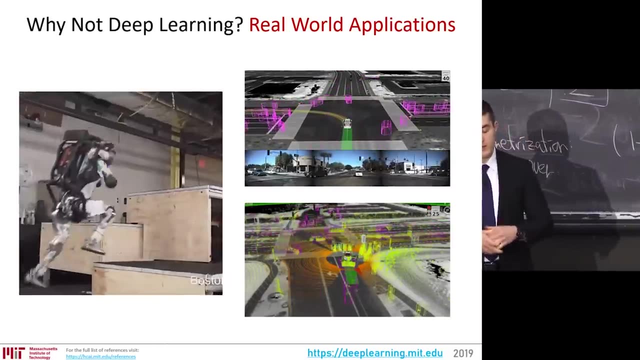 majority of the aspects of the autonomous vehicles do not involve to an extensive amount machine learning. to date, The problems are not formulated as data-driven learning. Instead, they're model-based optimization methods that don't learn from data over time And then from the speakers these couple of weeks. 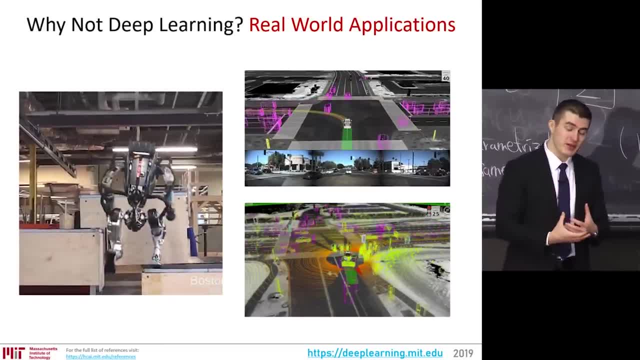 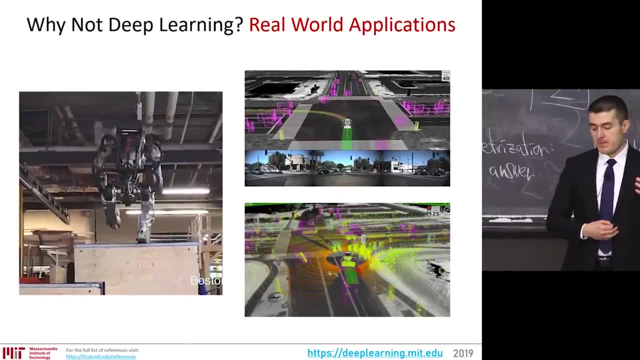 we'll get to see how much machine learning is starting to creep in. But an example. An example is shown here with the Boston, with amazing humanoid robotics and Boston Dynamics. To date, almost no machine learning has been used, except for trivial perception. 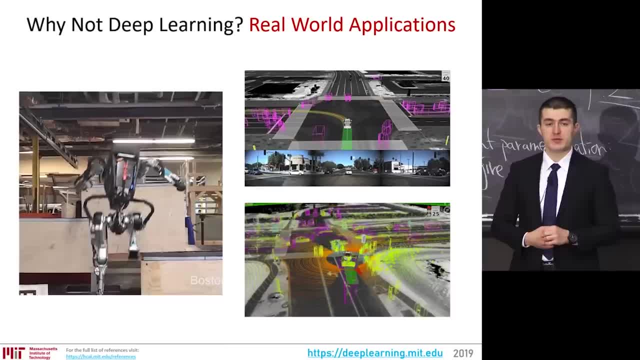 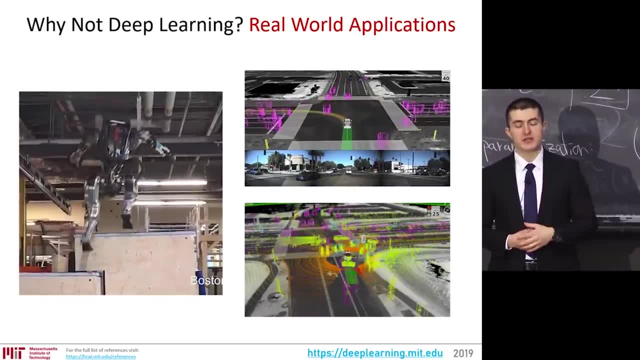 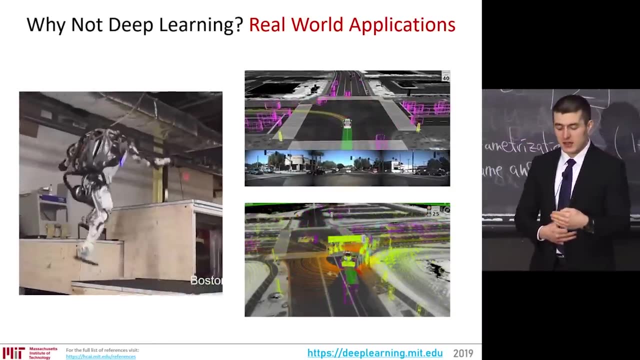 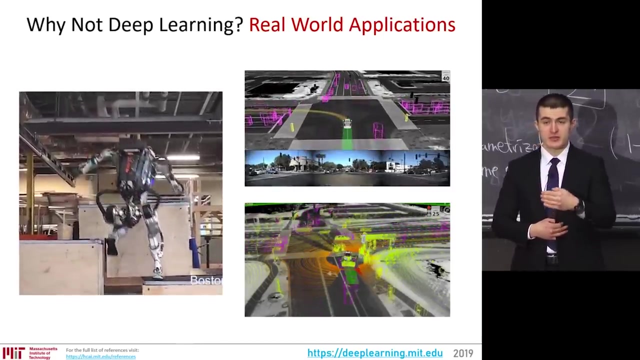 The same with autonomous vehicles. Almost no machine learning and deep learning has been used, except with perception, Some aspect of enhanced perception from the visual texture information Plus. what's starting to be used a little bit more is the use of recurrent neural networks to predict the future, to predict the intent. 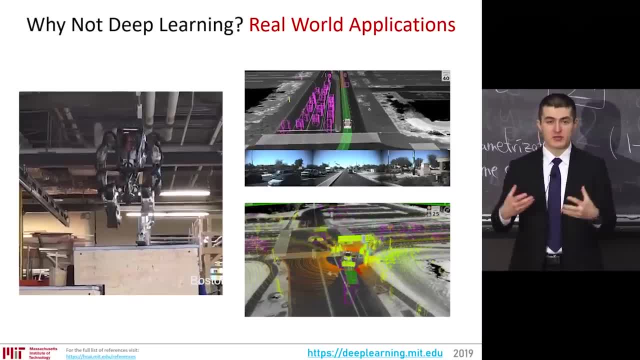 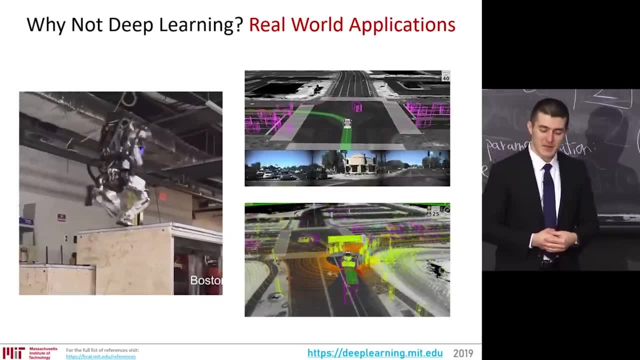 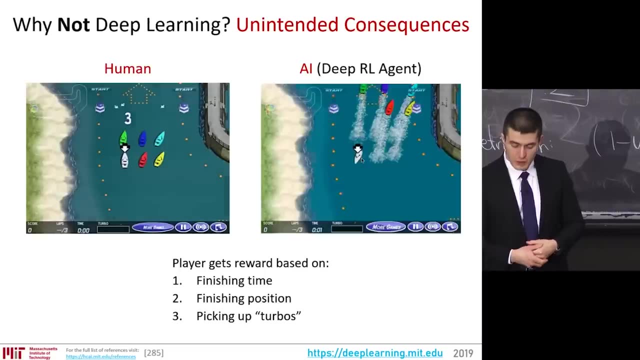 of the different players in the scene in order to anticipate what the future is. But these are very early steps. Most of the success that you see today- the 10 million miles that Waymo has achieved- has been attributed mostly to non-machine learning methods. 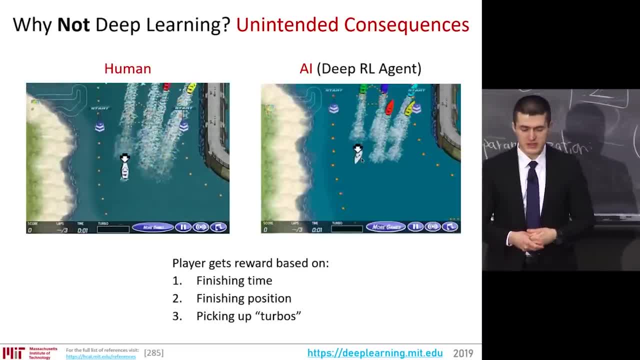 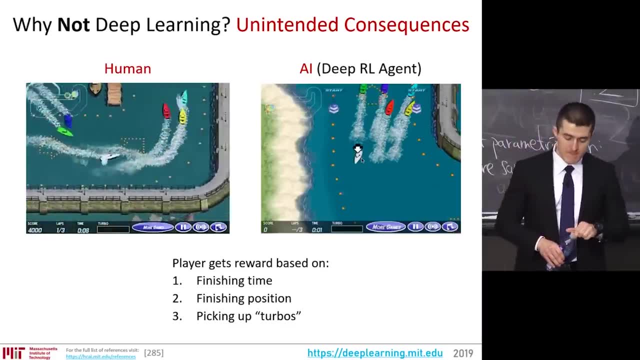 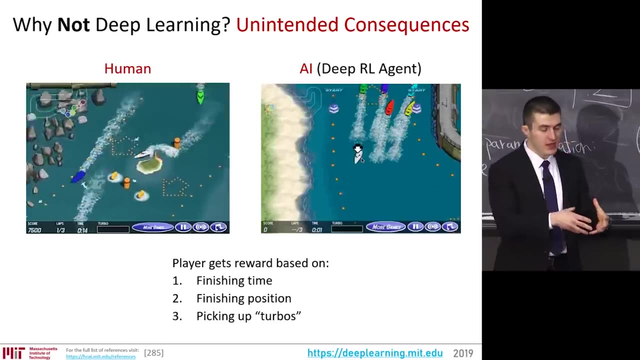 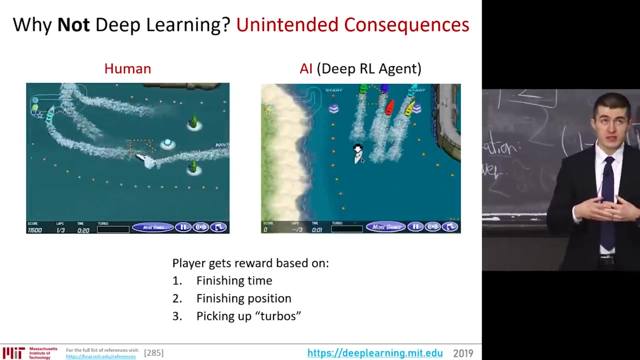 Why else not deep learning? Here's a really clean example of unintended consequences, Of ethical issues we have to really think about When an algorithm learns from data based on an objective function, a lost function, the power, the consequences of an algorithm. 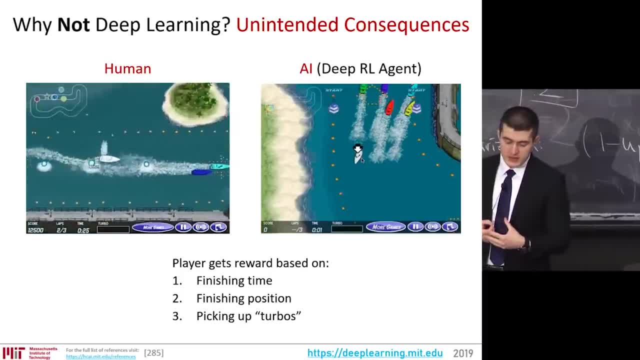 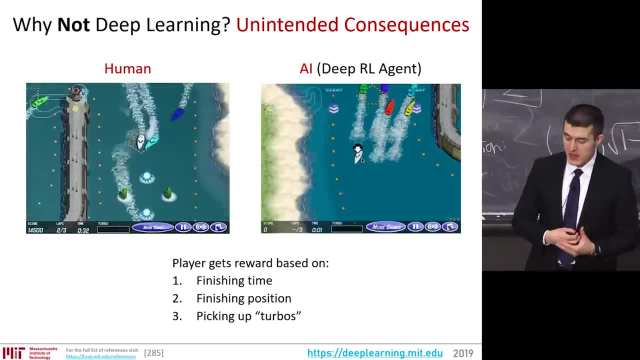 that optimizes that function is not always obvious. Here's an example of a human player playing games. In the game of Coast Runners. it's a boat racing game where the task is to go around the racetrack and try to win the race. 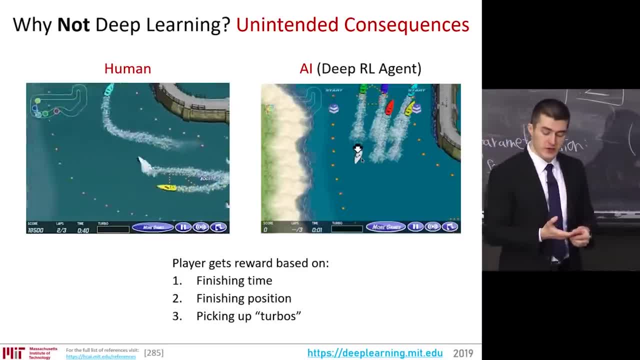 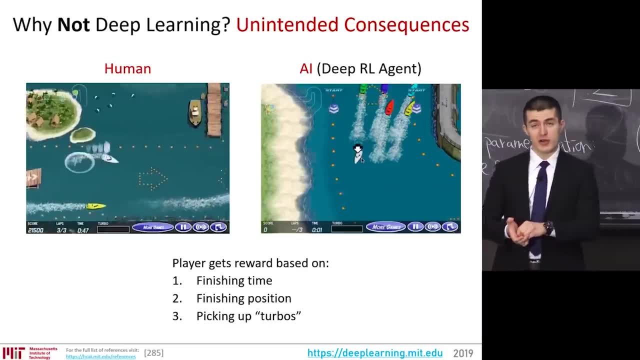 And the objective is to get as many points as possible. There are three ways to get points: The finishing time, how long it took you to finish. the finishing position where you were in the ranking and picking up. quote: unquote turbos. 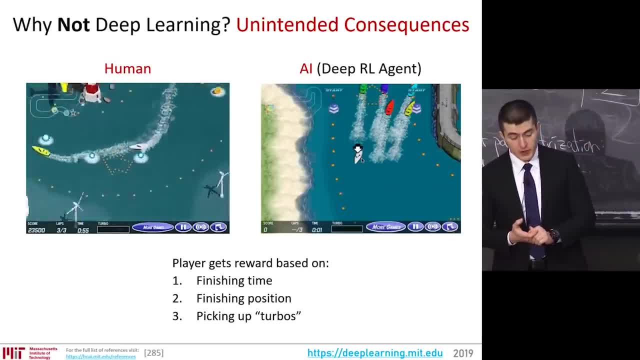 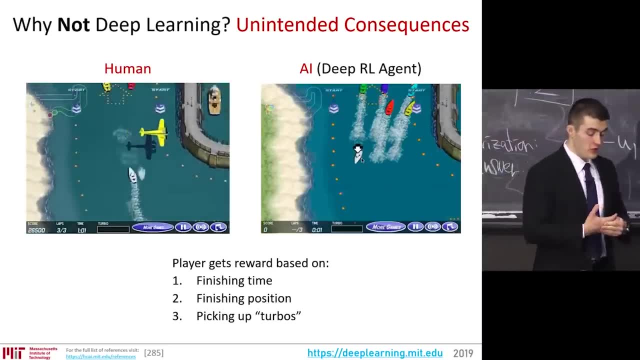 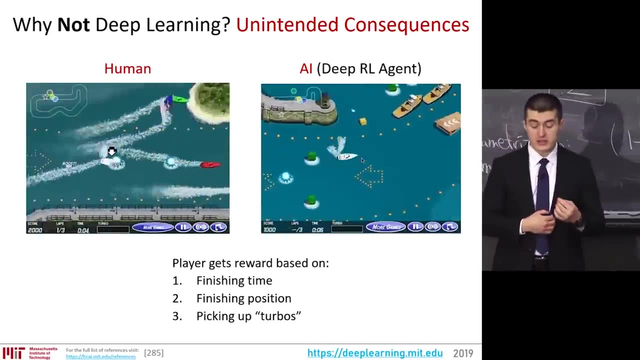 those little green things along the way. they give you points. Okay, simple enough. So we design an agent, in this case an RL agent, that optimizes for the rewards And what we find on the right here: the optimal. the agent discovers that the optimal. 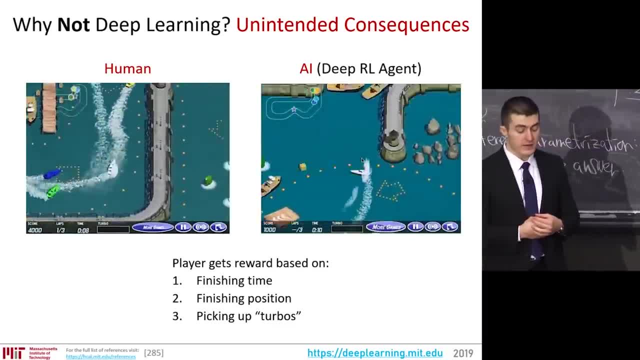 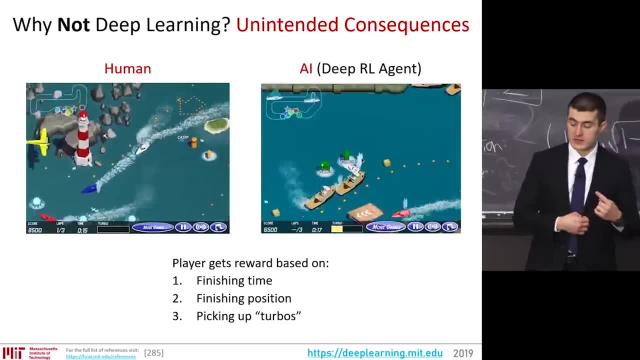 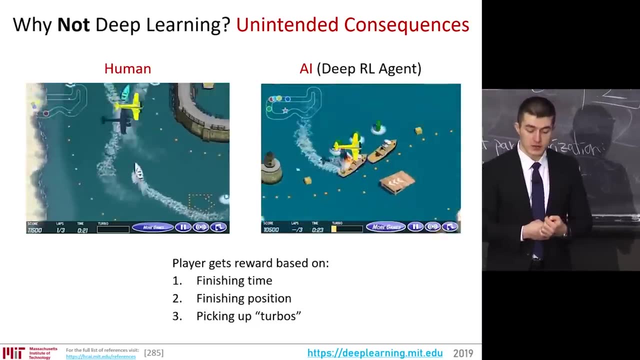 actually has nothing to do with finishing the race or the ranking. They can get much more points by just focusing on the turbos and collecting those little green dots, because they regenerate. So you go in circles, over and over and over, slamming into the wall, collecting the green turbos. 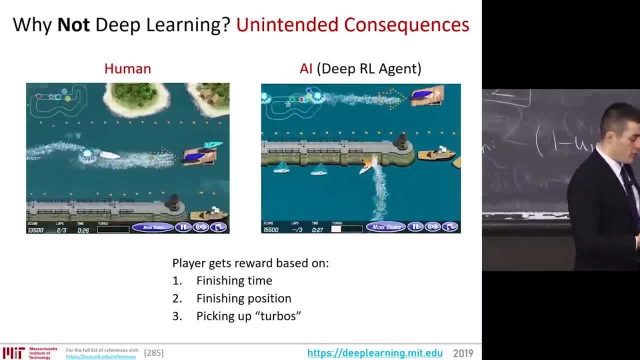 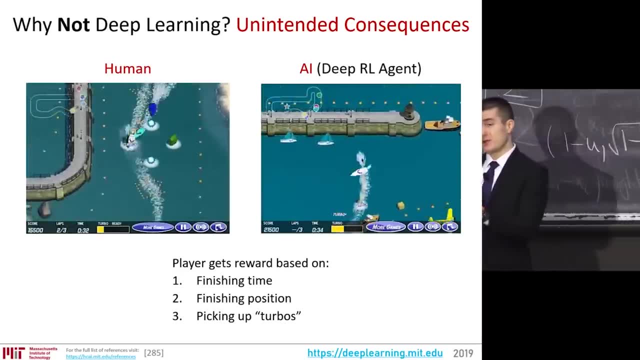 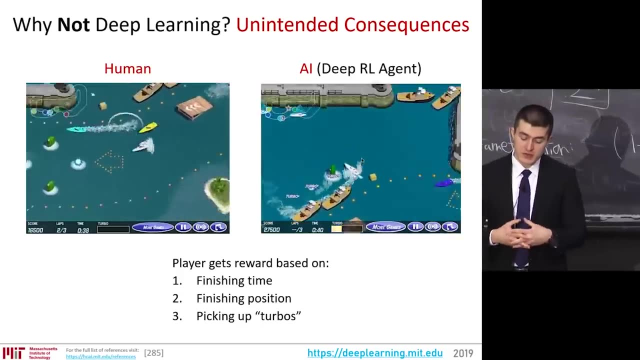 Now that's a very clear example of a well-reasoned, formulated objective function that has totally unexpected consequences, at least without sort of considering those consequences ahead of time, And so that shows the need for AI safety for a human in the loop of machine learning. 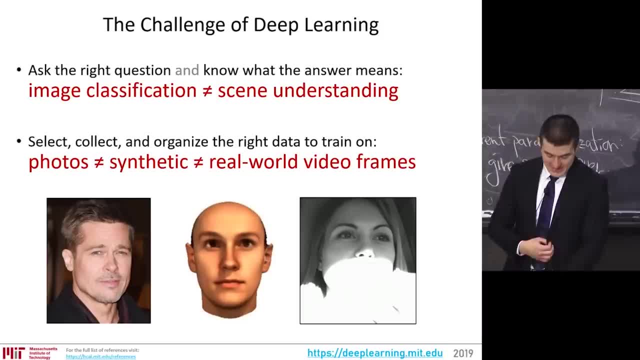 That's why not deep learning, deep learning exclusively. The challenge of deep learning, algorithms, of deep learning applied, is to ask the right question and understand what the answers mean. You have to take a step back and look at the difference, the distinction. 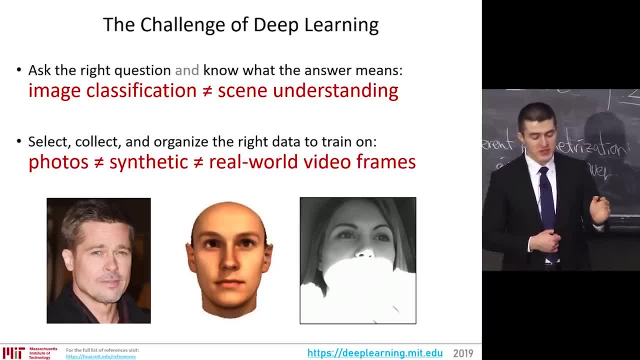 the levels, degrees of what the algorithm is accomplishing. For example, image classification is not necessarily scene understanding. In fact, it's very far from scene understanding. Classification may be very far from understanding And the data sets can vary drastically across the different benchmarks in the data sets used. 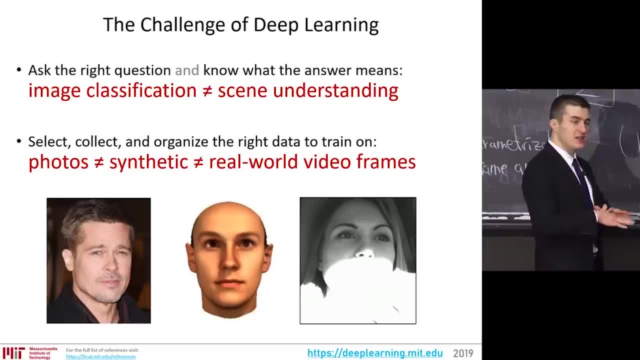 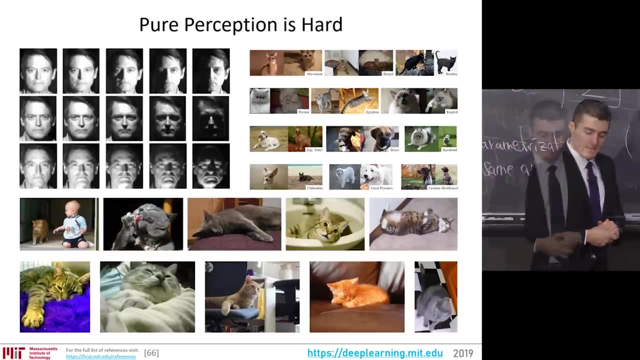 The professionally done photographs versus synthetically generated images, versus real-world data- And the real-world data is where the big impact is, So oftentimes the one doesn't transfer to the other. That's the challenge of deep learning: Solving all of these problems. 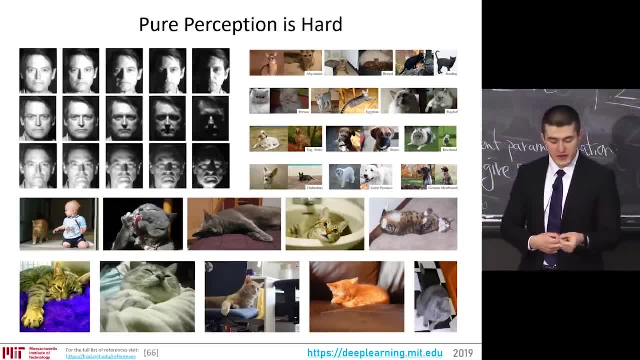 of different lighting, variations of pose variation, inter-class variation, all the things that we take for granted as human beings, with our incredible perception system, all have to be solved in order to gain greater and greater understanding of a scene, And all the other things we have to close the gap on. 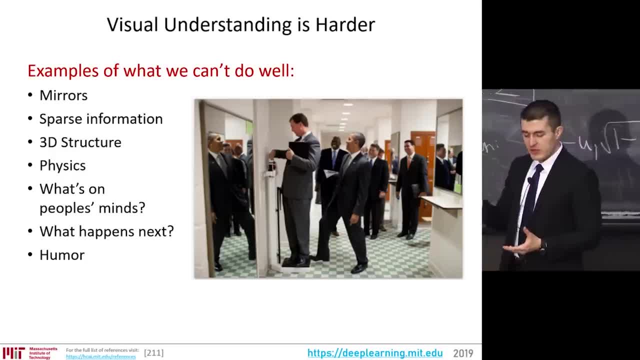 that we're not even close to yet. Here's an image from the Andrej Karpathy blog from a few years ago of former President Obama stepping on a scale. We can classify, we can do semantic segmentation of the scene, we can do object detection. 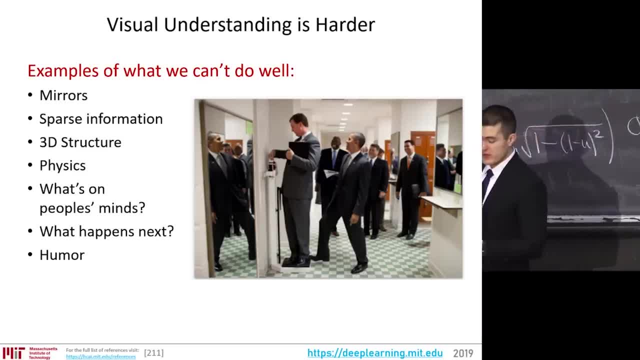 we can do a little bit of 3D reconstruction from a video version of the scene. But what we can't do well is all the things we take for granted. We can't tell the images in the mirrors versus in reality as different. We can't deal with the sparsity of information. 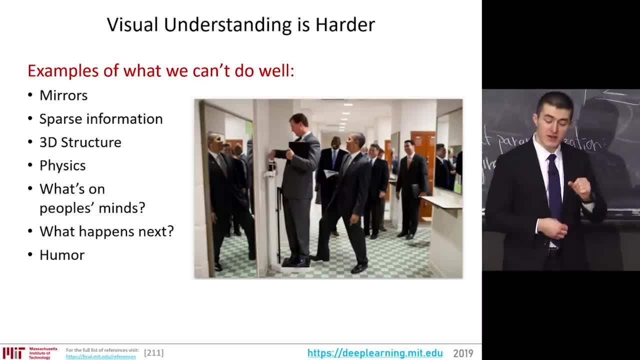 Just a few pixels on President Obama's face, we can still identify him as the President. The 3D structure of the scene, that there's a foot on top of a scale, that there's human beings behind, from a single image, things we can trivially do using. 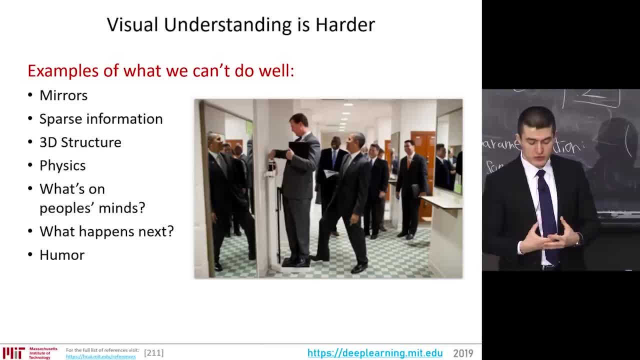 all the common sense, semantic knowledge that we have cannot do The physics of the scene, that there's gravity and the biggest thing, the hardest thing, is what's on people's minds And what's on people's minds about what's on other people's minds. 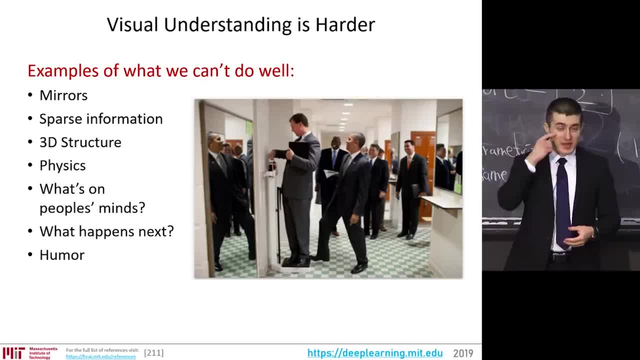 And so on. Mental models of the world, Being able to infer what people are thinking about. Being able to infer: there's been a lot of exciting work here at MIT about what people are looking at, But we're not even close to solving that problem either. 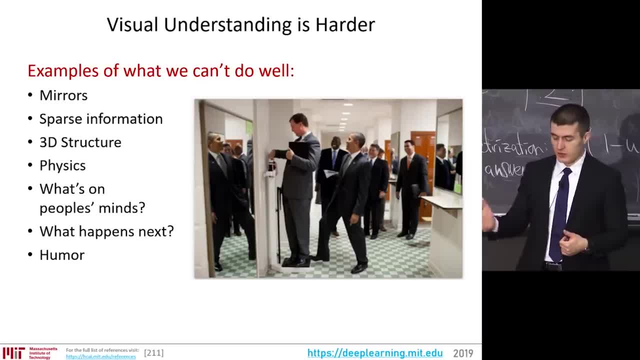 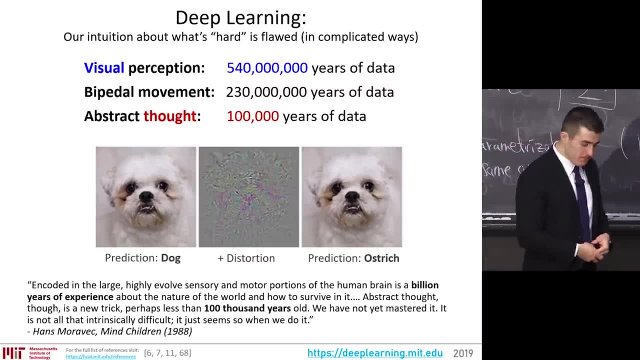 But what they're thinking about? we're not even. we haven't even begun to really think about that problem and we do it trivially as human beings. And I think at the core of that, I think I'm harboring on the visual perception problem. 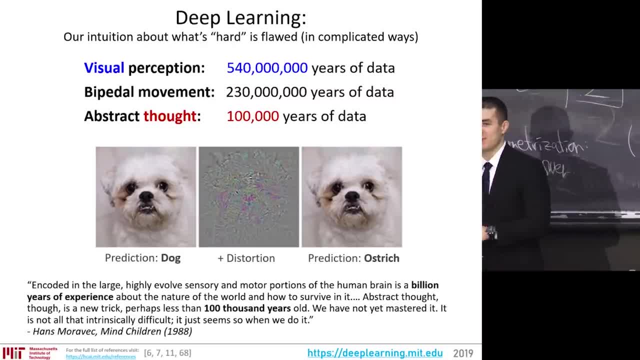 because it's one we take really for granted as human beings, especially when trying to solve real world problems, especially when trying to solve autonomous driving is. we have 540 million years of data for visual perception, so we take it for granted. We don't realize how difficult it is. 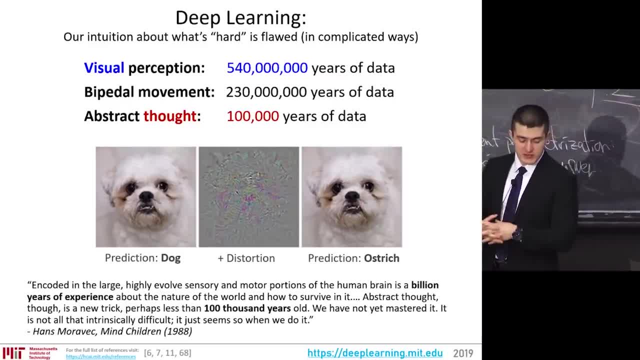 And we kind of focus all our attention on this recent development of 100,000 years of abstract thought, being able to play chess, being able to reason, But the visual perception is nevertheless extremely difficult at every single layer of what's required to perceive, interpret and understand. 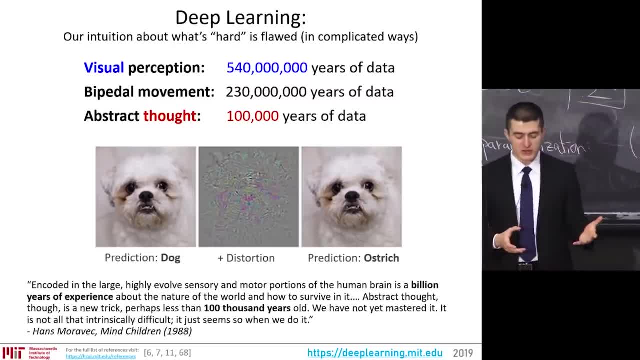 the fundamentals of a scene And a trivial way to show. that is just all the ways you can mess with these image classification systems by adding a little bit of noise. The last few years there's been a lot of papers, a lot of work to show that you can mess with these systems. 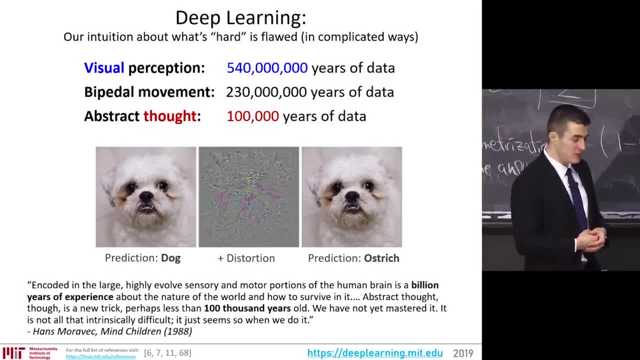 by adding noise Here, with 99% accuracy predict a dog. add a little bit of distortion. Immediately the system predicts with 99% accuracy that it's an ostrich And you can do that kind of manipulation with just a single pixel. 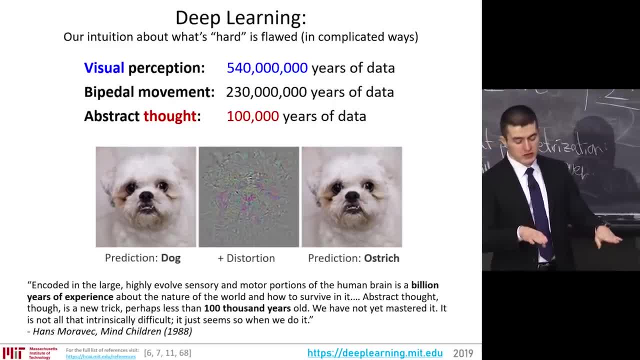 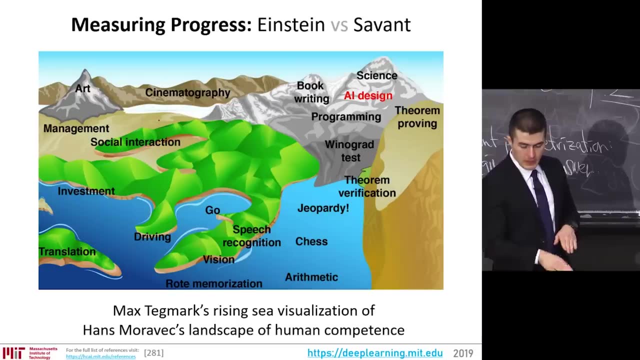 So that's just a clean way to show the gap between image classification on an artificial data set like ImageNet and real world perception. that has to be solved, especially for life-critical situations like autonomous driving. I really like this Max Tegmark's visualization. 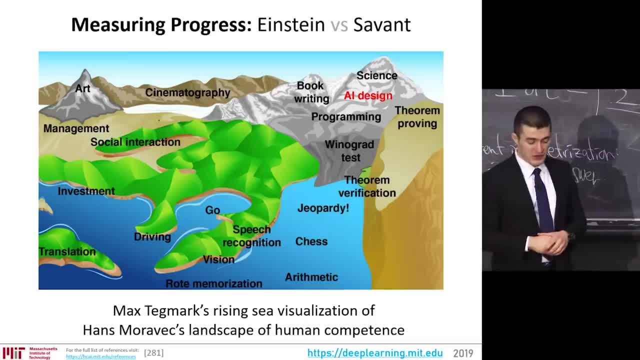 of this rising sea, of the landscape of human competence from Hans Maravec. And this is the difference, as we progress forward and we discuss some of these machine learning methods- is there is the human intelligence, the general human intelligence. let's call Einstein here. 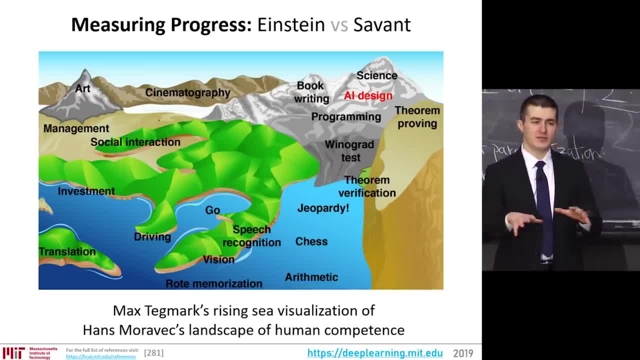 that's able to generalize over all kinds of problems, over all kinds of from the common sense to the incredibly complex. And then there is the way we've been doing, especially data-driven machine learning, which is savants, which is specialized intelligence. 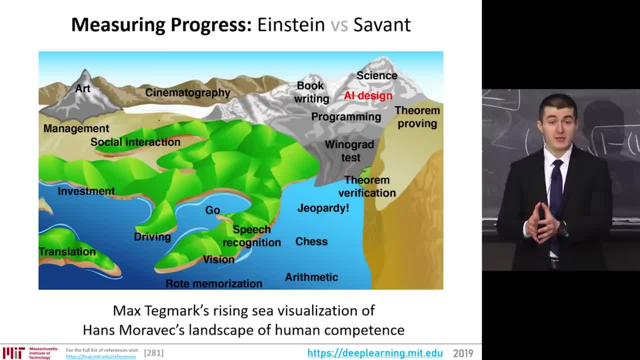 extremely smart at a particular task but not being able to transfer, except in the very narrow neighborhood, on this little landscape of different of art, cinematography, book writing at the peaks and chess, arithmetic and theorem proving and vision at the bottom in the lake. 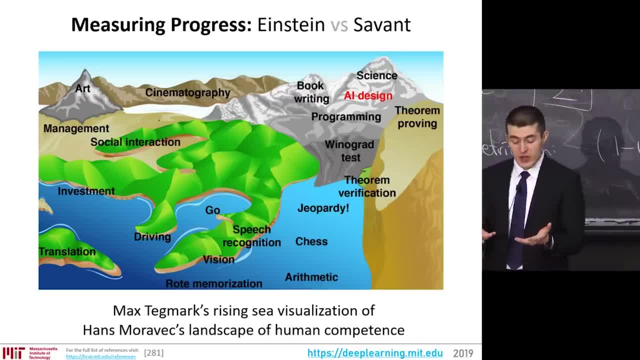 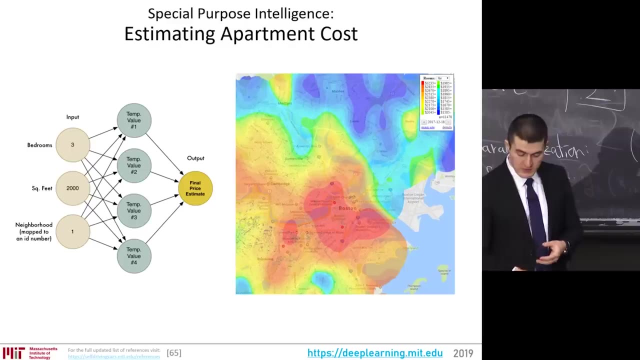 And there's this rising sea as we solve problem after problem. The question: can the methodology and the approach of deep learning of everything we're doing now keep the sea rising, Or do fundamental breakthroughs have to happen in order to generalize and solve these problems? 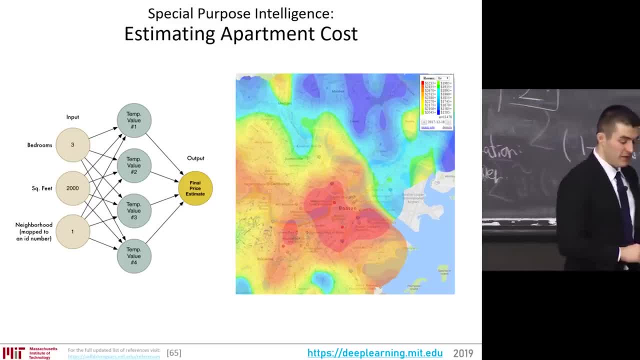 And so, from the specialized where the successes are. the systems are essentially boiled down to: given the dataset and given the ground truth for that dataset- here's the apartment cost in the Boston area- be able to input several parameters and, based on those parameters, 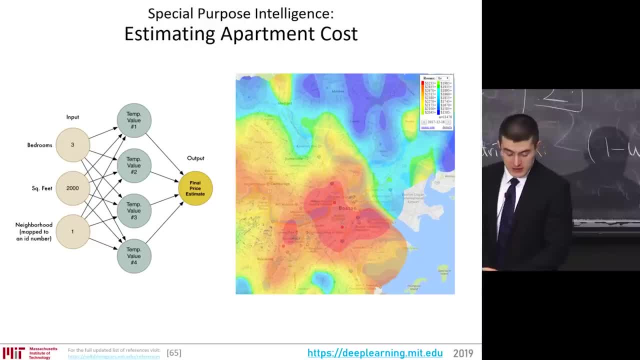 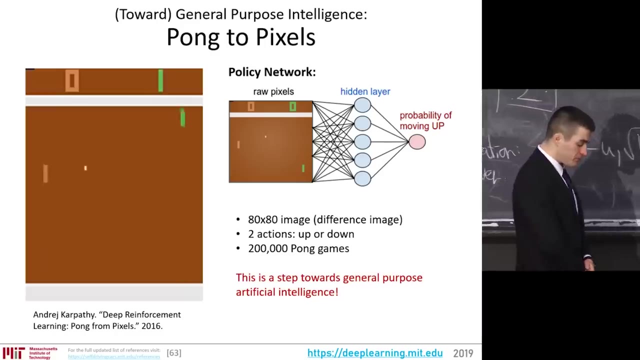 predict the apartment cost. That's the basic premise approach behind the successes- successful supervised deep learning systems today. If you have good enough data, that's good enough ground truth and can be formalized, we can solve it. Some of the recent promise: 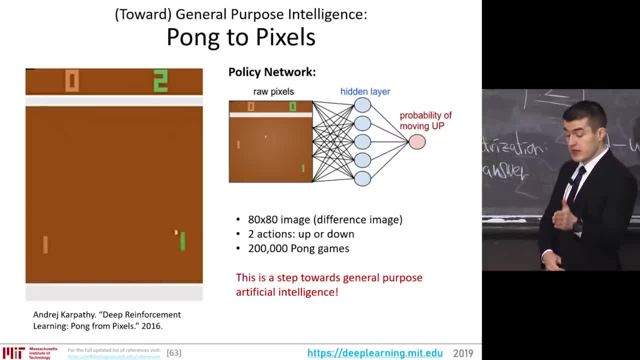 that we will do an entire series of lectures in the third week on deep reinforcement learning showed that from raw sensory information with very little annotation through self-play, whether systems learn without human supervision, are able to perform extremely well in these constrained contexts. The question of a video game: 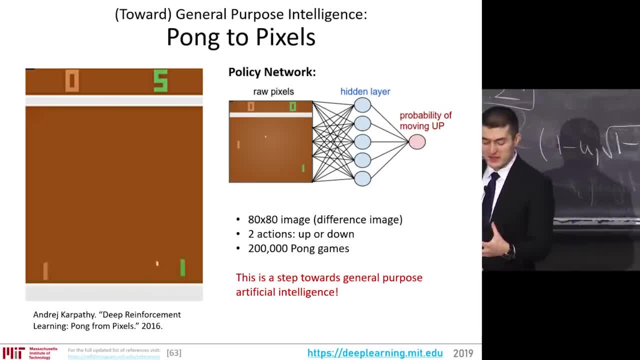 Here: pong to pixels. being able to perceive the raw pixels of this pong game as raw input and learn the fundamental quote-unquote physics of this game, Understand how it is this game behaves and how to be able to win this game, That's kind of a step toward. 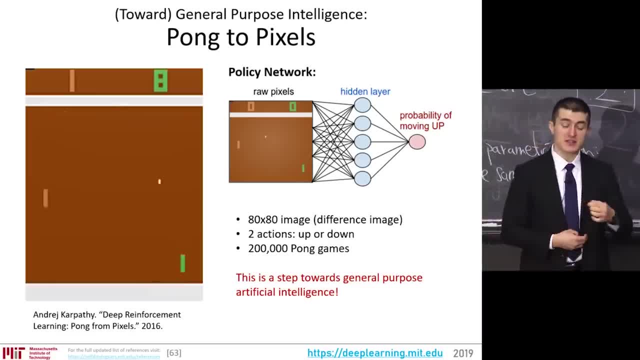 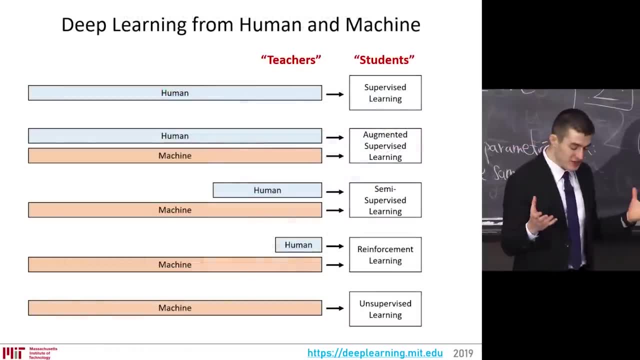 general purpose artificial intelligence. But it is a very small step because it's in a simulated, very trivial situation. That's the challenge that's before us. Would less and less human supervision be able to solve huge real-world problems From the up top supervised learning? 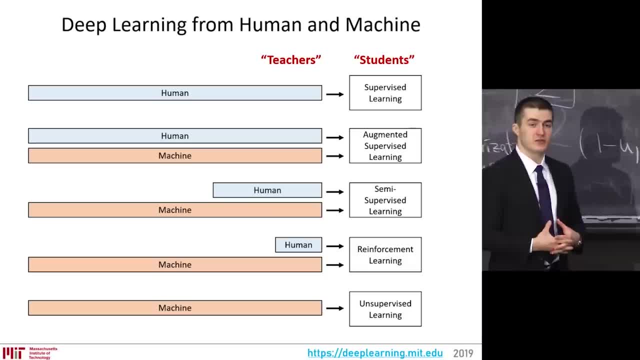 where majority of the teaching is done by human beings, throughout the annotation process, through labeling all the data, by showing different examples And further and further down to semi-supervised learning, reinforcement learning and supervised learning, Removing the teacher from the picture And 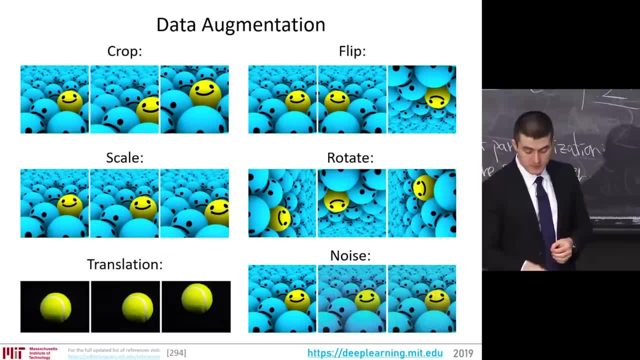 making that teacher extremely efficient when it is needed. Of course, data augmentation is one way, as we'll talk about. So taking a small number of examples and messing with that set of examples, augmenting that set of examples through trivial and through complex methods. 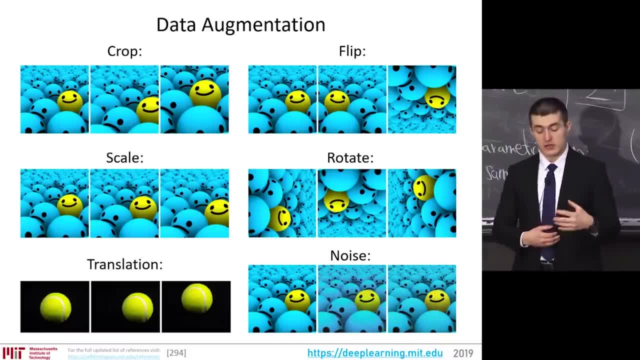 of cropping, stretching, shifting and so on, including through generative networks, modifying those images, to grow a small data set into a large one, to minimize, to decrease further and further the input that the human is, the input of the human teacher. 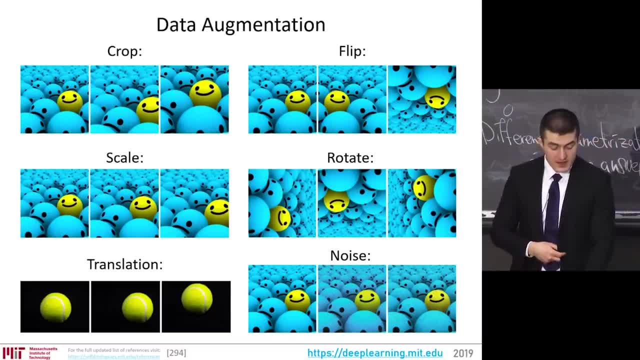 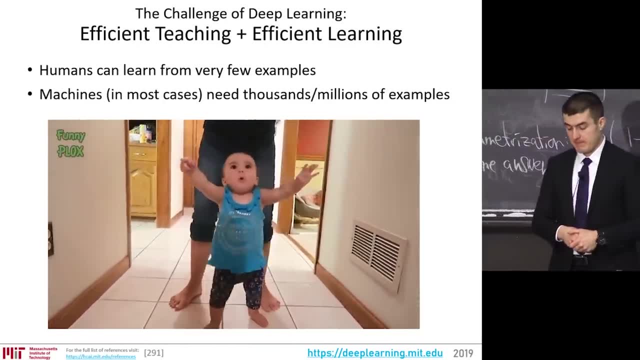 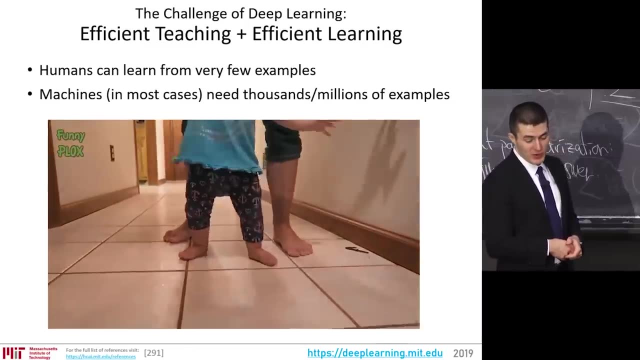 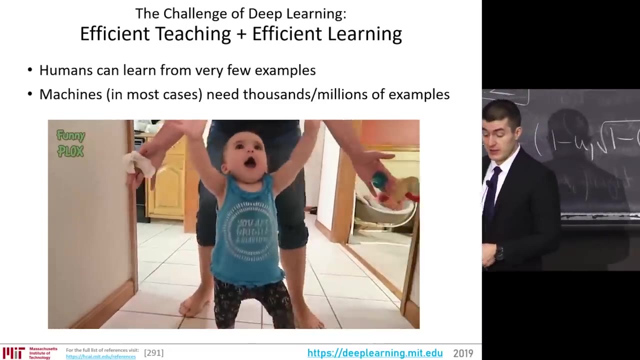 But still that's quite far away from the incredibly efficient, both teaching and learning that humans do. This is a video and there's many of them online. for the first time, a human baby walking We learn to do this. it's one-shot learning. 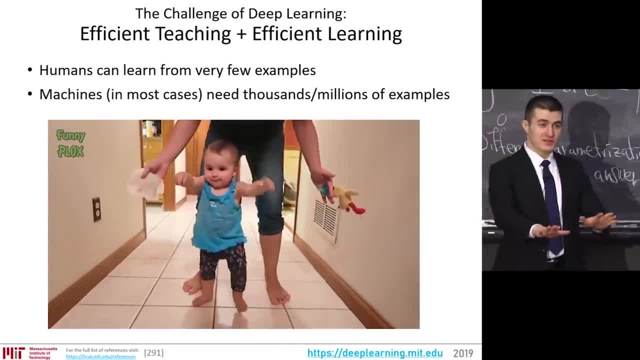 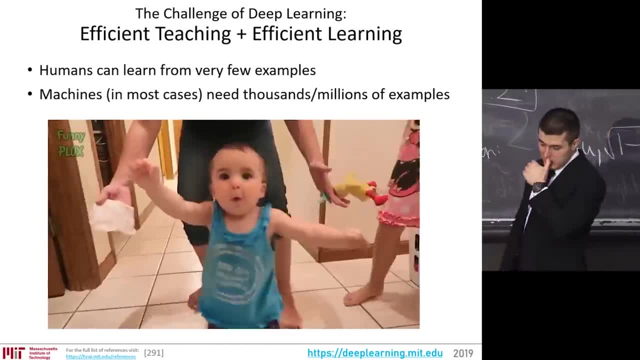 One day you're on all fours and the next day you put your two hands up and then you figure out the rest. One shot. Well, you can kind of. you can kind of play around with it, But the point is: 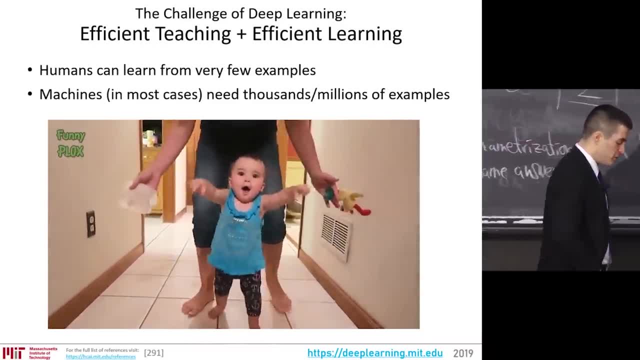 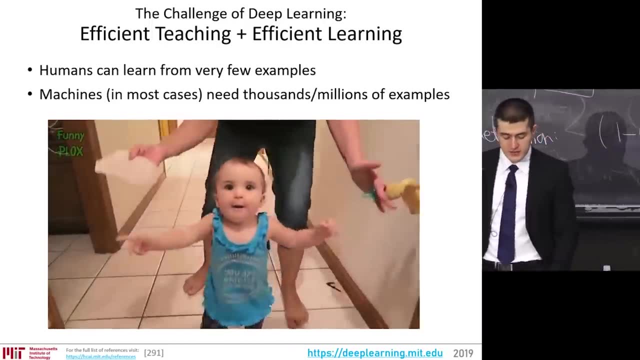 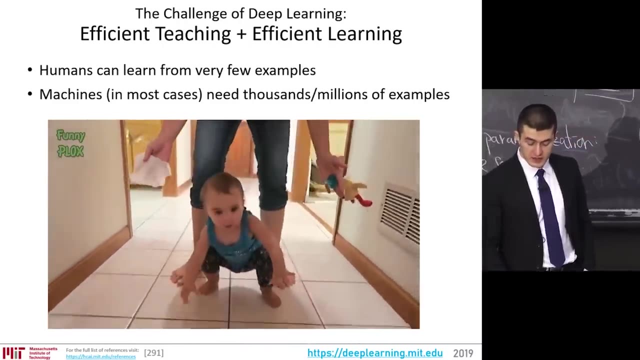 you're extremely efficient. With only a few examples, you're able to learn the fundamental aspect of how to solve a particular problem. Machines in most cases need thousands, millions and sometimes more examples, depending on the life-critical nature of the application. 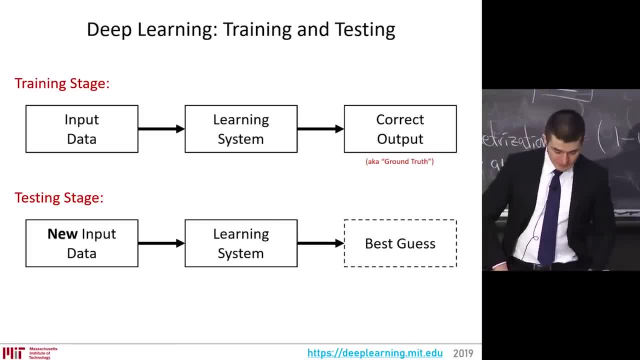 The data flow of supervised learning systems is: there's input data, there's a learning system and there is output. Now, in the training stage for the output, we have the ground truth, and so we use that ground truth to teach the system. 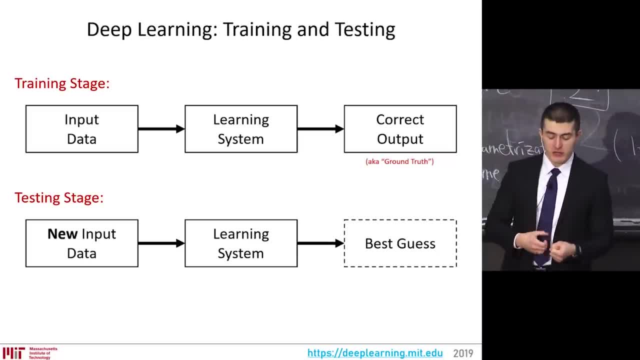 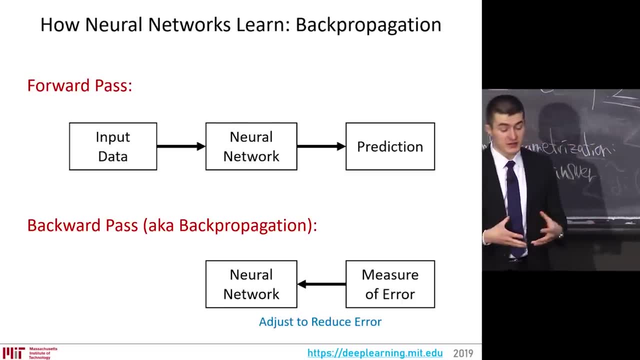 In the testing stage, when it goes out into the wild, there's new input data over which we have to generalize with the learning system and we have to make our best guess. In the training stage the process is with neural networks. 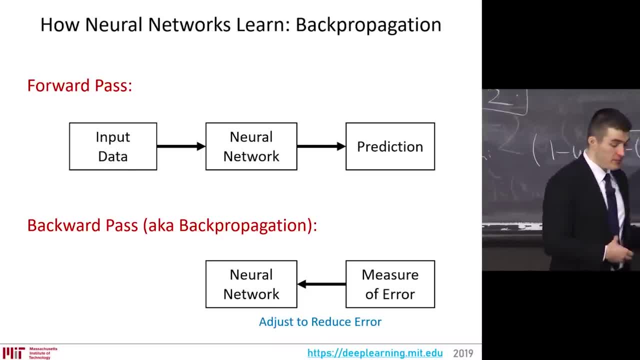 is: given the input data for which we have the ground truth, pass it through the model, get the prediction and, given that we have the ground truth, we can compare the prediction to the ground truth, look at the error and, based on that error, 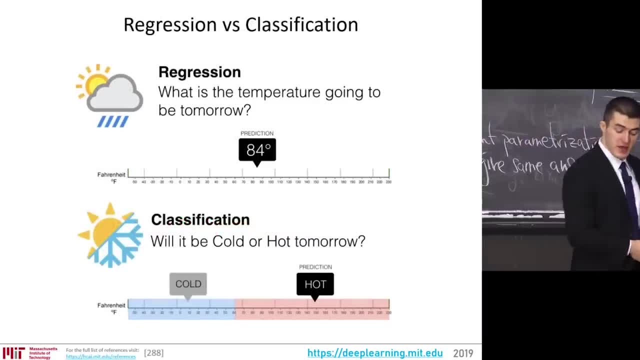 adjust the weights. The types of predictions we can make is regression and classification. Regression is a continuous and classification is categorical Here. if we look at what is, if we look at what is the weather, the regression problem says what is the temperature. 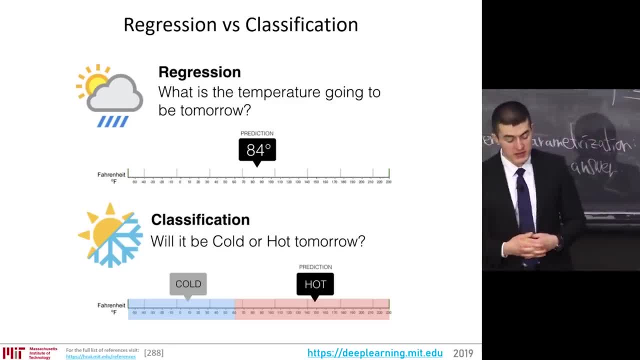 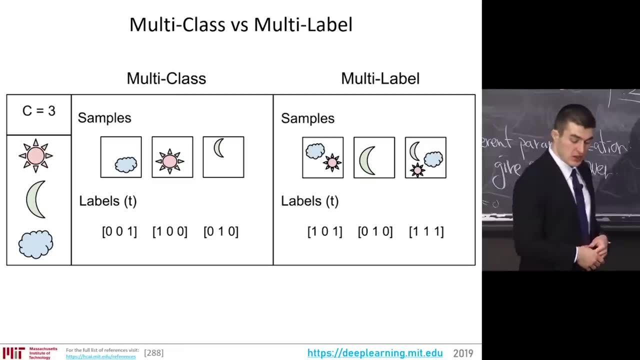 going to be tomorrow and the classification formulation of that problem says: is it going to be hot or cold or some threshold definition of what hot or cold is? That's regression classification. On the classification front, it could be multi-class, which is the standard formulation. 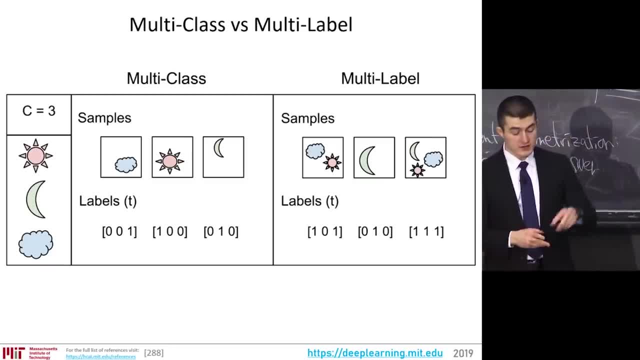 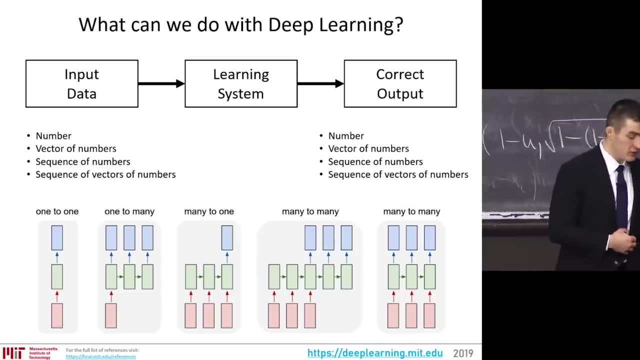 where you're tasked with saying what is. there's only a particular entity can only be one thing, and then there's multi-label, where a particular entity can be multiple things And overall the input to the system can be not just a single sample. 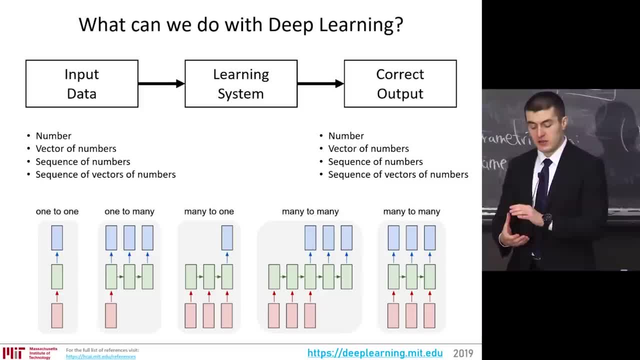 of the particular data set, and the output doesn't have to be a particular sample of the ground truth data set. It can be a sequence, sequence to sequence, a single sample to a sequence, a sequence to a sample, and so on. 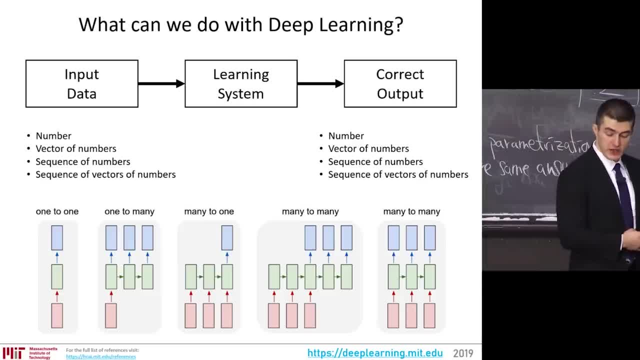 from video captioning, where it's video captioning, to translation, to natural language generation, to, of course, the one-to-one general computer vision. Okay, that's the bigger picture. Let's step back from the big to the small, to a single neuron. 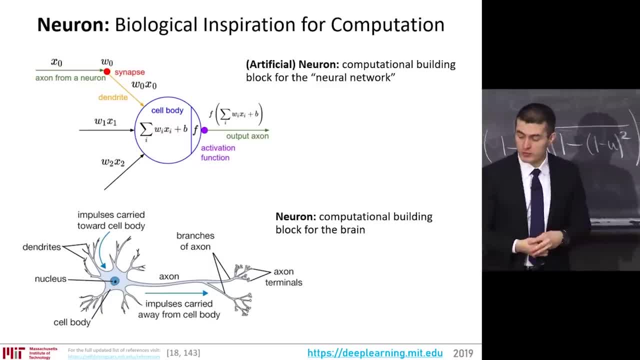 inspired by our own brain, the biological neural networks in our brain and the computational block that is behind a lot of the intelligence in our mind. The artificial neuron has inputs with weights on them, plus a bias and a number of inputs with weights on them. 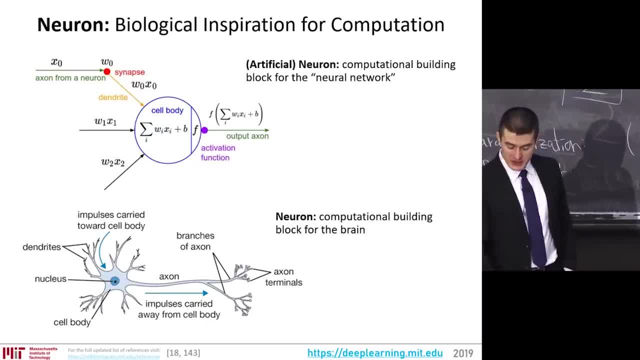 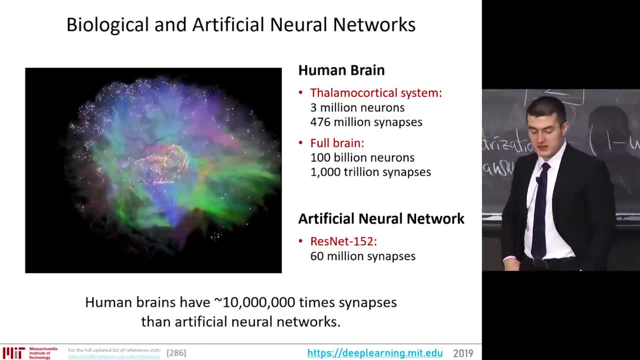 plus a bias plus a bias and an activation function and an output. It's inspired by this thing, As I showed it before here: visualizes the thalamocortical system with three million neurons and 476 million synapses. 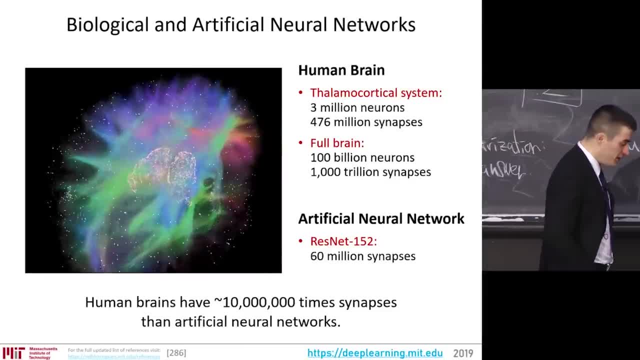 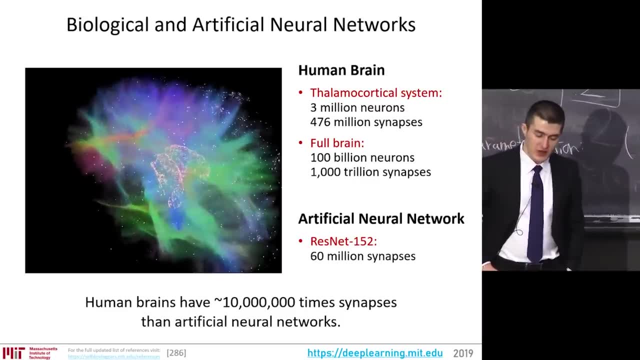 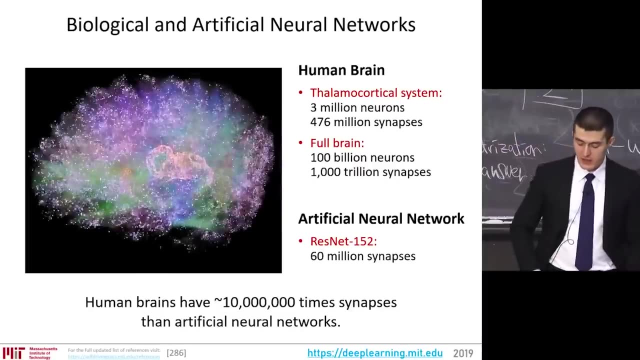 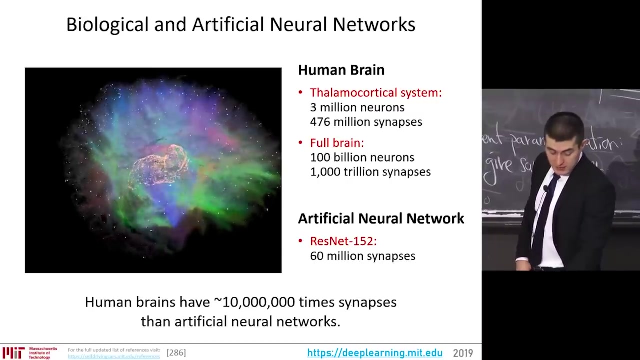 The full brain has a hundred billion billion neurons and a thousand trillion synapses. ResNet and some of the other state-of-the-art networks have in the tens, hundreds and hundreds of millions of edges of synapses. The human brain has 10 million times more synapses. 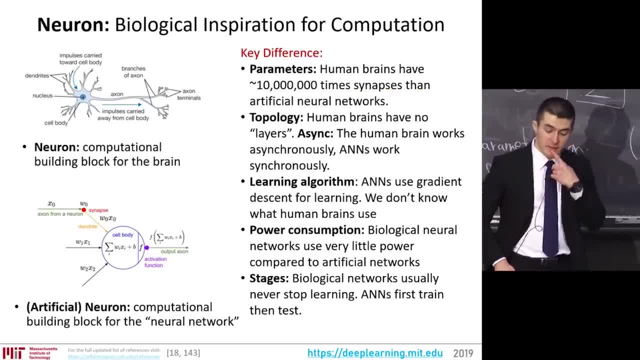 than artificial neural networks, and there's other differences. The topology is asynchronous and not constructed in layers. The learning algorithm for artificial neural networks is back propagation. What can we do for our biological networks if we don't know? That's one of the mysteries. 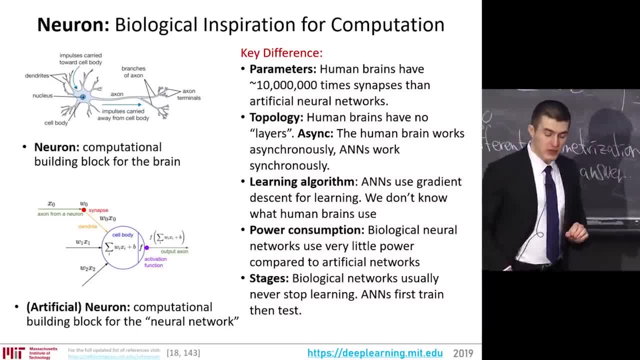 of the human brain. There's ideas, but we really don't know The power consumption of human brains are much more efficient than neural networks. That's one of the problems that we're trying to solve, and ASICs are starting to begin to solve. 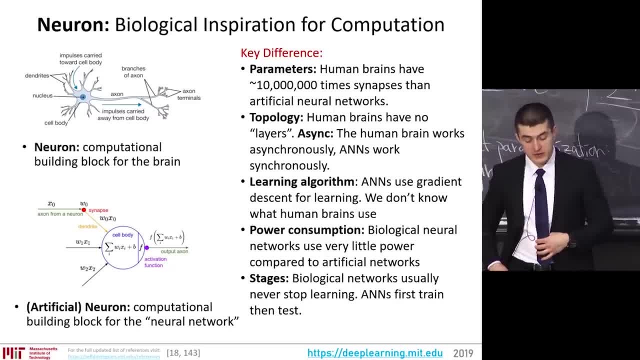 some of these problems And the stages of learning in the biological neural networks. you really never stop learning. You're always learning, always changing, both in the hardware and the software. You're developing a whole ever-changing neural network that can generate. 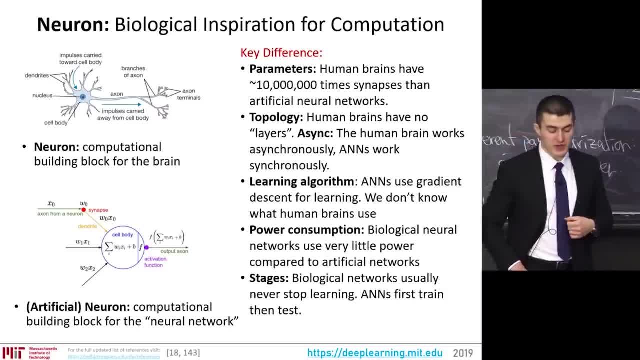 in artificial neural networks. often times there's a training stage, there's a distinct training stage and there's a distinct testing stage when you release the thing in the wild. online learning is an exceptionally difficult thing that we're still in the very early stages of this neuron. 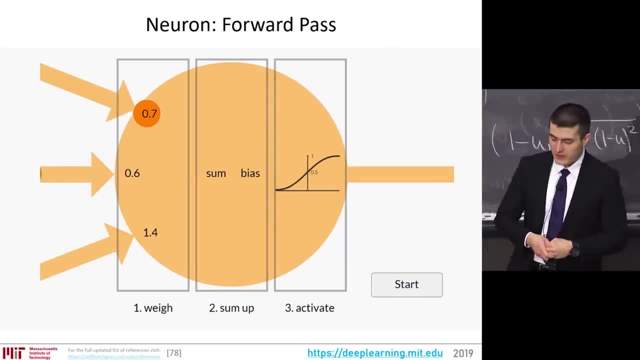 takes a few inputs- the fundamental computational block behind neural networks- takes a few inputs, applies weights, which are the parameters that are learned, sums them up, puts it into a non-linear activation function after adding the bias, also a learned parameter, and gives an output and the task of this neuron. 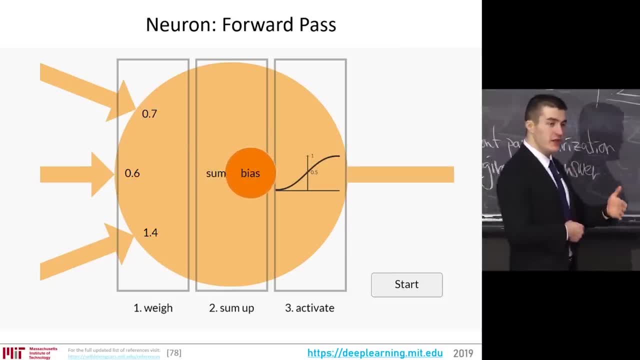 is to get excited based on certain aspects of the layers, features, inputs that followed before, and, in that ability to discriminate, get excited by certain things and get not excited by other things, hold a little piece of information of whatever level of abstraction it is. so when you combine many of them together, 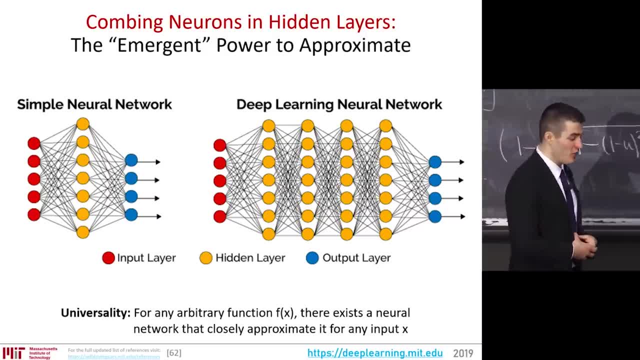 you have knowledge- different levels of abstractions form a knowledge base that's able to represent, understand or even act on a particular set of raw inputs, and you stack these neurons together in layers both in width and depth, increasing further on, and there's a lot of different. 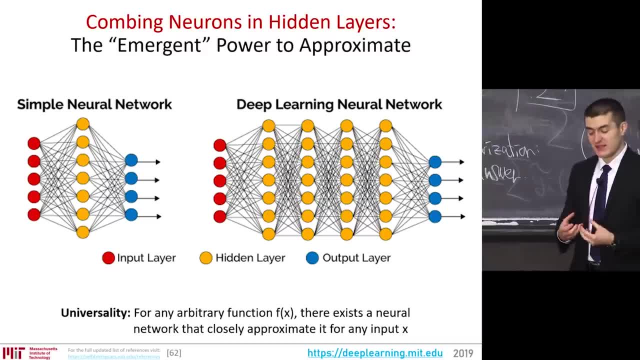 architectural variants, but they begin at this basic fact that with just a single hidden layer of a neural network, the possibilities are endless. it can approximate any arbitrary function. adding a neural network with a single hidden layer can approximate any function. that means any other neural network with multiple layers, and so on. 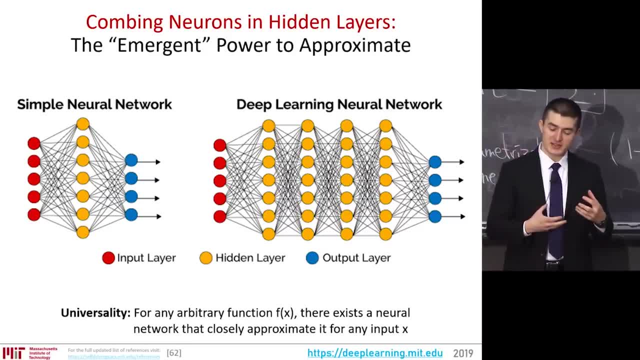 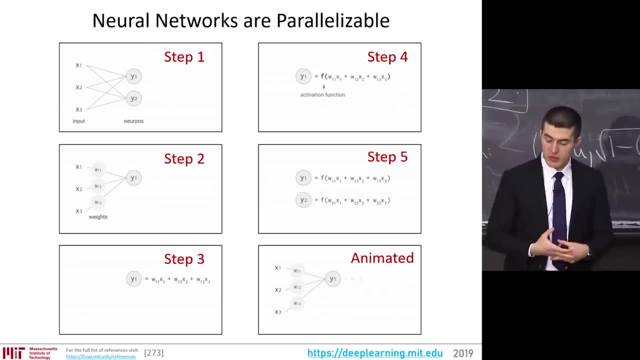 is just interesting optimizations of how we can discover those functions. the possibilities are endless. and the other aspect here is the mathematical underpinnings of neural networks with the weights and the differentiable activation. functions are such that in a few steps from the inputs to the outputs 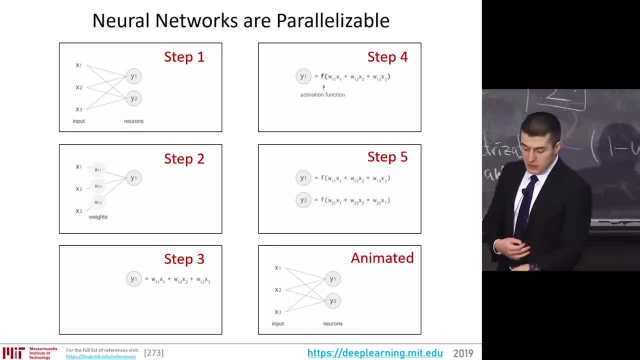 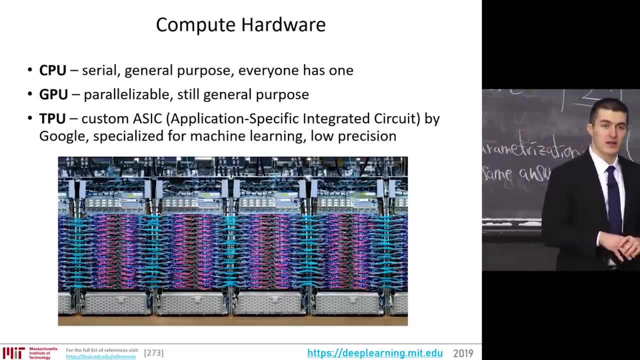 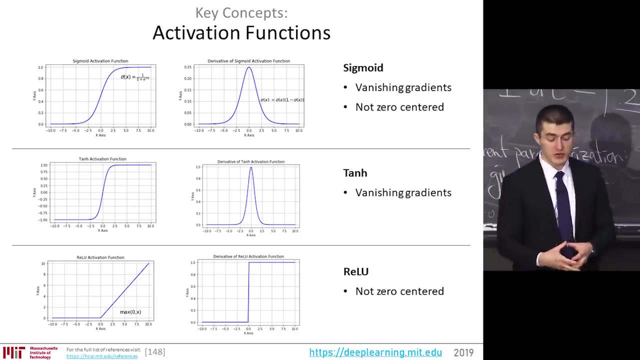 are deeply parallelizable and that's why the other aspect on the compute, the parallelizability of neural networks, is what enables some of the exciting advancements on the graphical processing unit, the GPUs, and with ASICs, TPUs, the ability to run across across machines, across GPU units. 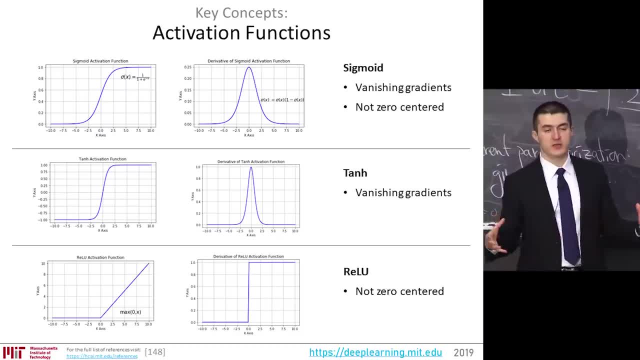 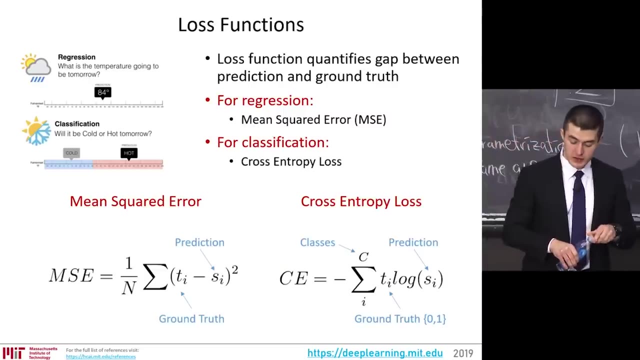 in the at a very large distributive scale, to be able to train and perform inference on neural networks. activation functions: these activation functions put together are tasked with optimizing the neural network. to be able to train and perform inference on neural networks utilizing a loss function for regression. 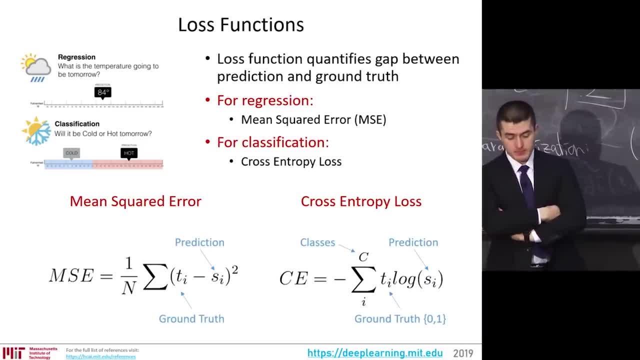 that loss function is mean squared error. usually there's a lot of variance and for classifications, cross-entropy loss. in the cross-entropy loss the ground truth is zero one in the mean squared error it's: it's a real number and so with the loss function, 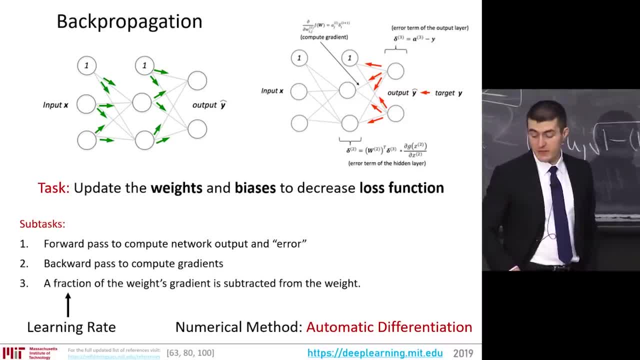 and the weights and the bias and the activation functions propagating forward through the network from the input to the output. Using the loss function, we use the algorithm of backpropagation. I wish I did an entire lecture last time to adjust the weights. 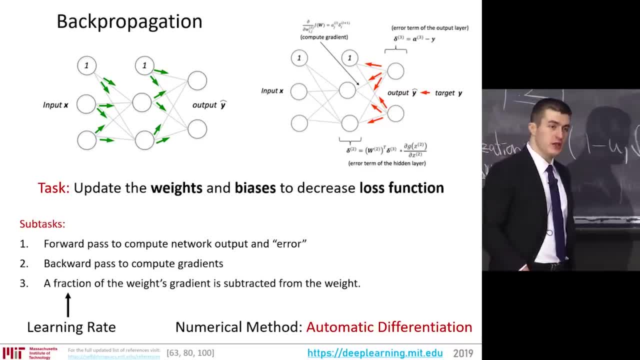 to have the air flow backwards to the network and adjust the weights such that, once again, the weights that were responsible for producing the correct output are increased and the weights that were responsible for producing the incorrect output were decreased. The forward pass gives you the error. 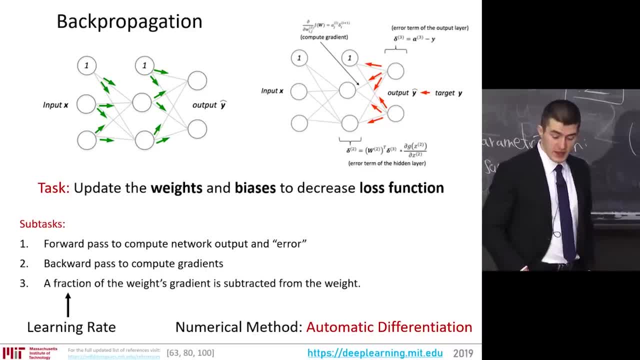 the backward pass computes the gradients and, based on the gradients, the optimization algorithm, combined with the learning rate, adjust the weights. The learning rate is how fast the network learns, And all of this is possible on the numerical computation side with automatic differentiation. 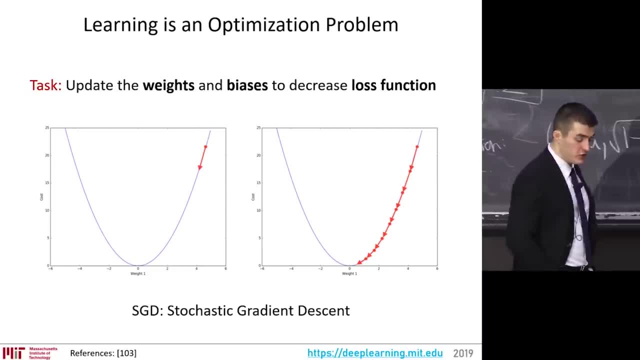 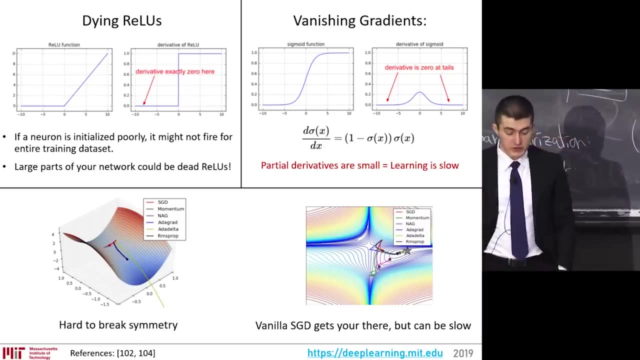 The optimization problem, given those gradients that are computed on the backward flow to the network of the gradients, is stochastic gradient descent. There's a lot of variance in this optimization algorithms that solve various problems, from dying values to vanishing gradients. There's a lot of different parameters on momentum and so on. 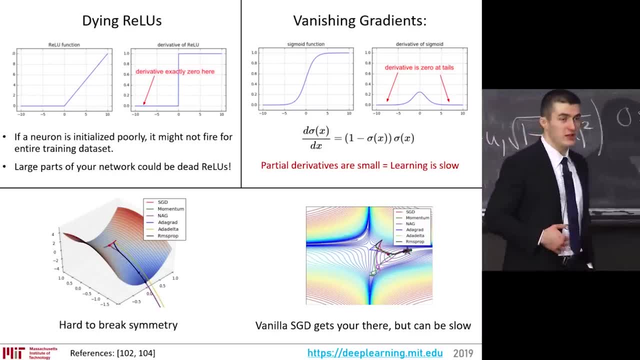 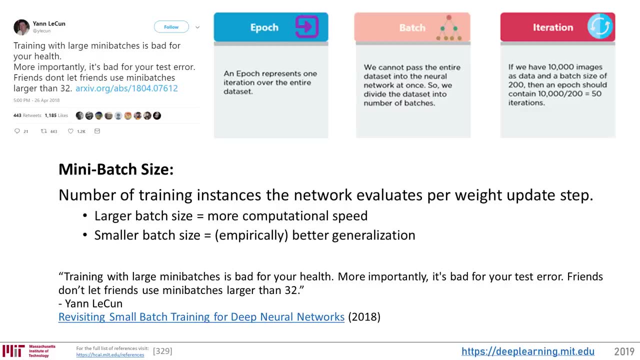 that really just boil down to all the different problems that are solved with nonlinear optimization. Mini-batch size: what is the right size of a batch- or really it's called mini-batch when it's not the entire data set based on which to compute the gradients. 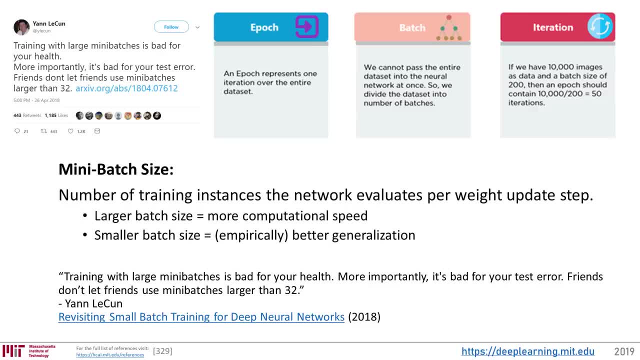 to adjust the learning? Do you do it over a very large amount or do you do it with stochastic gradient descent for every single sample of the data? If you listen to Yann LeCun and a lot of recent literature, it's small. 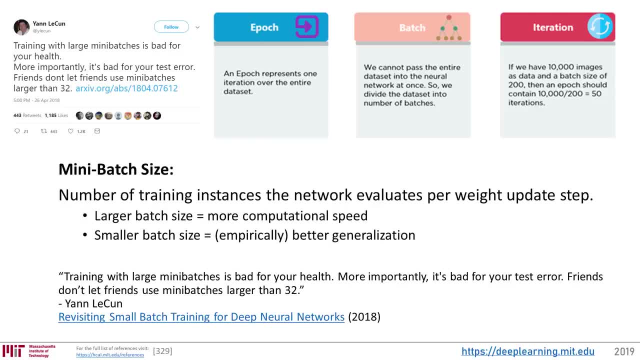 mini-batch sizes are good. He says training with large mini-batches is bad for your health. More importantly, it's bad for your test error. Friends, don't let friends use mini-batches larger than 32.. Larger batch size means more computational speed. 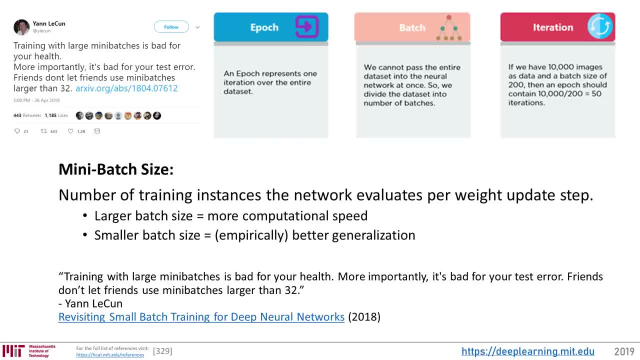 because you don't have to update the weights as often. but smaller batch size empirically produces better generalization. The problem we're often faced with is is that we don't have enough data. We don't have enough data. The problem we're often faced with is: 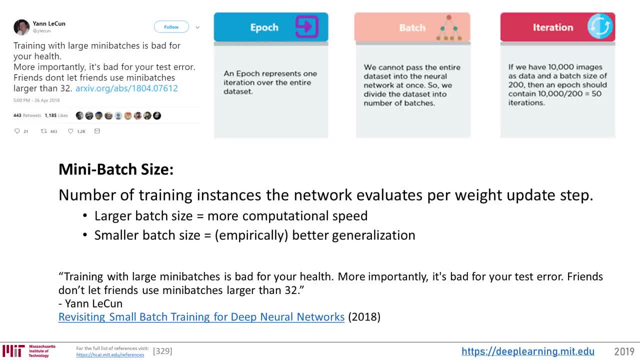 is that we don't have enough data. The problem we're often faced with is is that we don't have enough data. The problem we're often faced with is, on the broader scale of learning. trying to solve is overfitting. 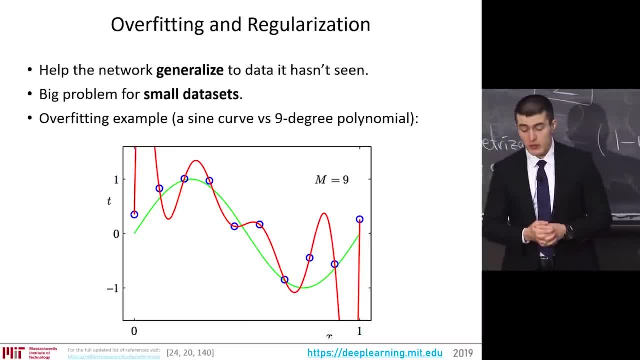 And the way we solve it is through regularization. We want to train on a data set without memorizing, to an extent that you only do well in that trained data set. So you want it to be generalizable into future, into the future things that you haven't seen yet. 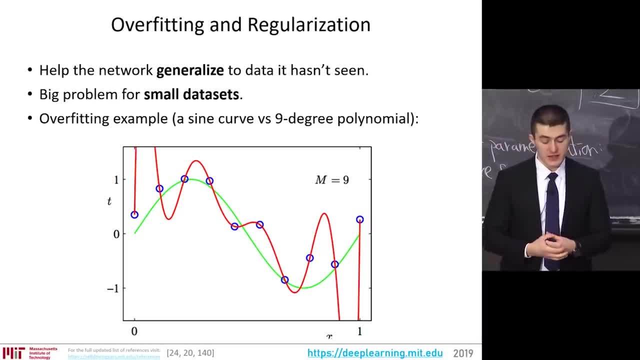 So obviously this is a problem for for small data sets and also for sets of parameters that you choose Here, shown an example of a sine curve trying to fit a particular data versus a ninth degree polynomial trying to fit a particular set of data with the blue dots: 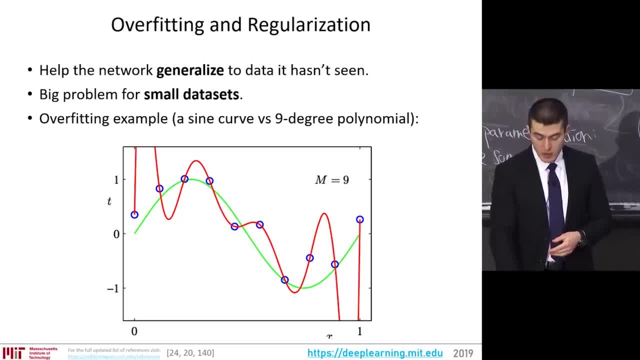 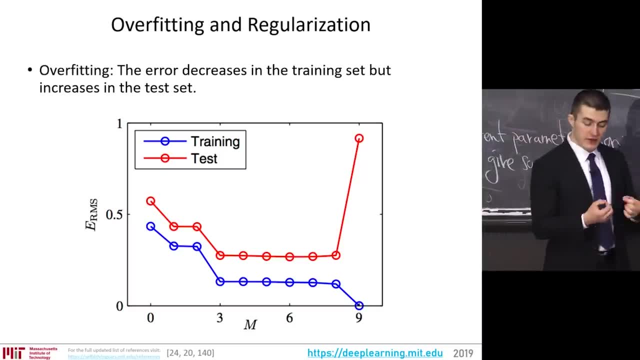 The ninth degree polynomial is overfitting. It does very well for that particular set of samples but does not generalize well in the general case. And the trade off here is: as you train further and further, you're going to be able to do a lot better at the test set. 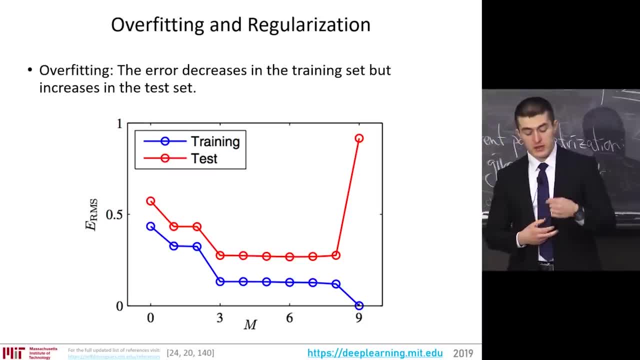 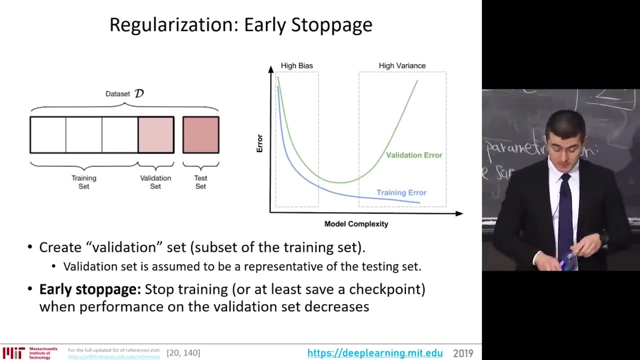 At a certain point there's a deviation between the error being decreased to zero on the training set and going to one on the test set, And that's the balance we have to strike. That's done with the validation set. So you take a piece of the training set. 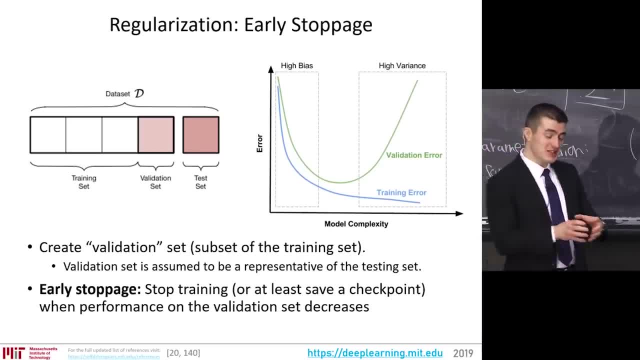 for which you have the ground truth, and you call it the validation set and you set it aside and you evaluate the performance your system on that validation set And after you notice that your train network is performing poorly on the validation set for a prolonged period of time, that's when you stop. 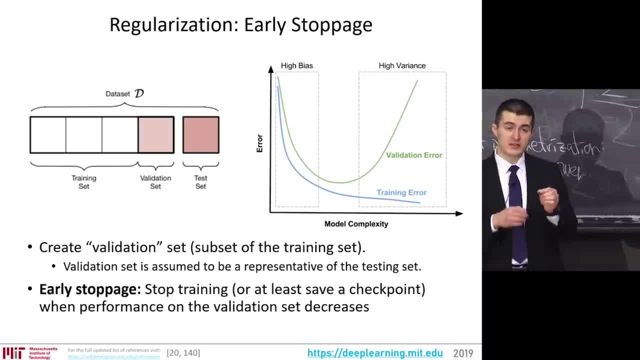 That's early stoppage. Basically, it's getting better and better and better, and then there's some period of time there's always noise, of course, and after some period of time it's definitely getting worse, And that's we need to stop there. 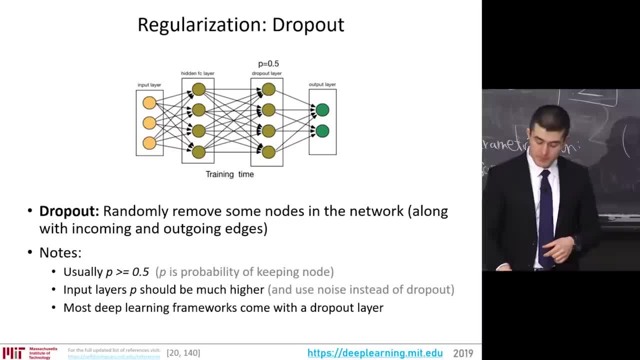 So that provides an automated way to discovering when you need to stop, And there's a lot of things that you can do. There's a lot of other regularization methodologies, Of course. as I mentioned, dropout is a very interesting approach for, and it's variants of simply. 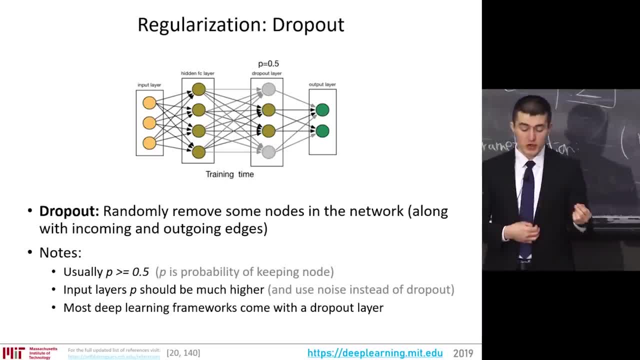 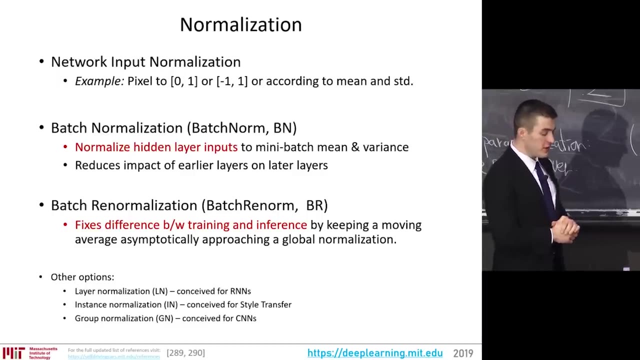 with a certain kind of probability, randomly remove nodes in the network, both the incoming and outgoing edges, randomly throughout the training process, And there's normalization, And normalization is obviously always applied at the input. So whenever you have a data set, 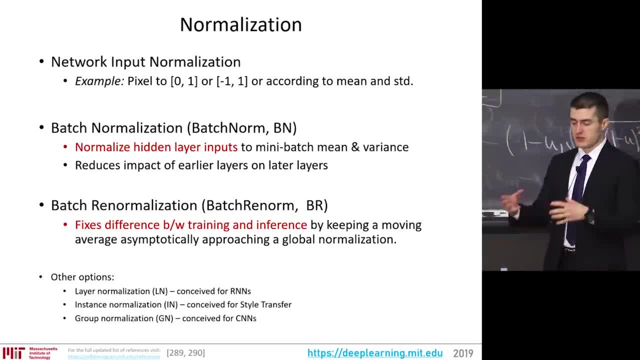 it has different lighting conditions, different variations, different sources and so on. you have to all kind of put it on the same level ground so that we're learning the fundamental aspects of the input data as opposed to some less relevant semantic information like lighting variation and so on. 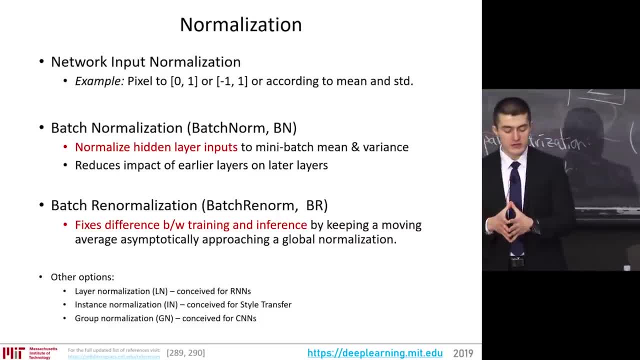 So we usually always normalize. for example, if it's computer vision with pixels from zero to 255, you always normalize to zero to one, or negative one to one, or normalize based on the mean and the standard deviation. That's something you should almost always do. 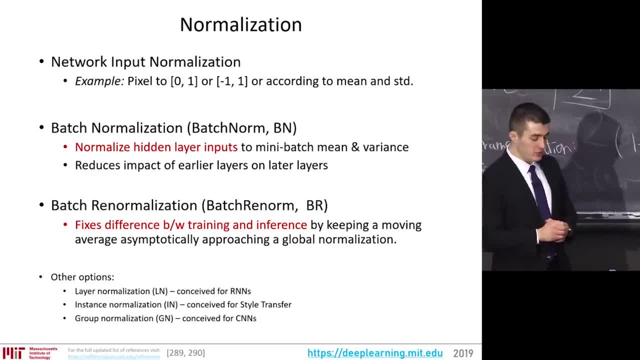 The thing that enabled a lot of breakthrough performances in the past few years is batch normalization. It's performing this kind of same normalization later on in the network, looking at the inputs to the, the hidden layers, and normalizing based on the batch of data which which you're training. 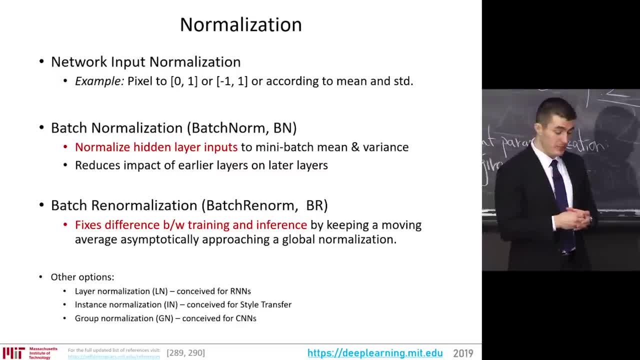 normalized based on the mean and the standard deviation as batch normalization with batch renormalization fixes a few of the challenges which is given that you're normalizing during the training on the media batch in the training data set that doesn't directly map to the inference. 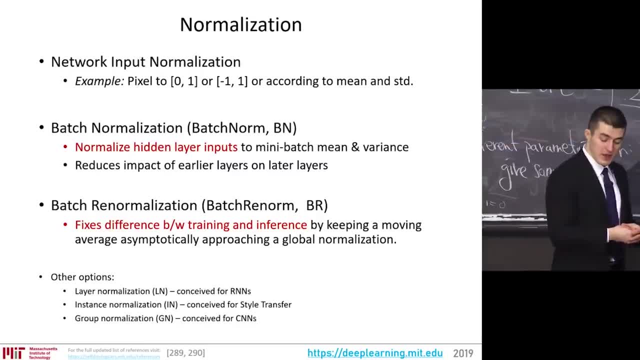 stage and the testing, and so it allows- by keeping a running average it across both training and testing- you're able to asymptotically approach a global normalization. so there's this idea across all the weights, not just the inputs, across all the weights, you normalize this. the normalize the. 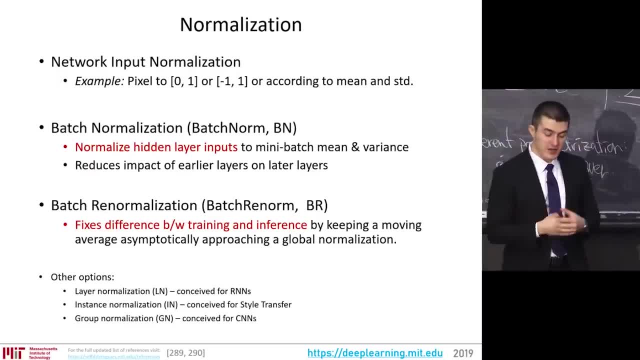 world in the all the levels of abstractions that you're forming, and batch renorm solves a lot of these problems during inference, and there's a lot of other ideas, from layers to weight, to instance normalization, to group normalization, and you can play with a lot of. 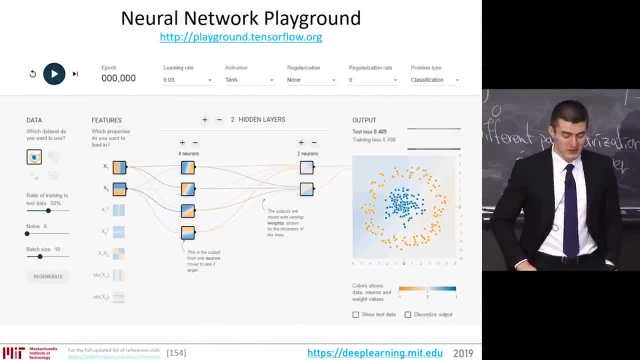 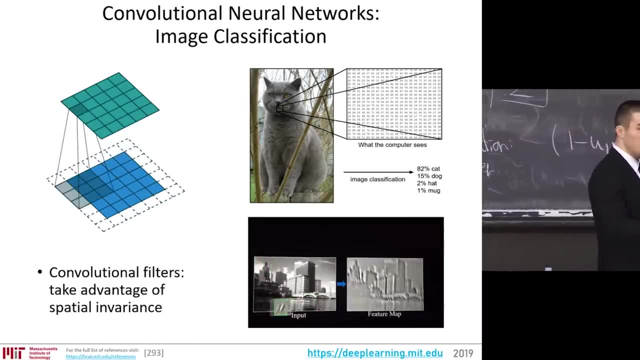 these ideas in the TensorFlow playground on playgroundtensorfloworg that I highly recommend. so now let's run through a bunch of different ideas, some of which we'll cover in future lectures of what is all of this in this world of deep learning, from computer vision to deep reinforcement. 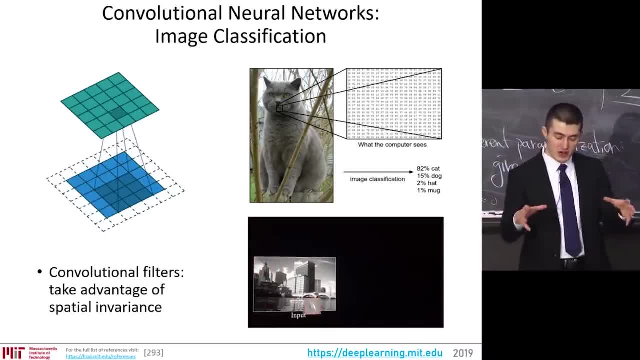 learning, to the different small level techniques, to the large natural language processing. so let's start with convolutional neural networks, the thing that enables image classification. so these convolutional filters slide over the image and are able to take advantage of the spatial invariance of visual information: that a cat in the top left corner is the same as features associated. 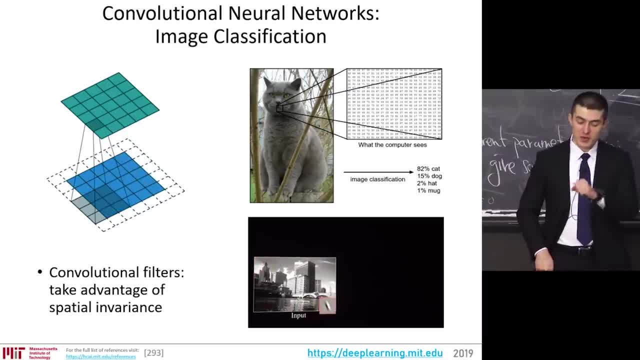 with cats in the top right corner and so on. images are just a set of numbers and our task is to take that image and produce a classification and use the spatial in the, the spatial variance of visual information, to make that, to slide a convolution filter across the image and learn that filter as opposed to. as opposed to. 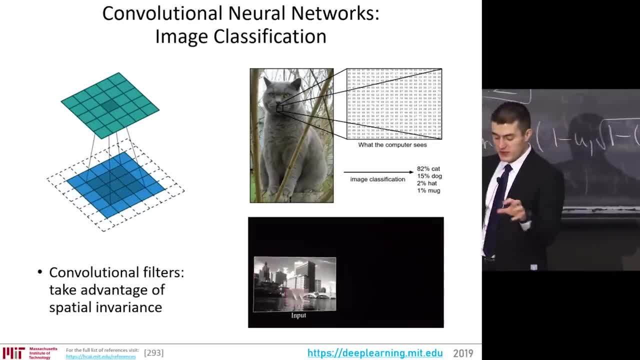 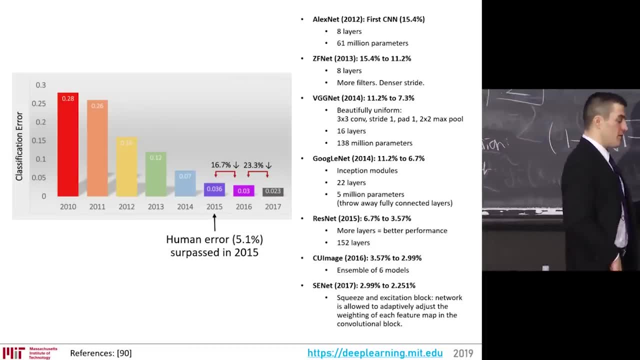 assigning equal value to features that are present in various various regions of the image and stacked on top of each other. these convolution filters can form high-level abstractions of visual information and images with Alex net, as I've mentioned, on an image net data set and challenge: captivating the. 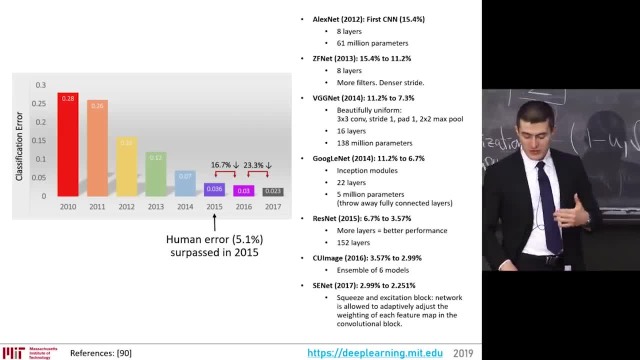 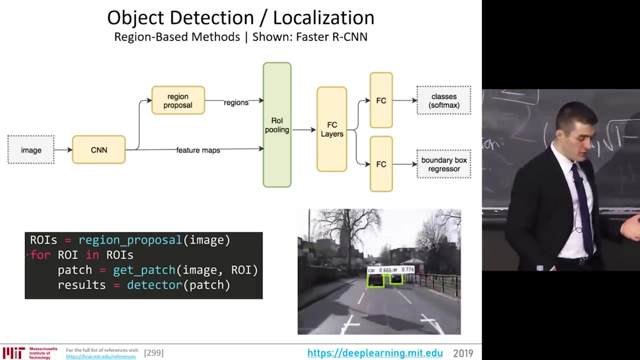 world of what is possible with neural networks have been further and further improved, superseding human, human performance, with, of special note, Google net with the inception module. there's different ideas that came along, res net with the residual blocks and SC net and most recently so the object detection problem is a step, the next step in the visual recognition, so the image class. 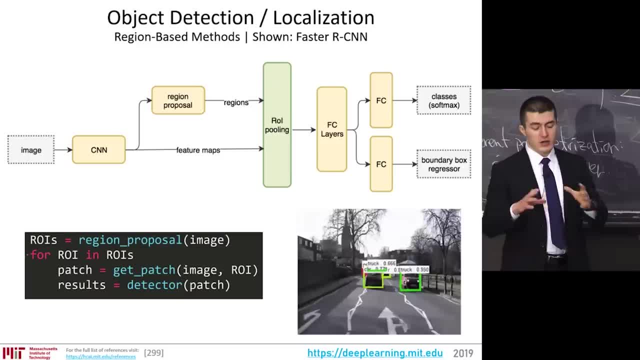 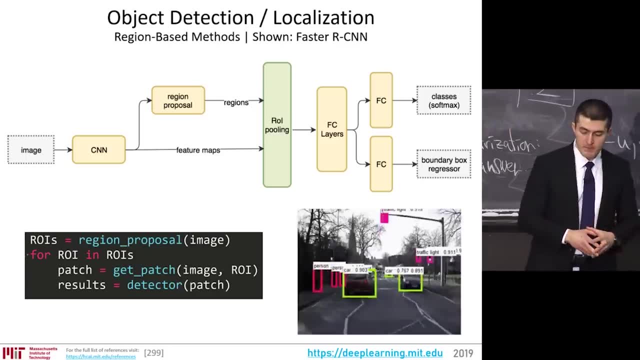 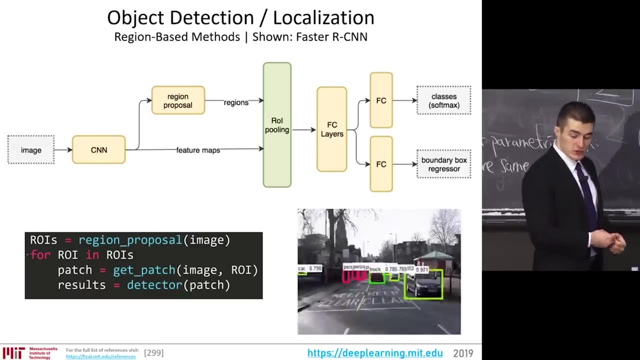 cation is just taking the entire image, is saying what's in the image? object detection localization is saying: find all the objects of interest in the scene and classify them. the region-based methods, like shown here, fast our CNN takes the image- uses convolution neural network to extract features in 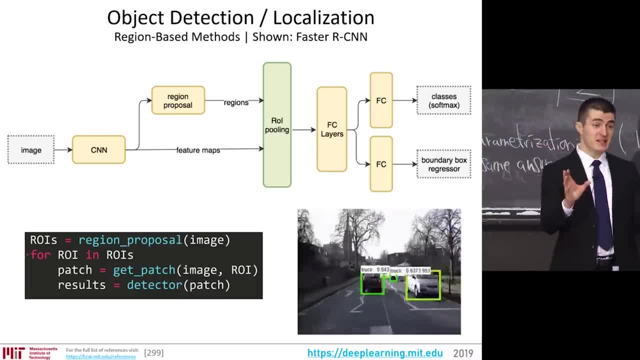 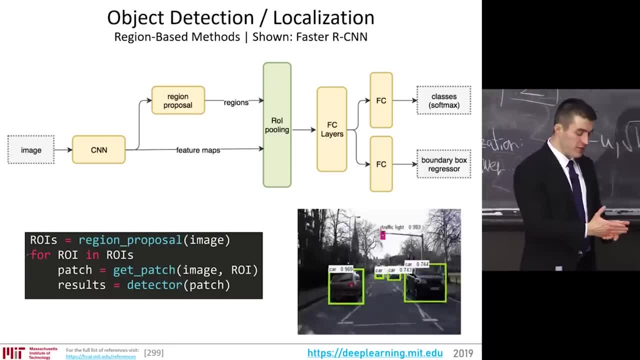 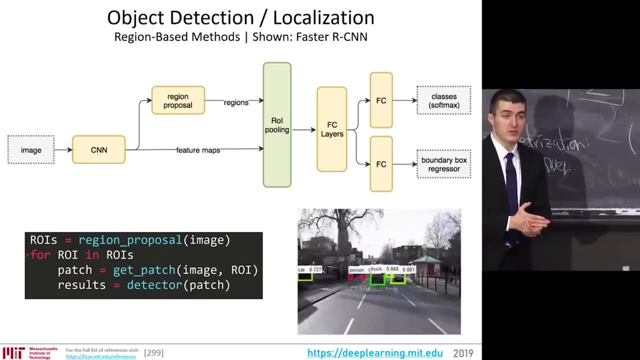 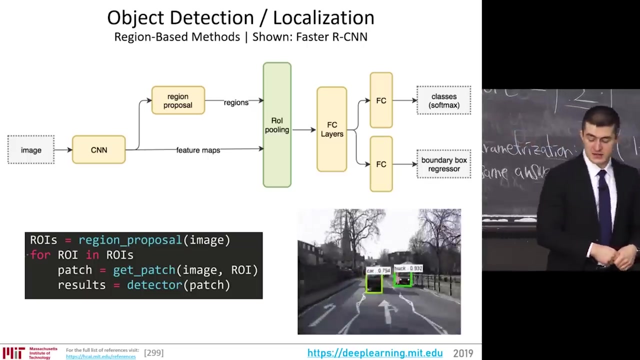 that image and generate region proposals. here's a bunch of candidates that you should look at and within those candidates it classifies what they are and generates a four parameters: the boundary box, that the, that's that thing that captures that thing. so object detection, localization ultimately boils down to a bounding box, a rectangle, with a class that's the most likely class. that's in that. 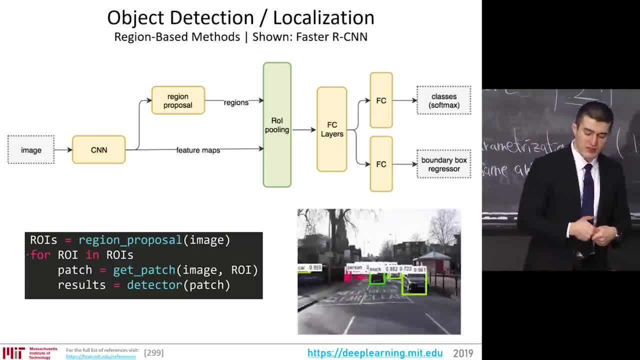 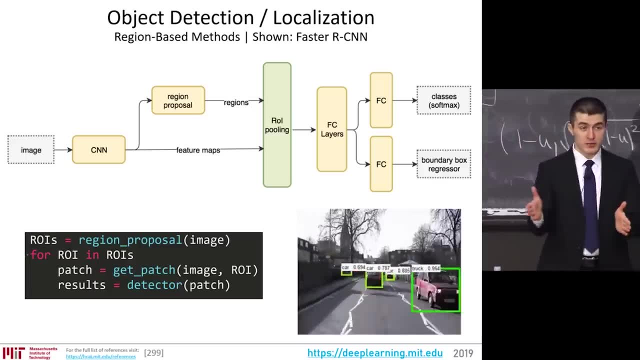 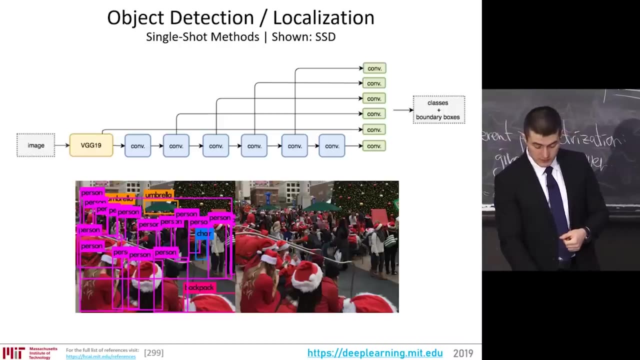 body box and you can really summarize region-based methods as you generate the region proposal- here a little pseudocode- and do a for loop over the over the region proposals and perform a detection on the on that for loop. the single shop methods. remove the for loop. there's a single pass. 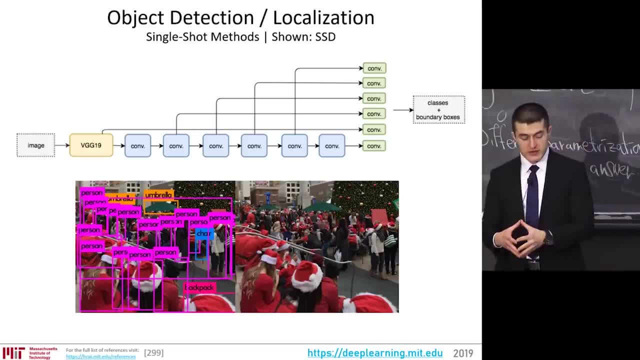 through you add a bunch of. take a, for example, here shown SSD. take a pre-trained neural network that's been trained to do image classification. stack a bunch of convolutional layers on top. from each layer, extract features that are then able to generate in a single pass classes, the bounding 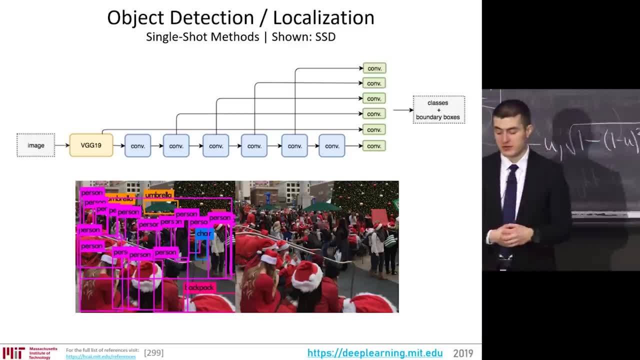 boxes, body box prediction and then generate a single pass class, that's a bounding box prediction and the class associated with those body box. the trade-off here- and this is where the popular Yolo v123 come from, the the trade-off here oftentimes is in performance and accuracy. so single shot. 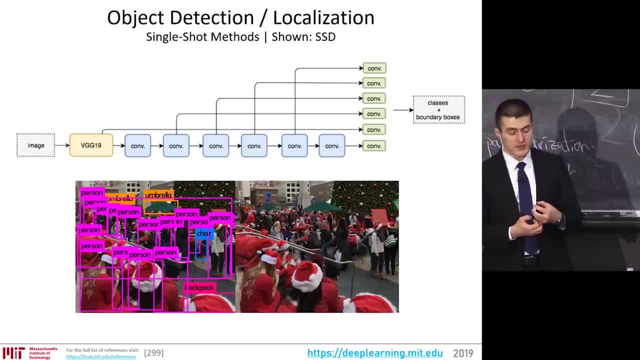 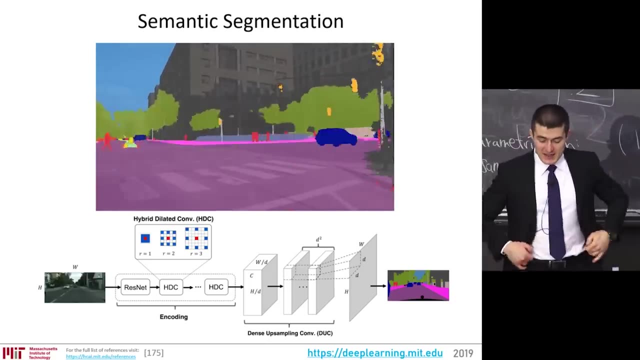 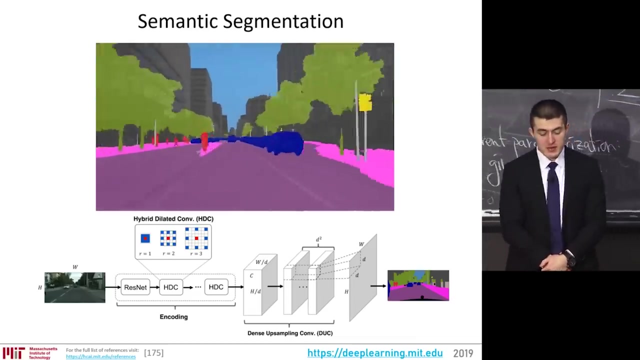 methods are are often less performant, especially on in terms of accuracy, on objects that are really far away, or rather objects that are small in the image or a really large, then the next step up in visual perception, visual understanding, is semantic segmentation. that's where the tutorial that we presented here on GitHub is covering semantic segmentation, is the task of now. 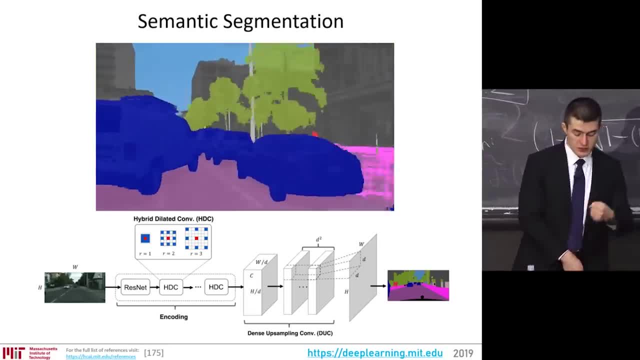 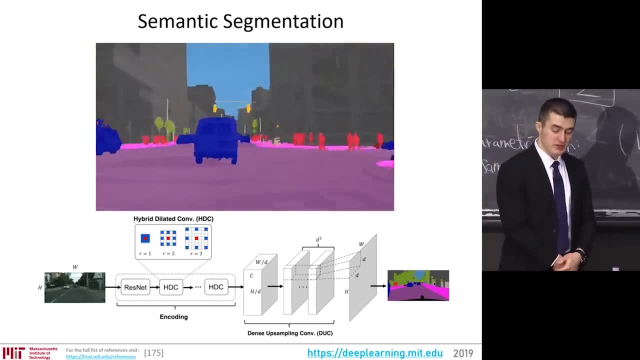 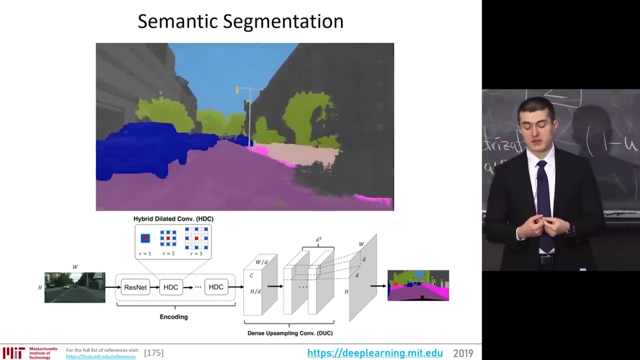 as opposed to a bounding box or to classify the entire image or detecting the objects as a body box, is assigning at a pixel level the boundaries of what the object is, every single in full scene classification, full scene segmentation, classifying what every single pixel which class that pixel belongs to and the fundamental aspect there is. 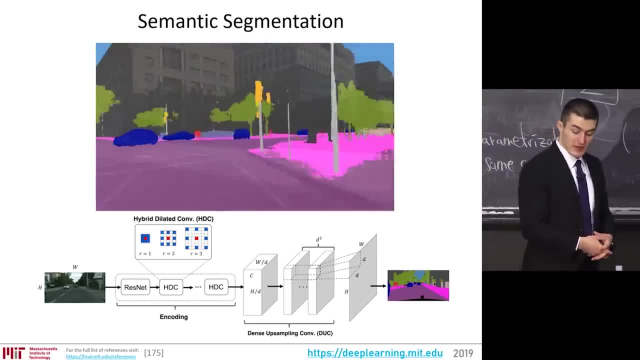 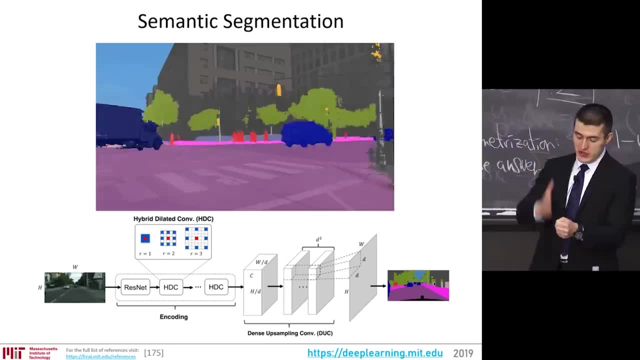 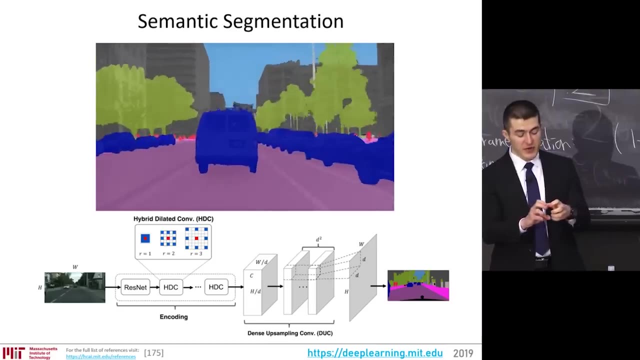 we'll cover a little bit or a lot more on Wednesday, is taking a image classification Network, chopping it off at some point and then having, which is performing the encoding step of of compressing a representation of the scene and taking that representation with a decoder up, sampling in a 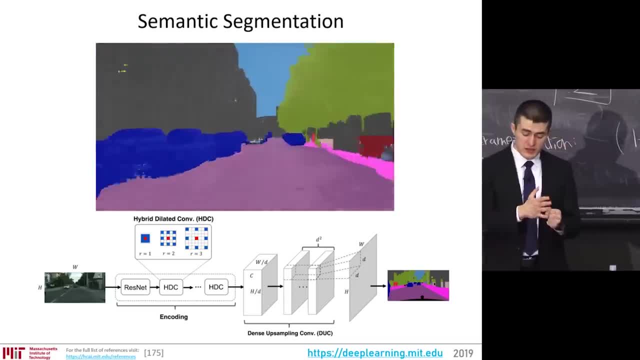 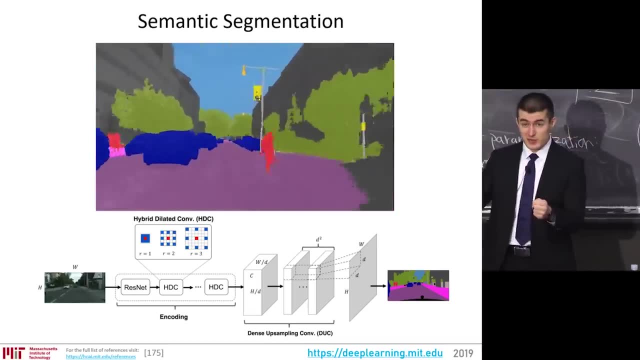 dense way, the uh. so taking that representation and up sampling the pixel level classification, so that up sampling- there's a lot of tricks that we'll talk through, that are interesting, but ultimately boils down to the encoding step of forming a representation. what's going on in the 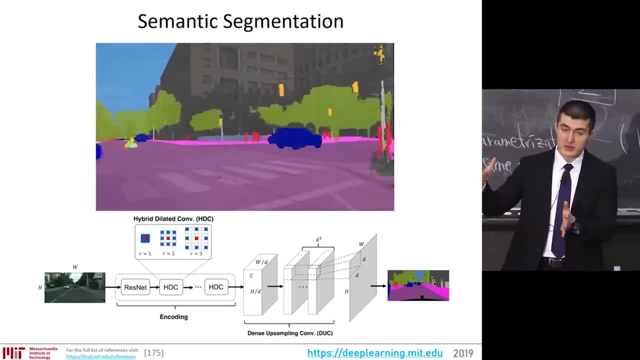 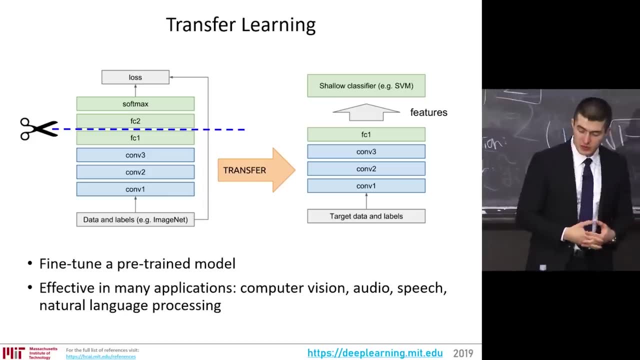 scene and then the decoding step, that up samples, the pixel level, annotation, classification of all the individual pixels and, as I mentioned here, the underlying idea applied most extensively, most successfully in computer vision, is transfer learning. most commonly applied way of transfer learning is taking a pre-trained neural network. 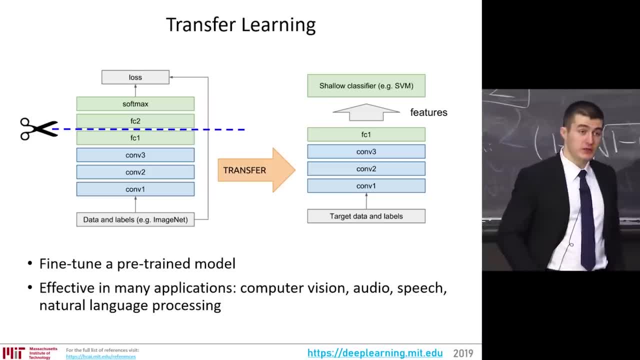 like ResNet, and chopping it off at some point. chopping off the fully connected layer layers, some aspects, some parts of the layers, and then taking a data set, that a new data set, training that Network. so what is this useful for? for every single application. computer vision in industry. 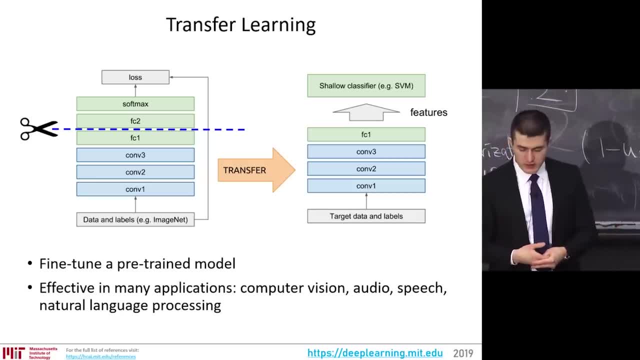 when you have a specific application, like you want to build a pedestrian detector. if you want to build a pedestrian detector and you have a pedestrian data set, it's useful to take ResNet, trained on ImageNet, or Coco, trained in the general case of vision perception, and taking that Network chopping. 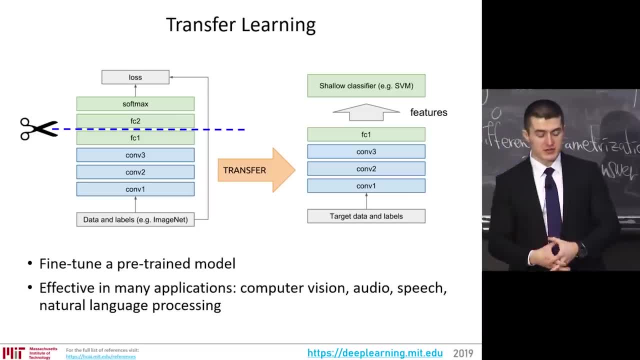 off some of the layers and then retraining on your specialized pedestrian data set and, depending on how large that data set is, the sum of the previous layers that from the pre-trained, pre-trained Network should be fixed, frozen, and sometimes not, depending on how large the data is. 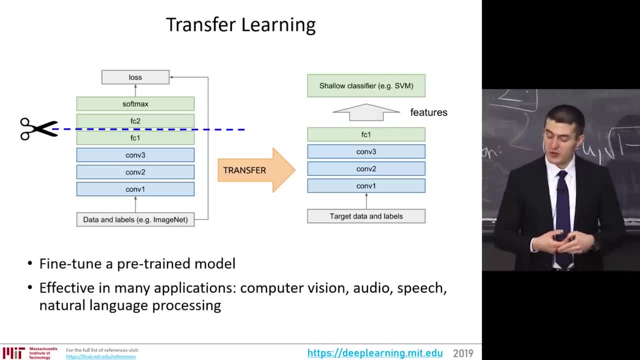 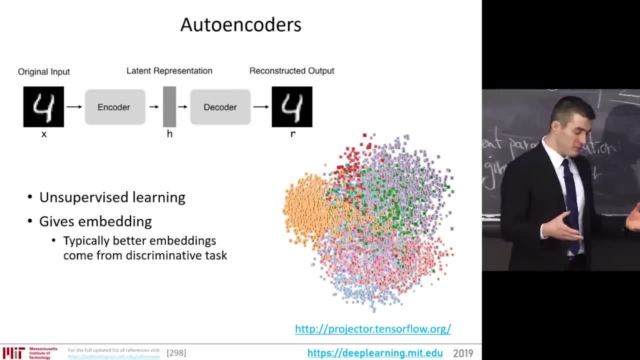 and this is extremely effective in a computer vision, but also in audio speech and NLP, and so, as I mentioned, with the pre-trained networks, they are ultimately forming representations of the data based on which classifications the regression is made, prediction is made. but a cleanest example of this is the auto encoder. 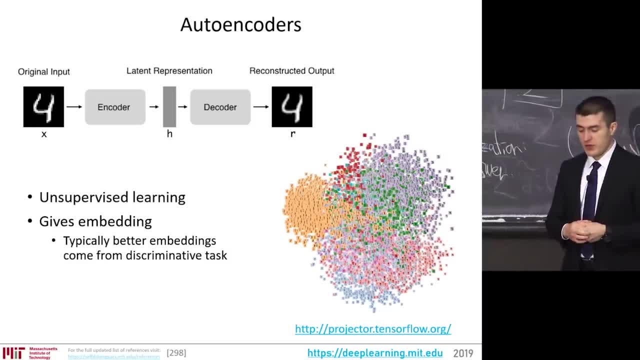 of forming representations in an unsupervised way. the output- the input- is an image and the output is that exact same image. so why do we do that? well, if you add a bottleneck in the network, where there is, where the network is narrower at the in the middle than it is on the inputs and the outputs, it's forced to compress. 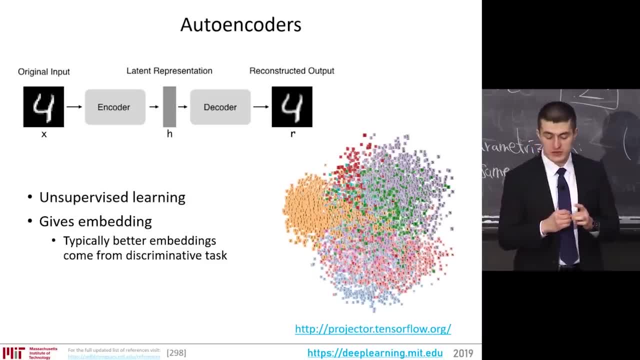 the data down into meaningful representation. that's what the auto encoder does. you're training it to reproduce the output and reproduce it with a latent representation that is smaller than the original raw data, and that's a really powerful way to compress the data it's used for. 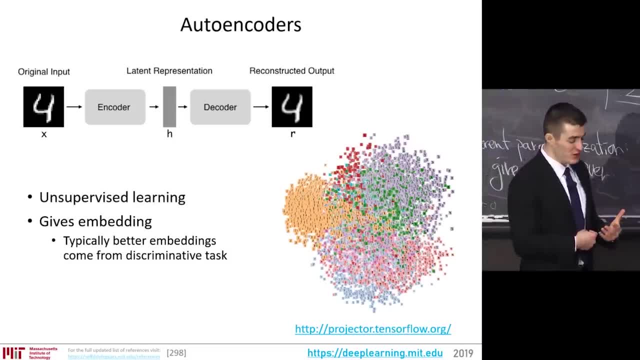 removing noise and so on, but it's also just an effective way to demonstrate a concept. it can also be used for embeddings. we have a huge amount of data and you want to uh, form a compressed, efficient representation of that data. now, in practice, this is completely unsupervised in practice. if you want to form an efficient, useful representation of the data, 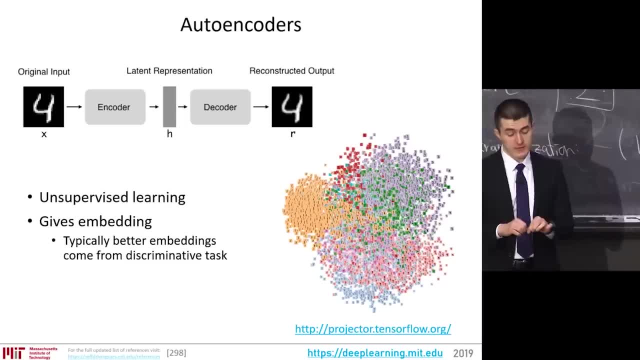 uh, you want to train it in a supervised way. you want to train it on a discriminative task where you have label data and the network is trained to identify cat versus dog. that network that's trained in a discriminative way on an annotated, supervised learning way. 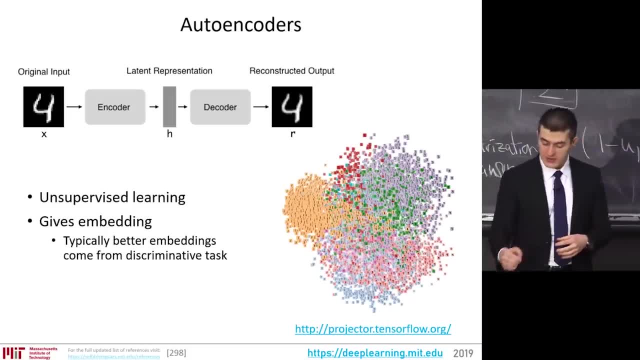 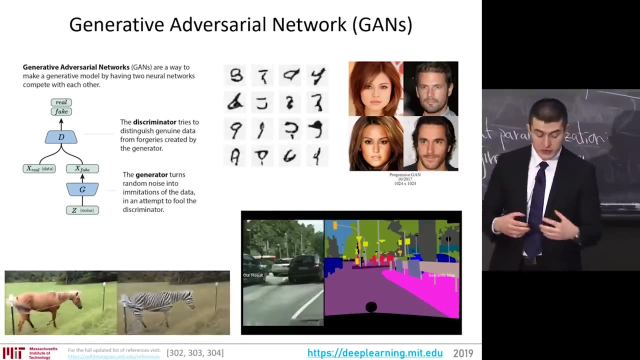 uh, is able to form better representation, but nevertheless, the concept stands, and one way to visualize these concepts is the. the tool that I really love, projectortensorfloworg, is a way to visualize these different representations, these different embeddings you should, you should definitely play with and you can insert your own data. okay, going further and further in this direction of 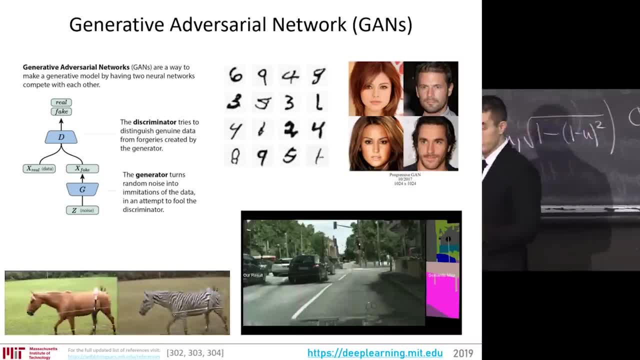 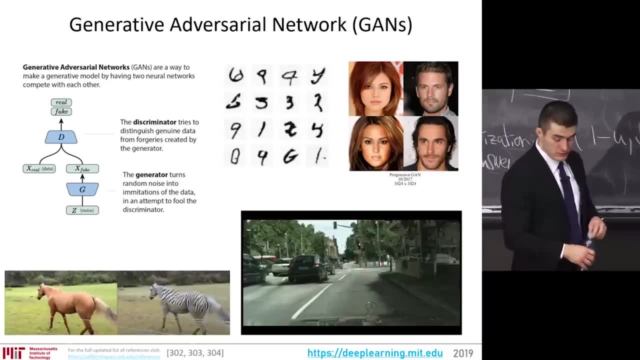 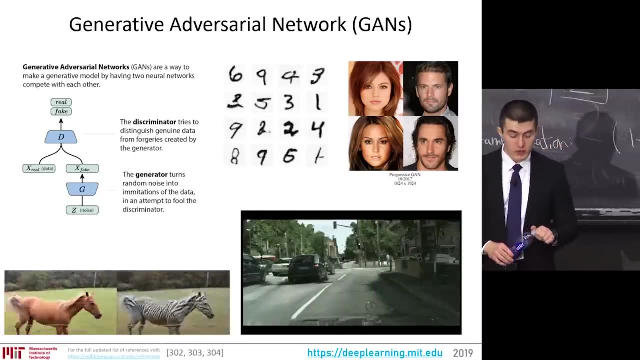 unsupervised and forming representations is generative adversarial networks, from these representations being able to generate new data. and the fundamental methodology of of Gans is to have two networks: one is the generator, one of the discriminator, and they compete against each other in order to for the generator. 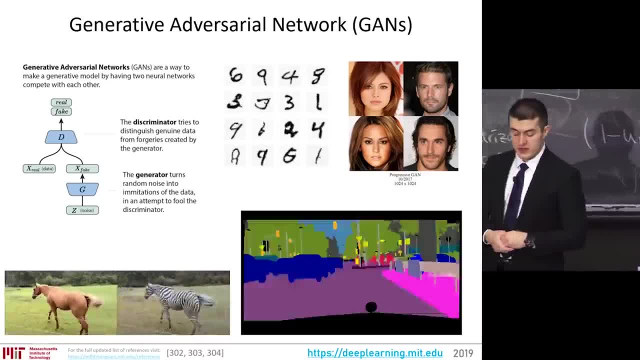 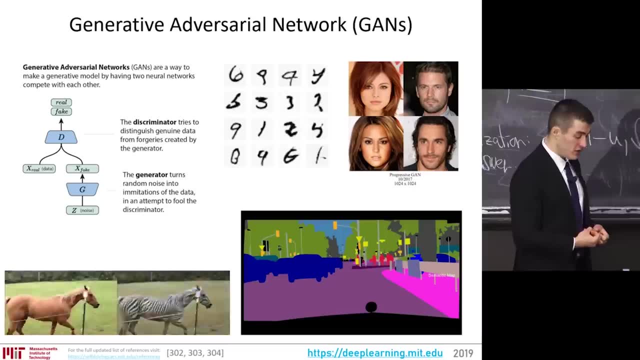 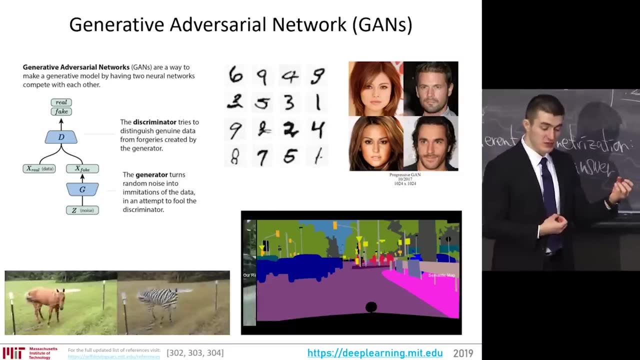 to uh get better and better and better at generating realistic images. The generator's task from noise to generate images based on a certain representation, that are realistic, and the discriminator is the critic that has to discriminate between real images and those generated by the generator. 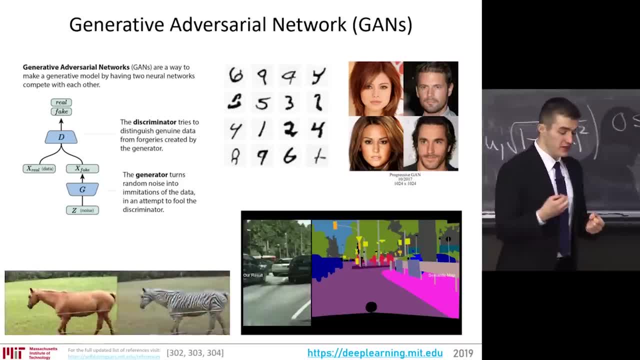 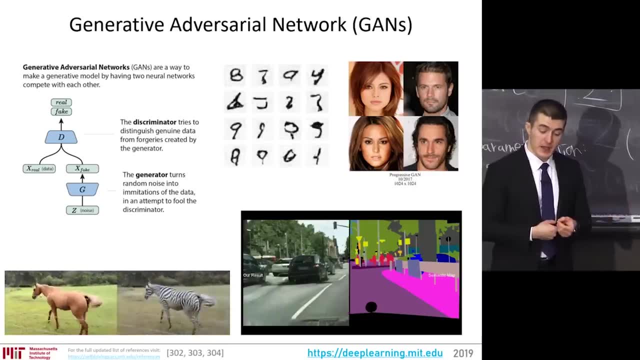 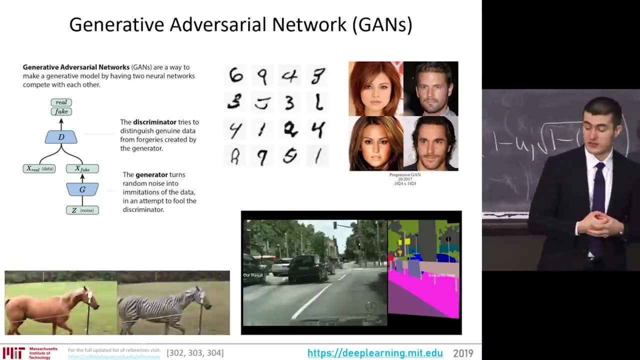 and both get better together. The generator gets better and better at generating real images to trick the discriminator, and the discriminator gets better and better at telling the difference between real and fake, until the generator is able to generate some incredible things, So shown here by the work with NVIDIA. 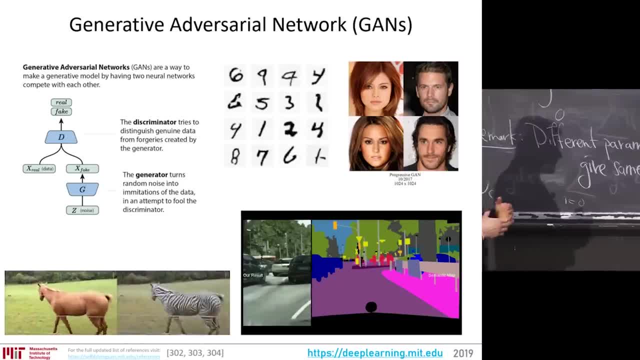 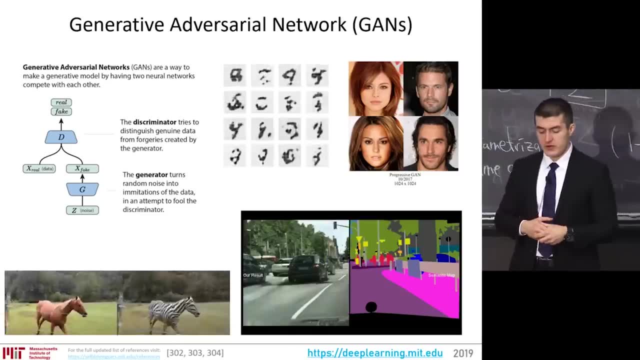 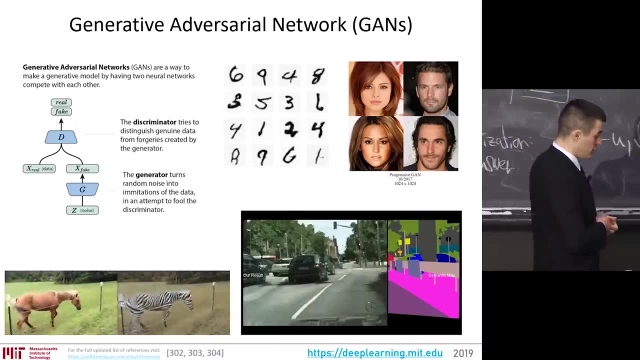 the ability to generate realistic faces has skyrocketed in the past three years, So these are samples of celebrities' photos that have been able to generate. Those are all generated by- again, there's ability to generate temporally consistent video over time with GANs. 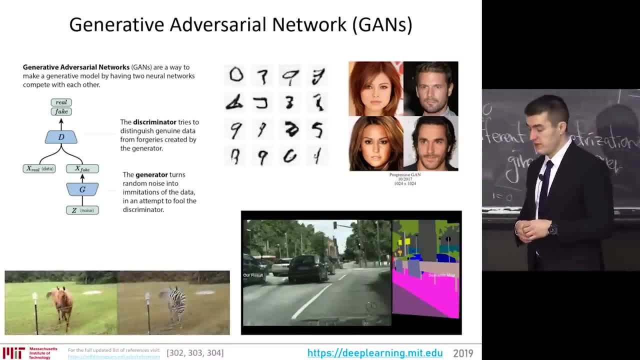 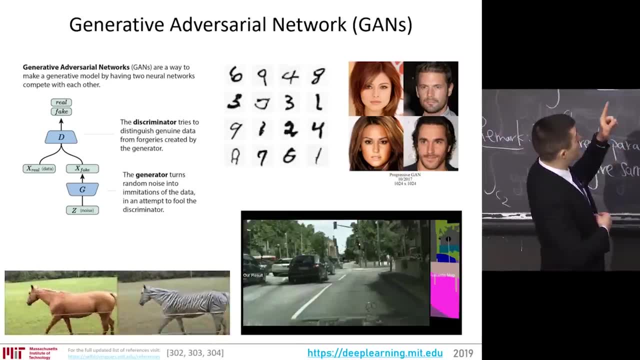 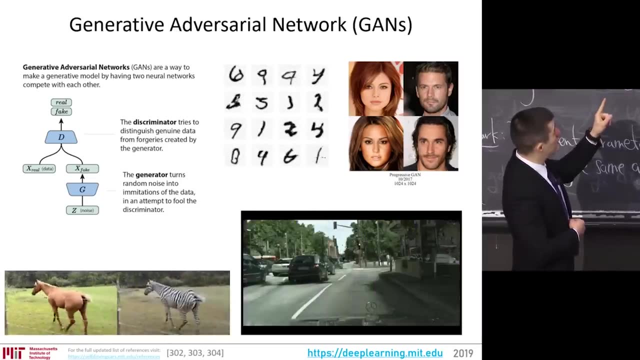 and then there's the ability shown at the bottom right in NVIDIA- I'm sure Arles will talk about- on a pixel level from semantic segmentation. so from the semantic pixel segmentation on the right, being able to generate completely the scene on the left. 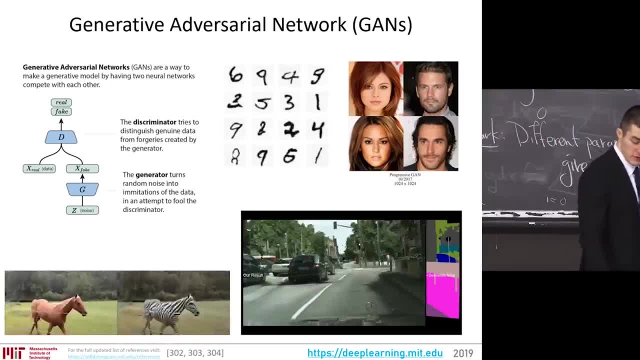 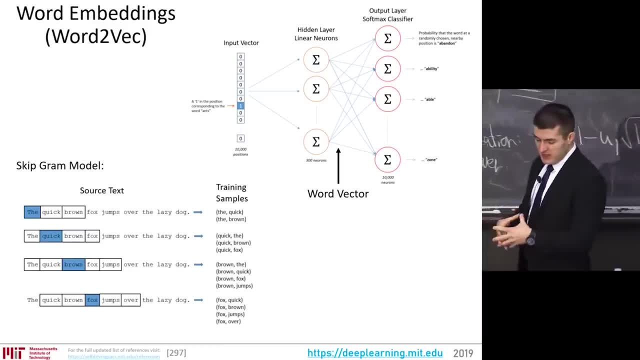 all the raw, rich, high-definition pixels on the left. The natural language processing world. same forming representations, forming embeddings with Word2Vec, the ability from words to form representation that are efficiently able to then be used to reason about the words. 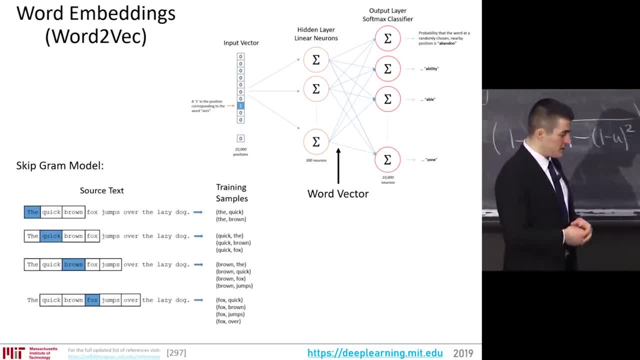 The whole idea of forming representation about the data is taking a huge vocabulary of a million words. you want to be able to map it into a space where words that are far apart from each other are in a Euclidean sense, in a Euclidean distance between words. 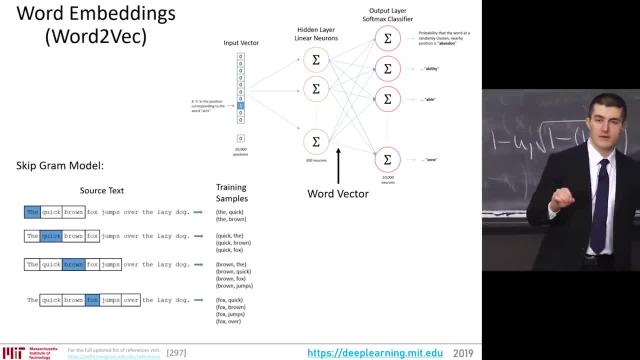 are semantically far apart from each other as well, So things that are similar are together in that space, And one way of doing that, with skip grams, for example, is looking at a source text and turning into a large body of text, into a superposition. 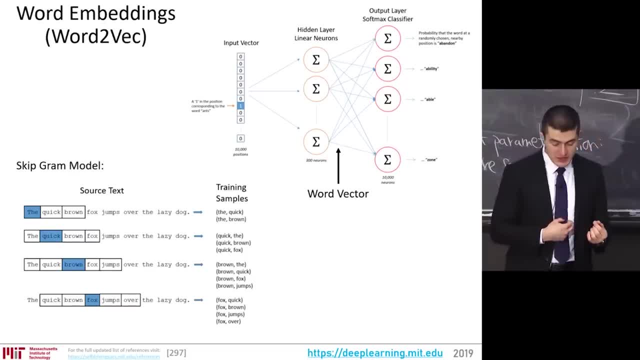 So you will get a very simple behavior where what you're doing is you're looking at various information, but you're also looking at your. Unfortunately, when you're doing your financial analysis, you're looking at the data and you're looking at a very simple analysis. 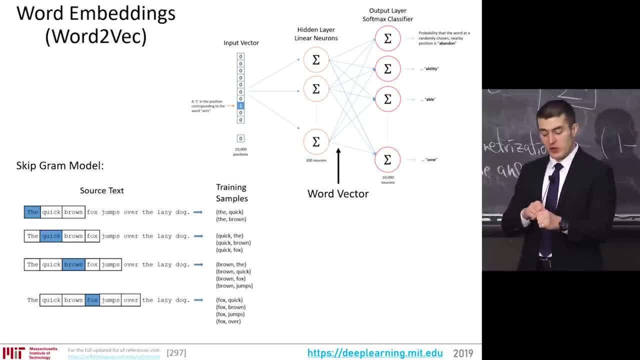 Lots of data, lots of information, lots of keys that are different than what you'd want to get if you were to have a training platform. I'm pretty sure you're gonna use a lot of data, but you're not gonna be able to predict. 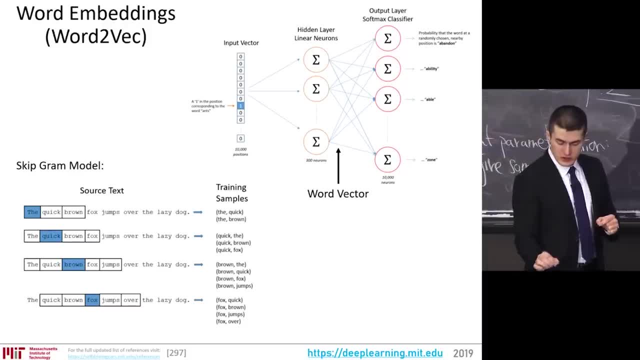 from a particular word to all its neighbors. So train a network on the connections that are commonly seen in natural language And, based on those connections, a vector representing the probability that those words are connected to each other. the main thing, both are thrown away in the end. 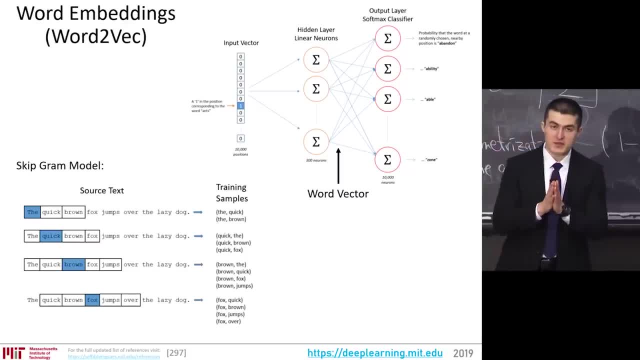 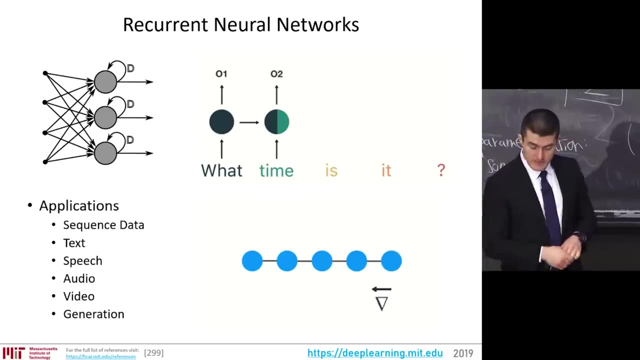 the main thing is the middle, the hidden layer. that representation gives you the embedding, that represent these words in such a way where, in the Euclidean space, the ones that are close together are semantically together and the ones that are not are semantically far apart. and 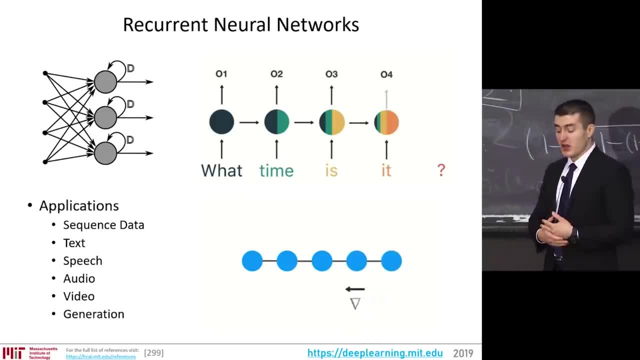 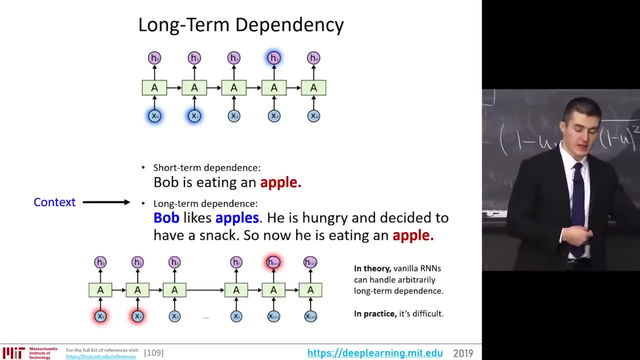 natural language and other sequence data. text, speech, audio video relies on recurrent neural networks. recurrent neural networks are able to learn temporal data, temporal dynamics in the data, sequence data and are able to generate sequence data. the challenge is that they're not able to learn. 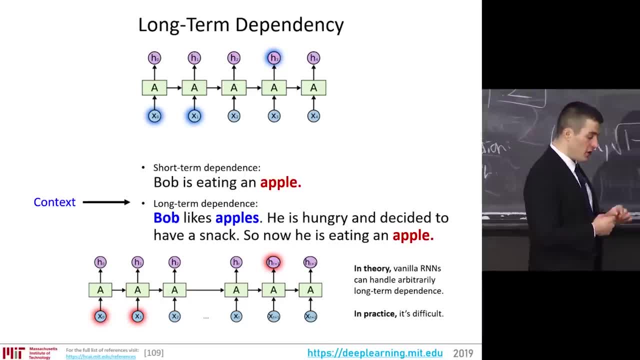 long term context because when unrolling a neural network it's trained by unrolling and doing back propagation. without any tricks, the back propagation of the gradient fades away very quickly, so you're not able to memorize the context in a longer form of the sentences unless there's extensions here. 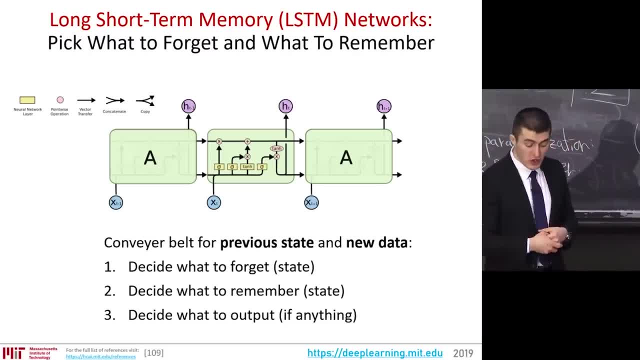 with LSTMs and GRIUs. long term dependency is captured by allowing the network to forget information, allow it to freely pass through information in time, so what to forget, what to remember and every time decide what to output. and all of those aspects have gates that are all trainable. 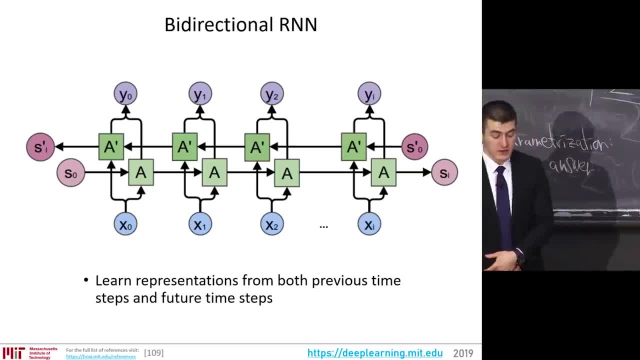 with sigmoid and 10H functions. bidirectional recurrent neural networks from the 90s is an extension often used for providing context in both directions. so recurrent neural networks simply define vanilla way is learning representations for what happened in the past. now, in many cases, you're able. 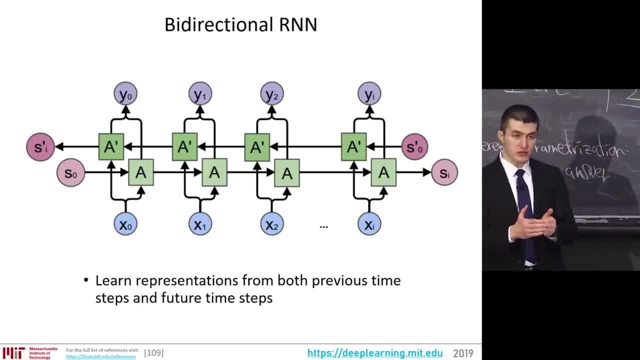 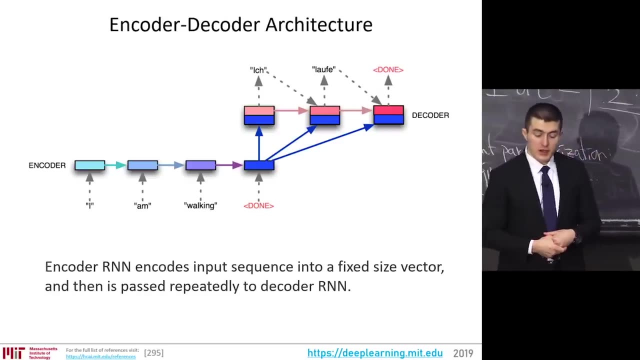 it's not real time operation in that you're able to also look into the future. you look into the data that follows after, the sequence so benefits: you do a forward pass through the network beyond the current and then back the encoder decoder architecture in recurrent neural networks. 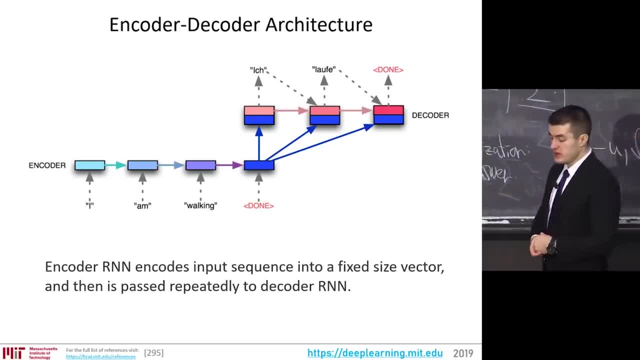 used very much when the sequence on the input and the sequence on the output are not relied to be of the same length. the task is to first, with the encoder network, encode everything, that's came everything on the input sequence. so this is useful for machine translation, for example. 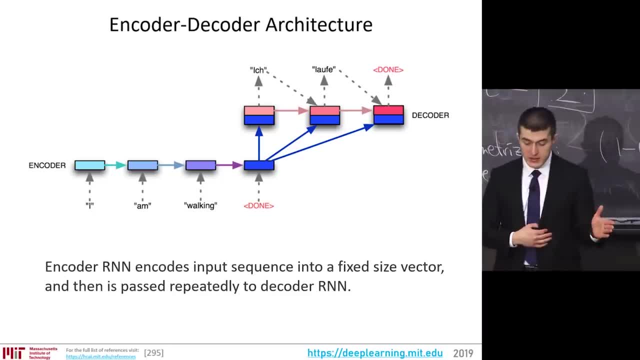 so encoding all the information, the input sequence in English and then in the language you're translating to. given that representation, keep feeding it into the decoder recurrent neural network to generate that translation. the input might be much smaller and much larger than the output. that's the encoder decoder. 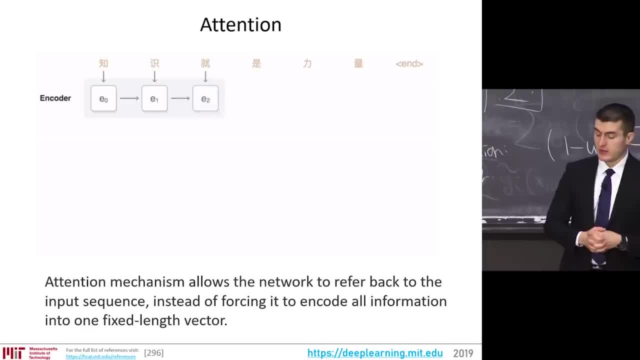 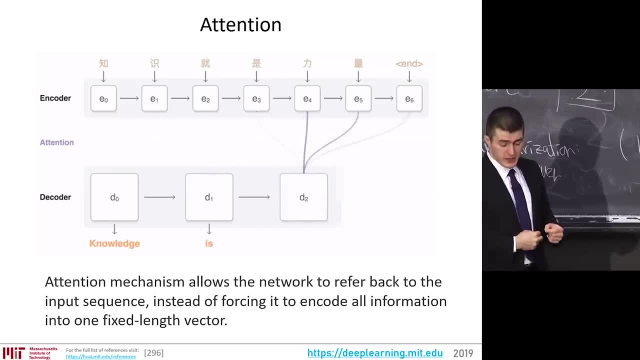 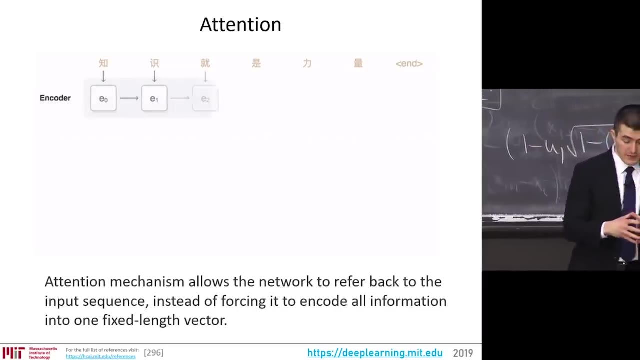 architecture. and then there's improvements. attention is the improvement on this encoder, decoder architecture that allows you to- as opposed to taking the input sequence, forming representation of it and that's it. it allows you to actually look back at different parts of the input, so not just relying on the. 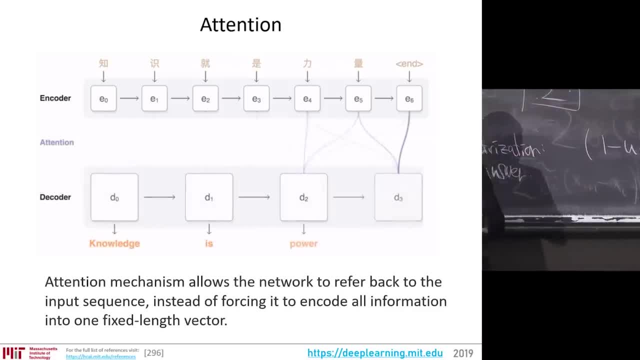 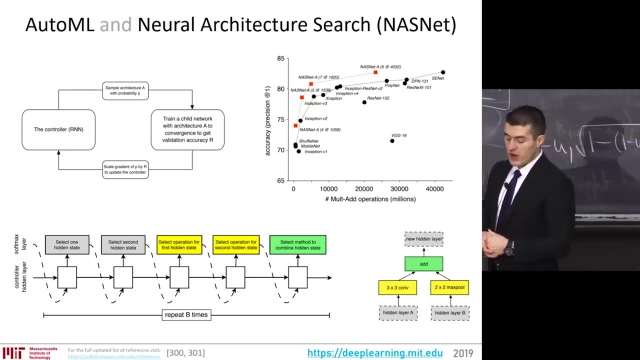 output on the on the single vector representation of all the entire input, and a lot of excitement has been around the idea. as I mentioned, some of the dream of artificial intelligence and machine learning in general has been to remove the human more and more and more from the picture. 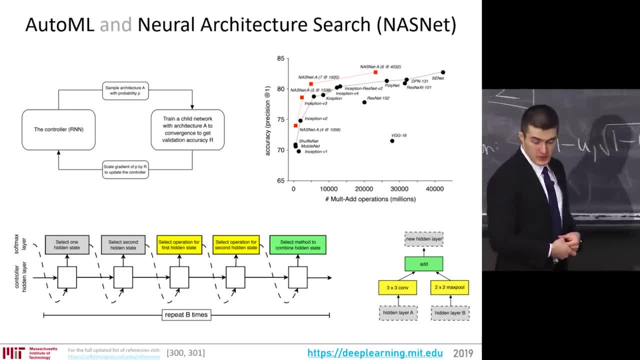 being able to automate some of the difficult tasks. so AutoML from Google and just the general concept of neural architecture search, NASNet, the ability to automate the discovery of parameters of a neural network and the ability to discover the actual architecture that produces the best result. so, with neural architecture search, 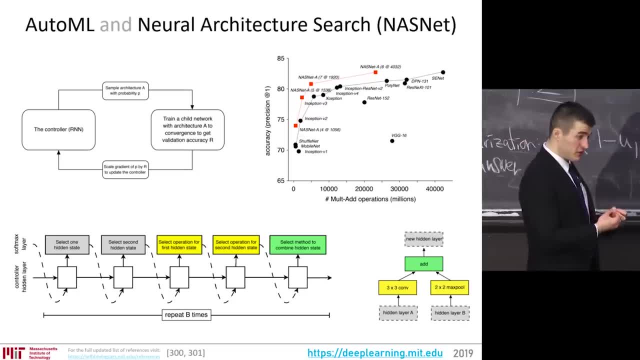 you have basic, basic modules similar to the ResNet modules and with a recurring neural network. you keep assembling a network together and assembling it in such a way that it minimizes the loss of the overall classification performance, and it's shown that you can then construct a neural network. 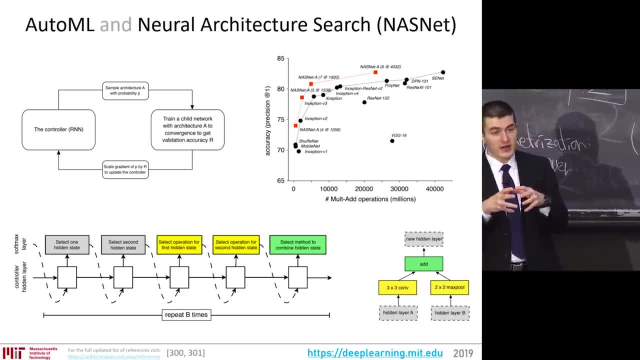 that's much more efficient and much more accurate than state of the art on classification tasks like ImageNet- here shown with a plot- or at the very least competitive with the state of the art and SCNet. it's super exciting that, as opposed to, like I said, stacking Lego pieces yourself, 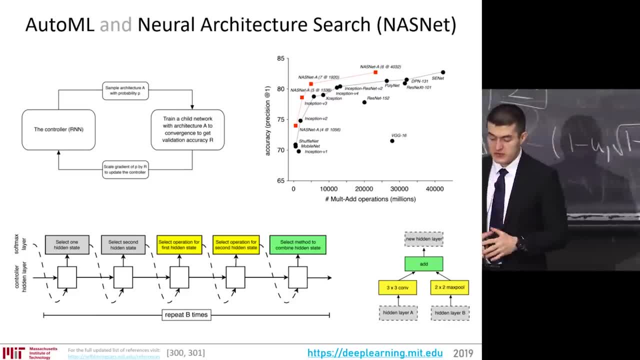 the final result is essentially, you step back and you say: here's, I have a data set with the, with the labels, with the ground truth, which is what Google, the dream of Google AutoML, is. I have the data set. you tell me what kind of neural network. 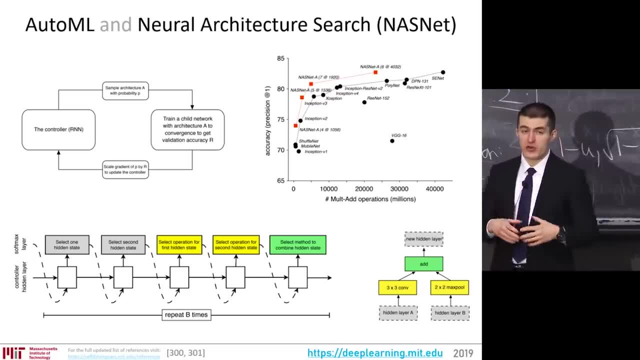 will do best on this data set and that's it. so all you bring is the data. it constructs the network through this neural architecture search and returns to you the model, and that's it it solves. it makes it possible to solve exception, you know, solve many of the real world problems. 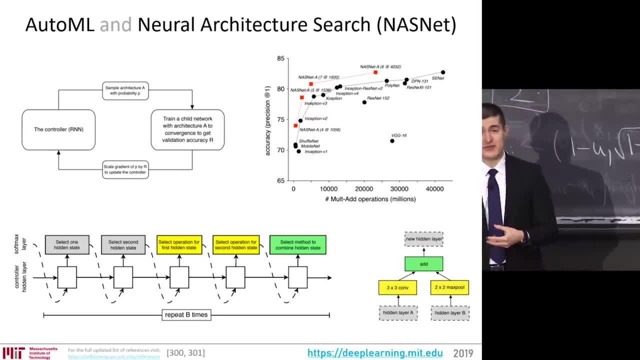 that essentially boil down to. I have a few classes I need to be very accurate on. here's my data set. and then it converts the problem of a deep learning researcher to the problem of maybe what's traditionally what's more commonly called sort of a data science engineer. 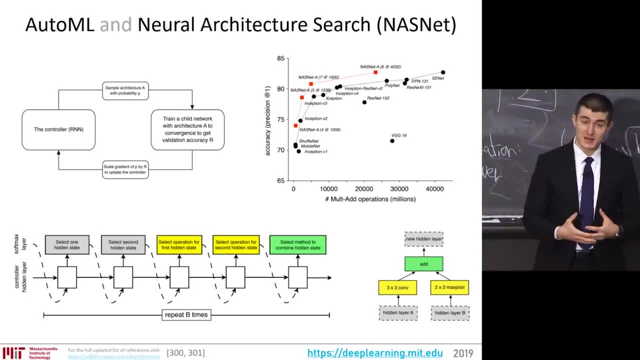 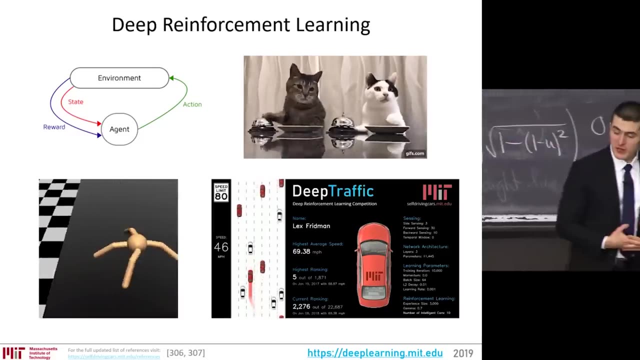 where the task is. as I said, focuses on what is the right question and what is the right data to solve that question, and deep reinforcement learning taking further steps along the path of decreasing human input. deep reinforcement learning is the task of an agent to act in the world. 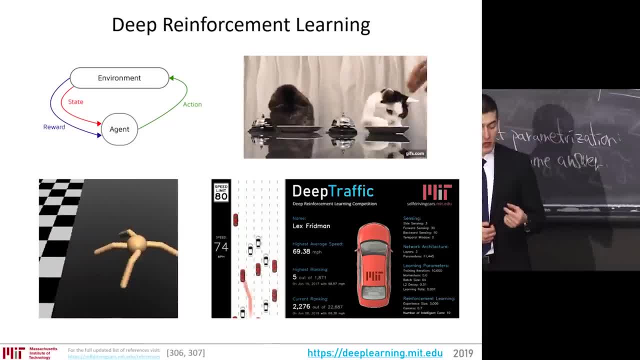 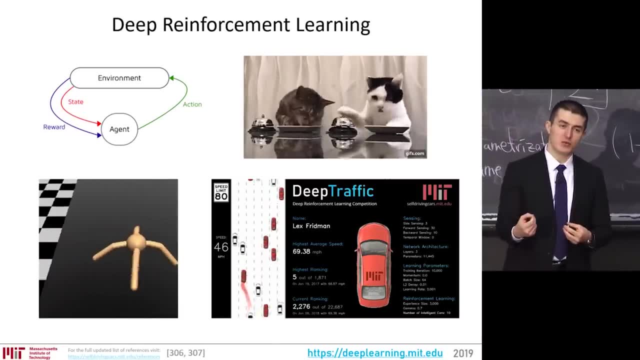 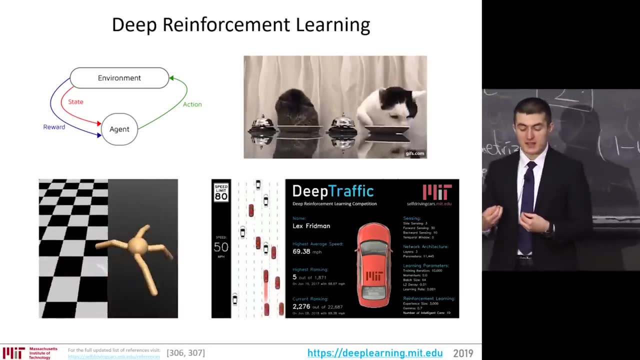 based on the observation of the state and the rewards received in that state, knowing very little about the world and learning from the very sparse nature of the reward, sometimes only when you in the gaming context, when you win or lose, or in the robotics context, when you successfully accomplish a task. 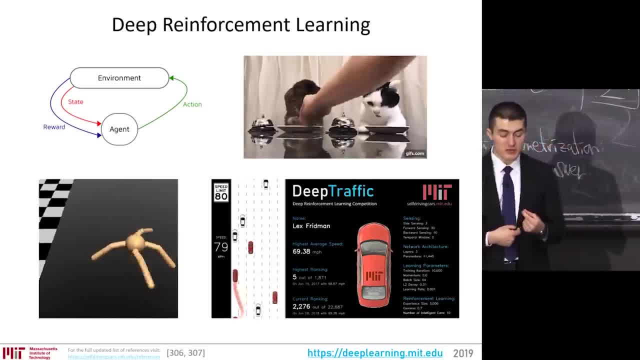 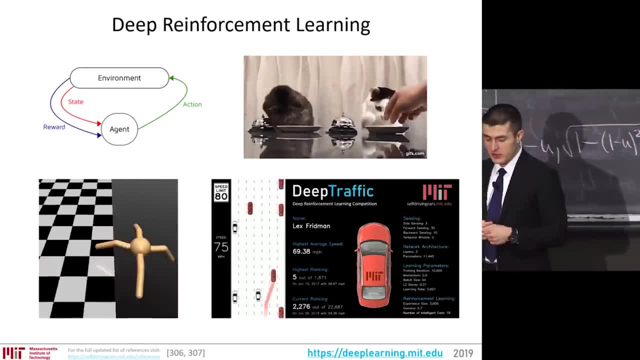 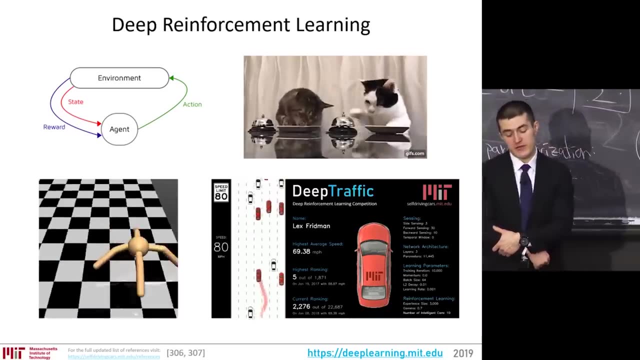 or not. with that very sparse reward, are able to learn how to behave in that world. here with with Katz learning how the bell maps to the food and a lot of the amazing work at OpenAI and DeepMind about the robotics, manipulation and navigation through self play. 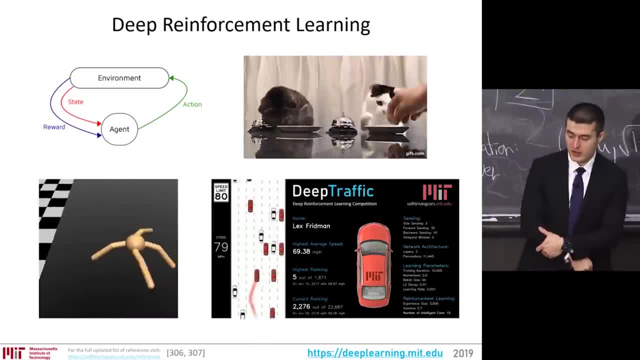 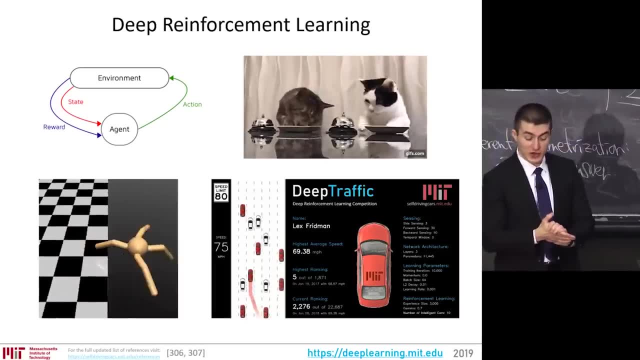 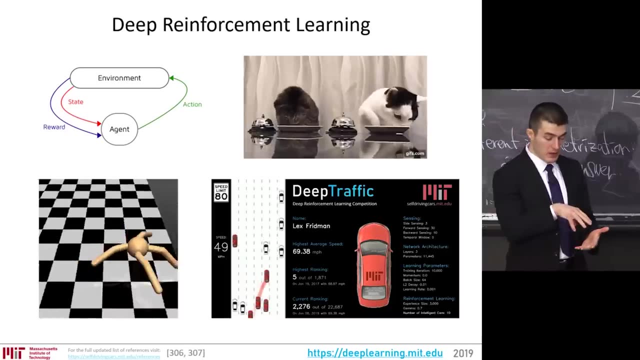 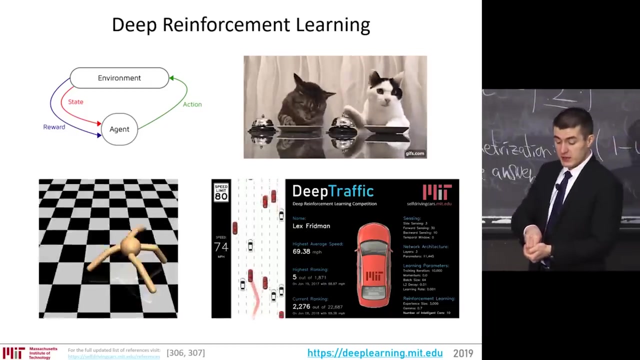 in simulated environments and, of course, the best, our own deep reinforcement, learning competition with deep traffic that all of you can participate and I encourage you to try to win that, with no supervised knowledge, no human supervision, through sparse rewards from the simulation or through self play, constructs able to learn. 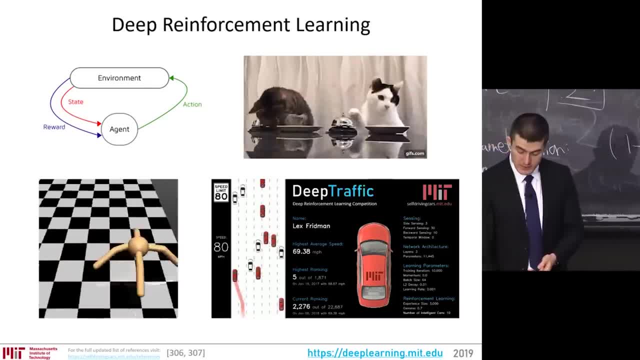 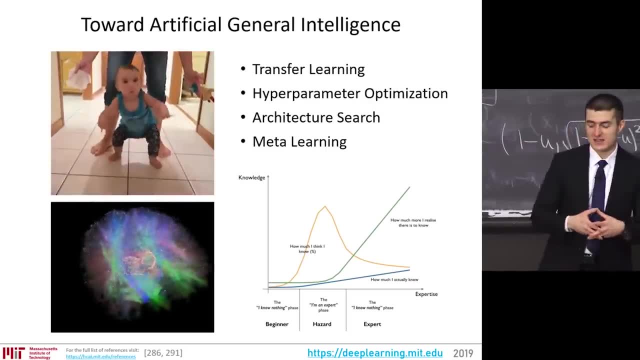 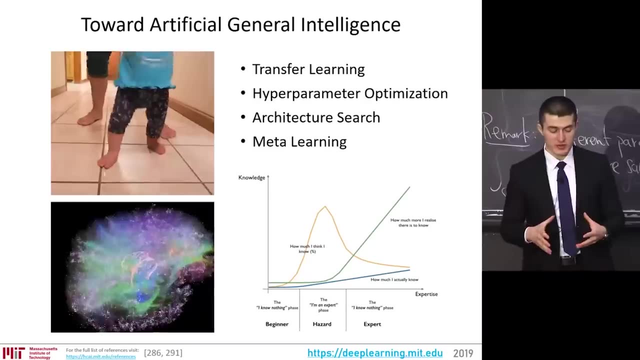 how to operate successfully in this world, and those are the steps we're taking towards general, towards artificial, general intelligence. this is the exciting from from the breakthrough ideas that we'll talk about on Wednesday: natural language processing to generate adversarial networks able to generate arbitrary data. high resolution data. 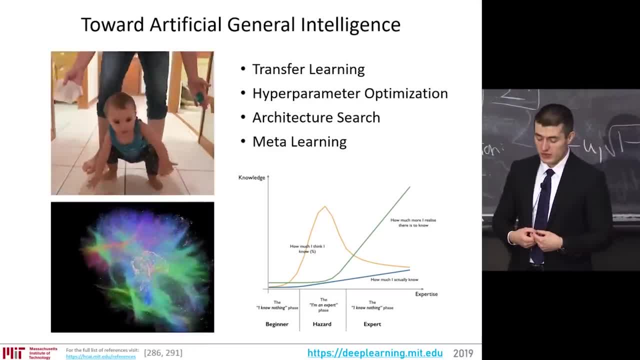 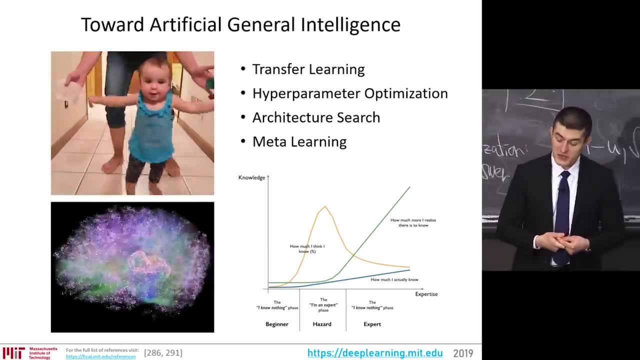 create data really, from this understanding of the world to deep reinforcement, learning, being able to learn how to act in the world- very little input from human supervision. it's taking further and further steps and there's been a lot of exciting ideas going by different names, sometimes misused.